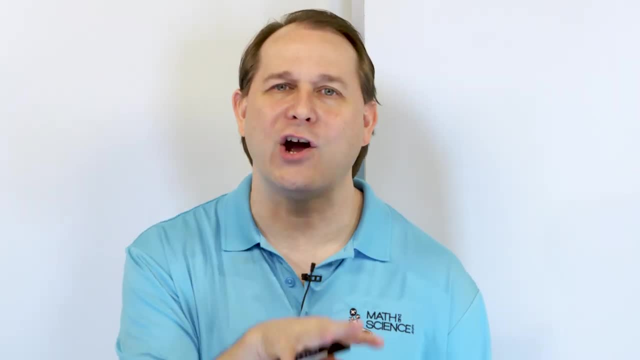 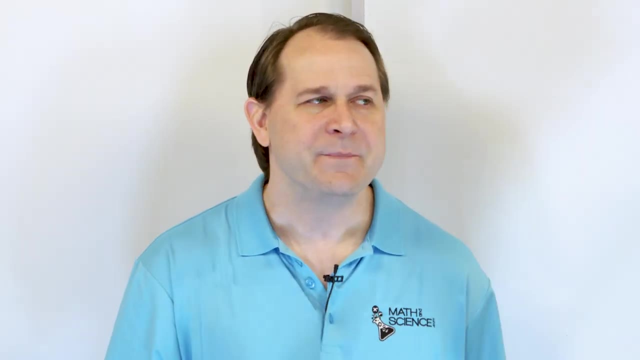 integration. Integration in calculus is based on the concept of a series. So when you learn this material in this lesson right now, learning the concept of a series, it is going to directly feed into what you learn for about two months in calculus one. It is that important okay. 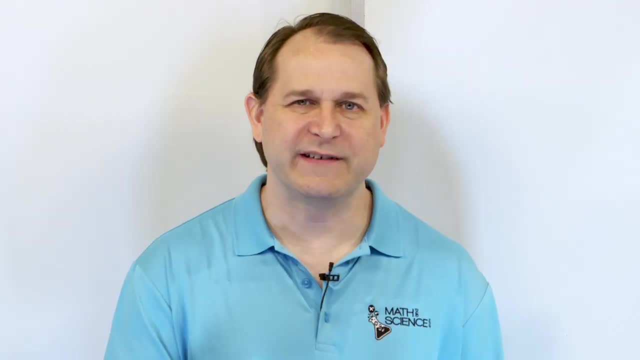 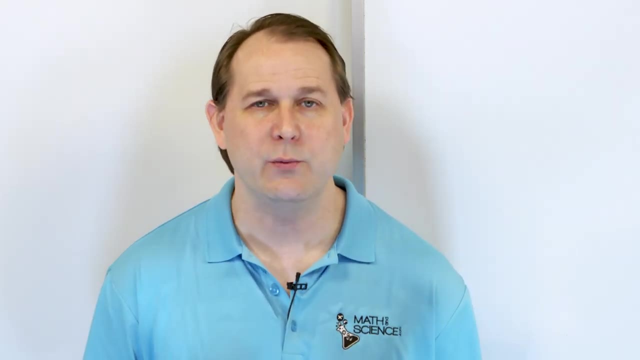 And then, finally, I'll just give you a little more motivation, This concept of a series. it doesn't ever go away, In fact, when you get into more advanced physics, when you talk about, for instance, Einstein's general theory of relativity, which is his theory of gravity. 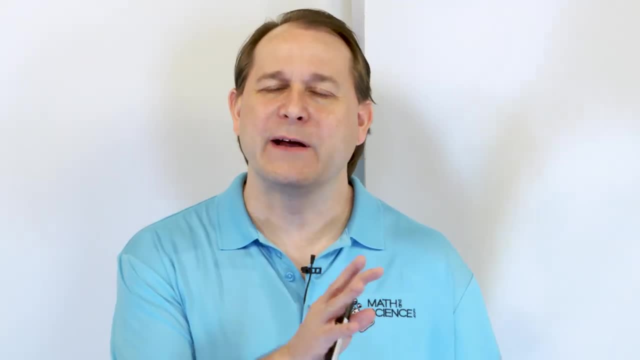 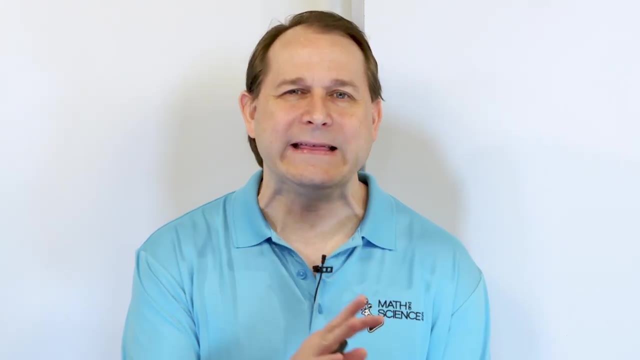 all of the equations have. actually, there's something called the Einstein summation convention, which is very closely related to series. In other words, there's so many things in gravity theory that we have to add together that Einstein invented his own way of writing. 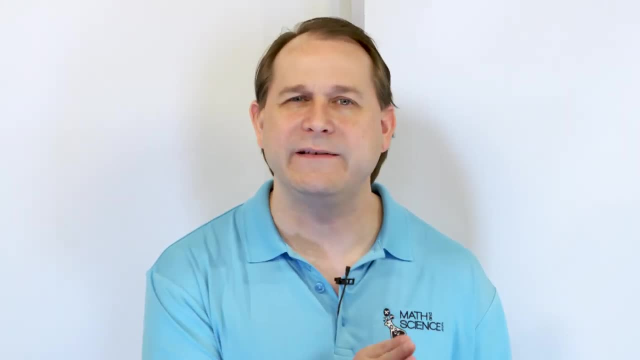 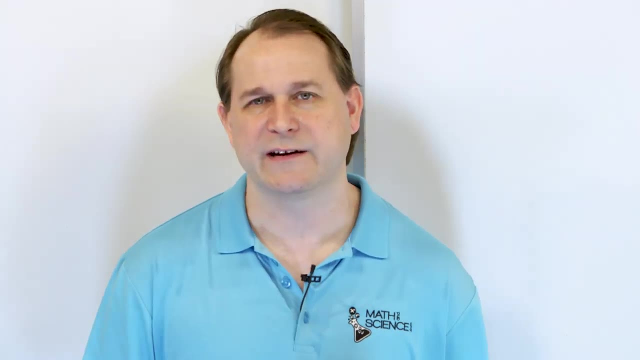 it down. So that's how important it is. The stuff you're learning right now feeds in the calculus, feeds in the very advanced modern physics theories that we use Even in the modern day, So it's something that's going to be around, Okay, so let's go back to the 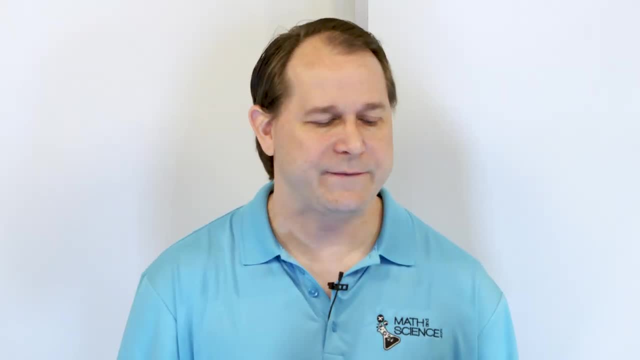 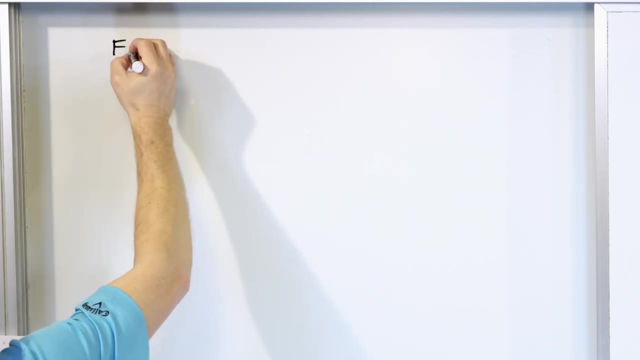 beginning. talk about what a sequence is, talk about what a series is, write down the sigma notation so we can solve problems. So let's go back down memory lane. let's talk about what we've learned before. Finite sequence. Now the reason I'm putting. 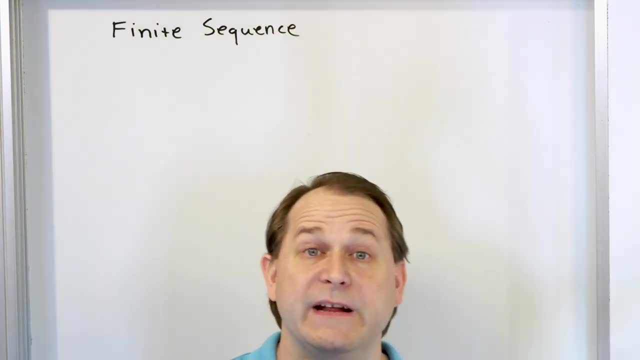 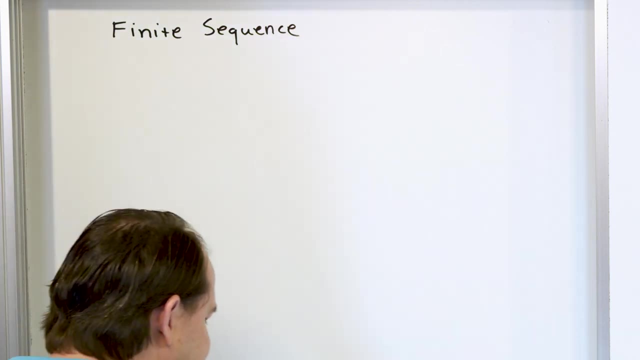 the word finite in the beginning is because we can actually have infinite sequences. You know, when you don't actually have an end point, when you just keep on adding numbers into the sequence, it would be infinite. But here let's just talk about and remember what a finite sequence is. 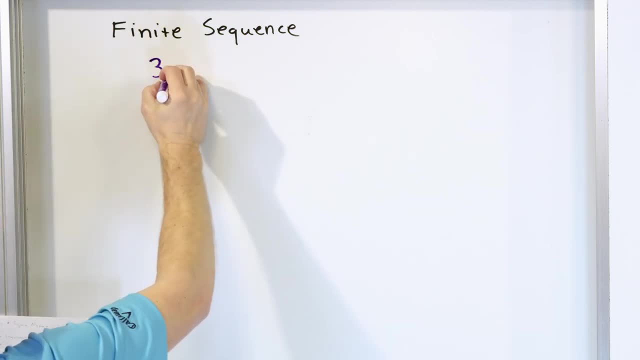 Let's give an example. A finite sequence might be something like 3, 7,, 11,, 15,, 19.. Now this is finite because it has 1, 2, 3, 4, 5 terms, only 5 terms in there. The terms do not. 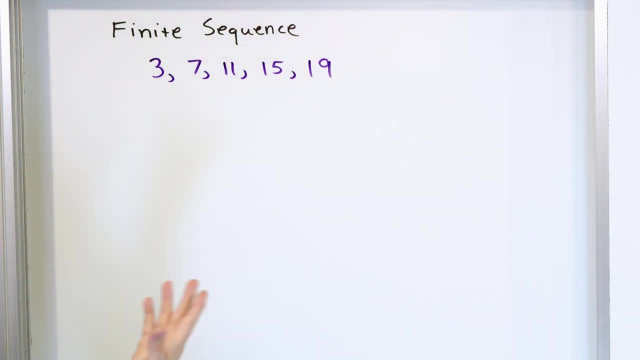 go on forever. There's just a finite listing of them And it's a sequence because there's just commas here. Now, what kind of sequence is this? Because there's lots of different kinds of sequences. This one's one that we've studied before We start here. If we add 4, we get the. 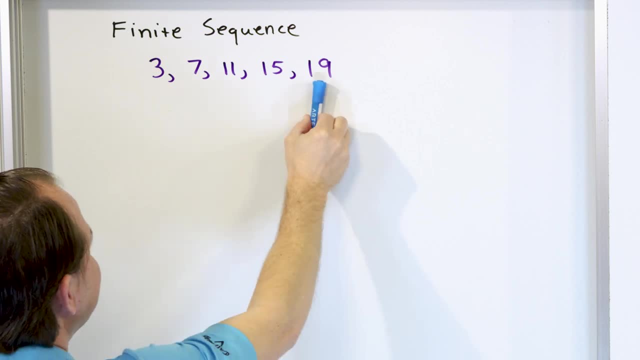 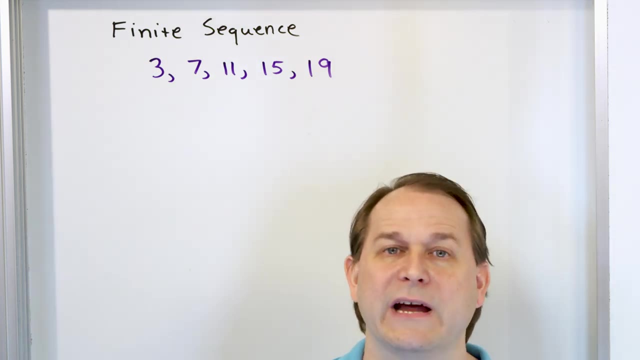 7.. If we add 4,, we get the 11. We add 4, and we add 4.. We can get all of these by just adding a number. So if you remember back to sequences, when we add numbers to get the terms, that's called. 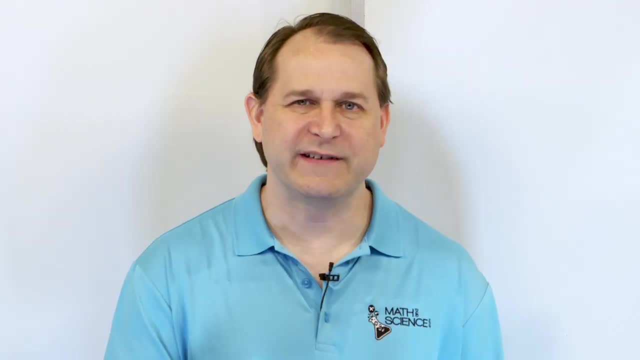 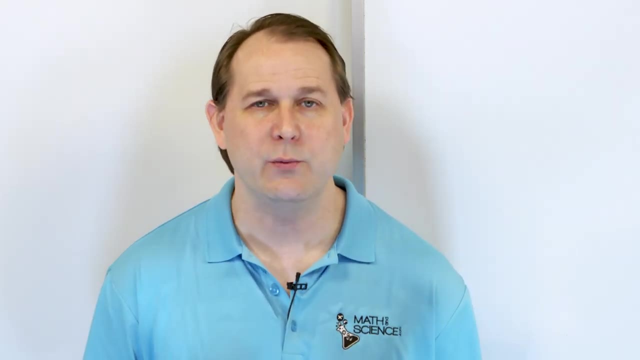 And then, finally, I'll just give you a little more motivation, This concept of a series. it doesn't ever go away, In fact, when you get into more advanced physics, when you talk about, for instance, Einstein's general theory of relativity, which is his theory of gravity. 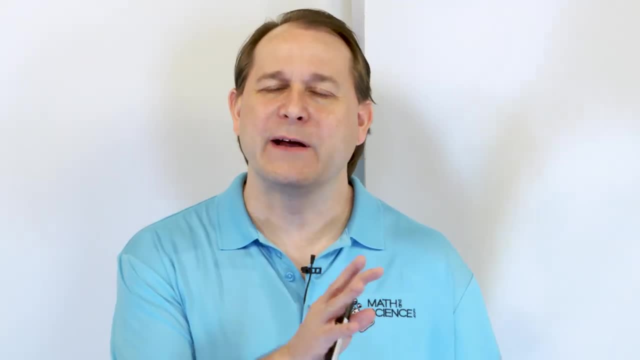 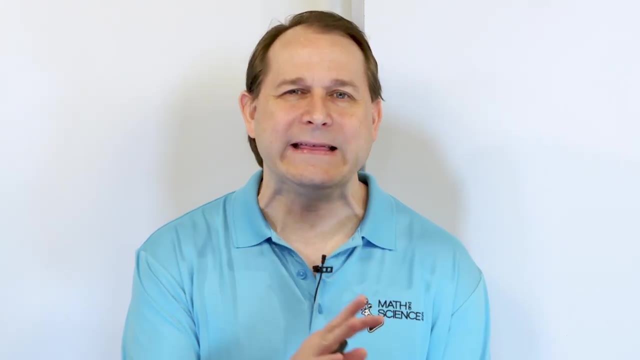 all of the equations have. actually, there's something called the Einstein summation convention, which is very closely related to series. In other words, there's so many things in gravity theory that we have to add together that Einstein invented his own way of writing. 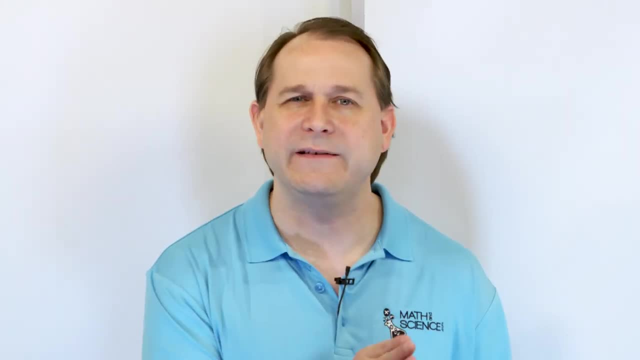 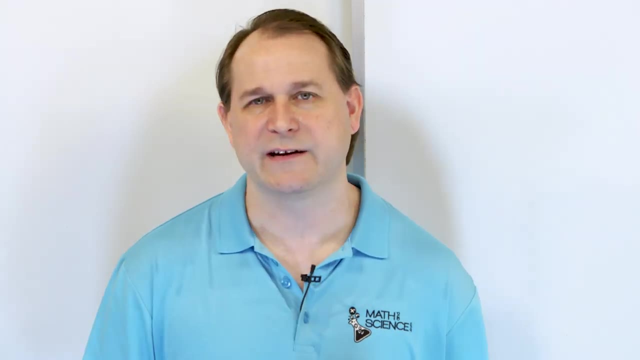 it down. So that's how important it is. The stuff you're learning right now feeds in the calculus, feeds in the very advanced modern physics theories that we use Even in the modern day, So it's something that's going to be around, Okay, so let's go back to the 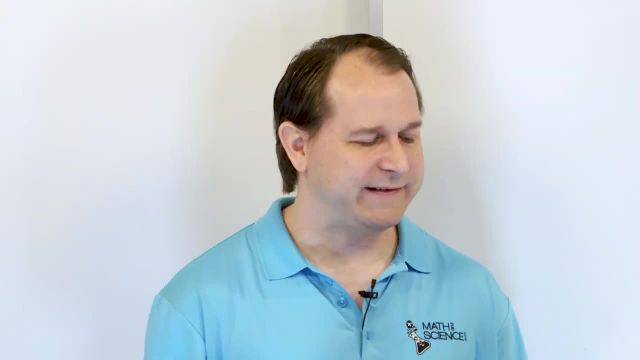 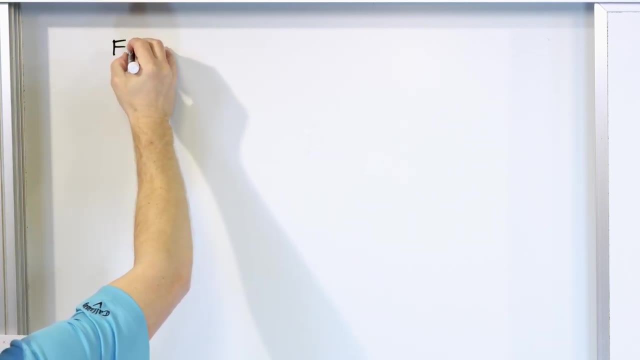 beginning. talk about what a sequence is, talk about what a series is. write down the Sigma notation so we can solve problems. So let's go back down memory lane. Let's talk about what we learned before. finite sequence. Now, the reason I'm putting the word finite in the beginning is 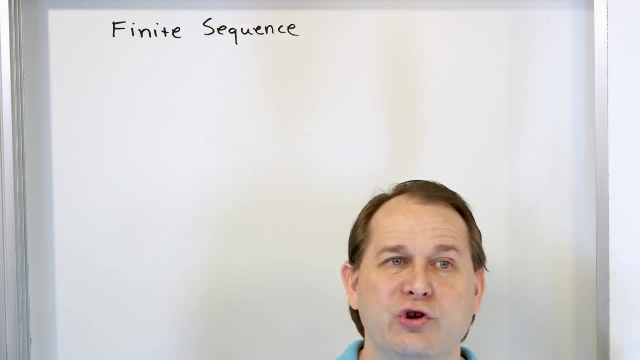 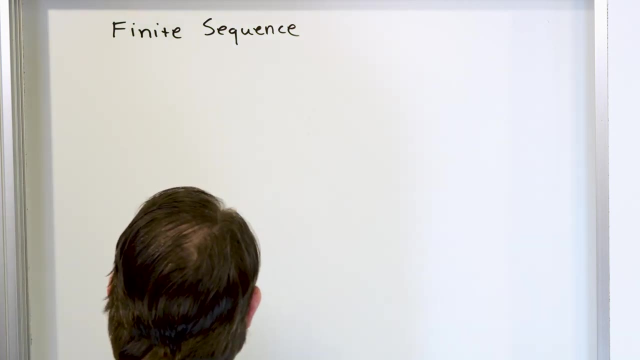 because we can actually have infinite sequences. You know when you, when you don't actually have an end point, when you just keep on adding numbers into the sequence, it would be infinite. But here let's just talk about and remember what a finite sequence is. 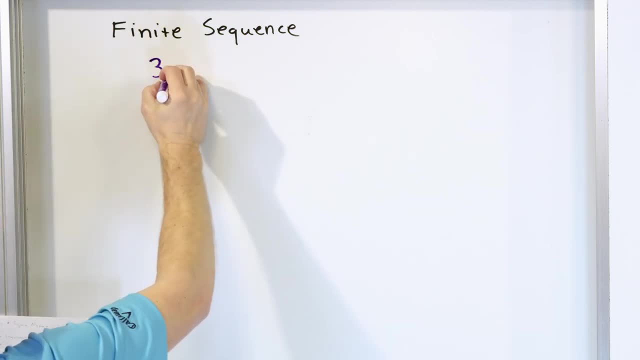 Let's give an example. A finite sequence might be something like 3, 7,, 11,, 15,, 19.. Now this is finite because it has 1, 2, 3, 4, 5 terms, only 5 terms in there. The terms do not. 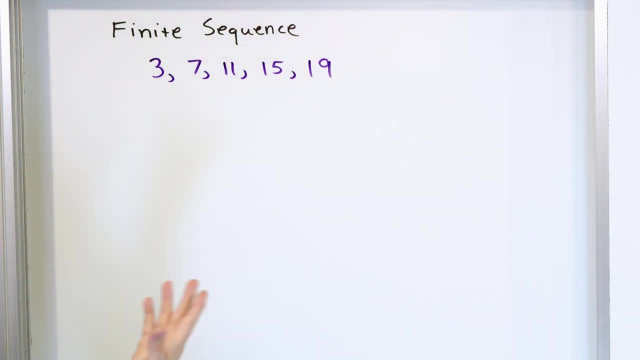 go on forever. There's just a finite listing of them And it's a sequence because there's just commas here. Now, what kind of sequence is this? Because there's lots of different kinds of sequences. This one's one that we've studied before We start here. If we add 4, we get the. 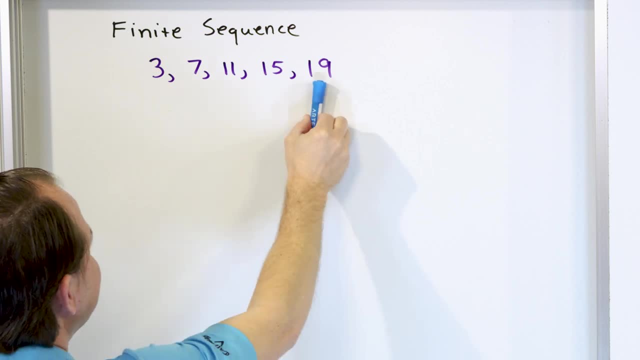 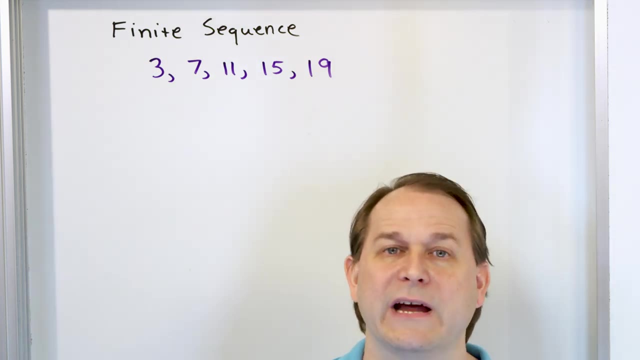 7.. If we add 4,, we get the 11. We add 4, and we add 4.. We can get all of these by just adding a number. So if you remember back to sequences, when we add numbers to get the terms, that's called. 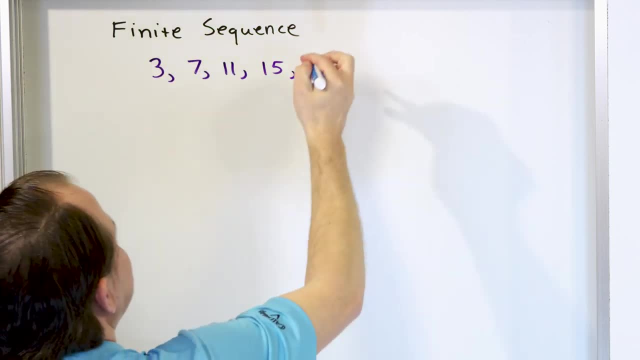 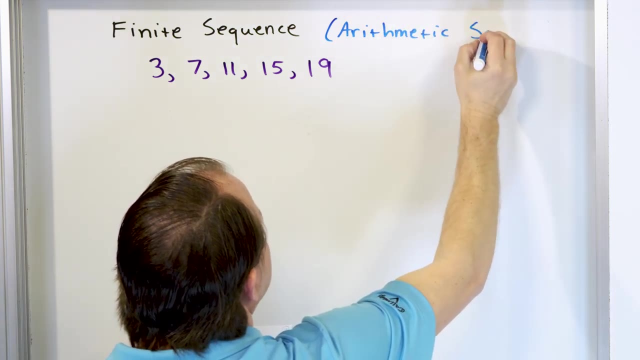 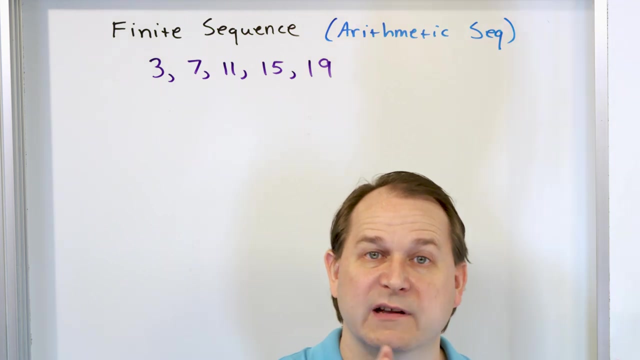 an arithmetic sequence. So up here, under finite sequence, I'm going to remind you that this one is arithmetic And it's an arithmetic sequence: S-E-Q. I'm going to call that arithmetic sequence. Now, the concept of a sequence is just when you have the numbers listed, When we have a series, we actually 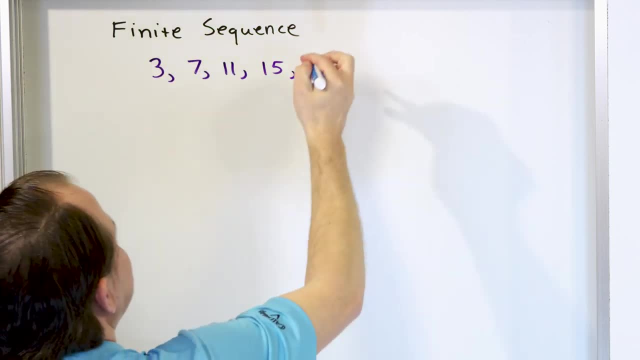 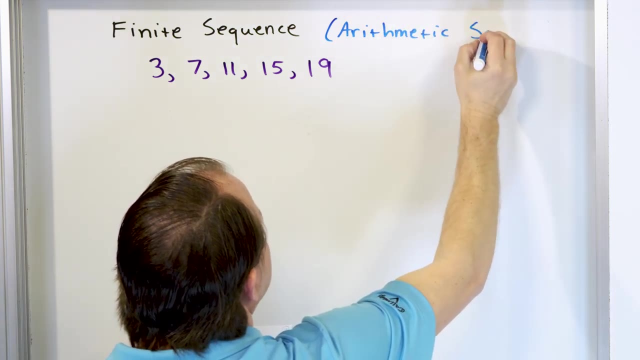 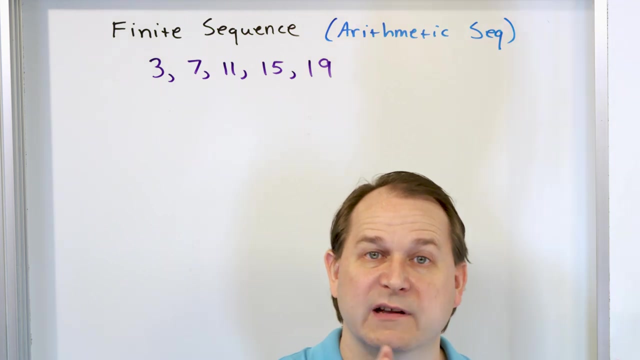 an arithmetic sequence. So up here, under finite sequence, I'm going to remind you that this one is arithmetic And it's an arithmetic sequence: S-E-Q. I'm going to call that arithmetic sequence. Now, the concept of a sequence is just when you have the numbers listed, When we have a series, we actually 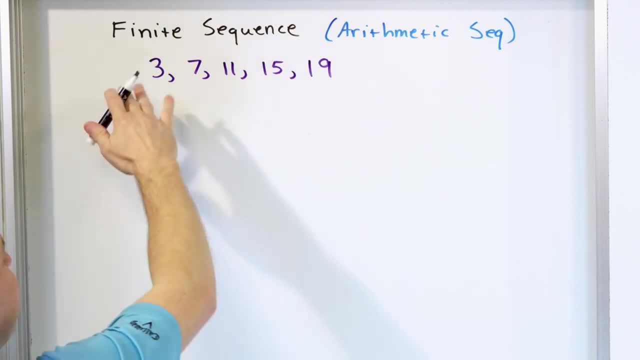 are going to add those numbers together. So, related to this finite sequence, which we now know is an arithmetic sequence, we have an example of a finite series. Now, what do you think this finite series is going to be? I've kind of already given the punchline away. That's fine, It's going to be. 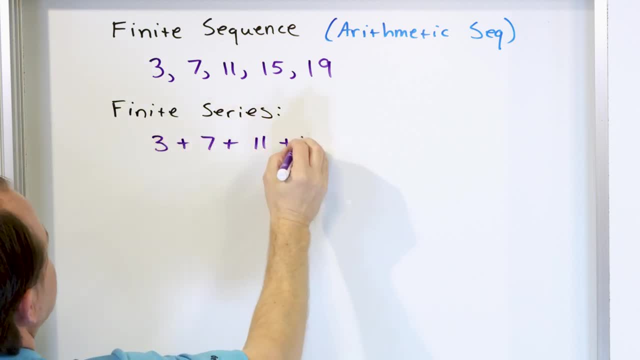 3. Plus 7, plus 11,, plus 15, plus 19.. Now you might look at this and say, well, that's so easy. All you did was put plus signs in between where the commas were. That is the only difference between a. 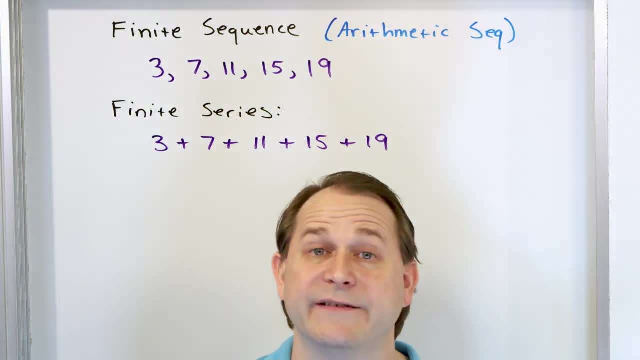 sequence and a series. A sequence is just a listing of numbers and a series is just the addition of those numbers. Try to burn that in your mind. The reason we use series so much in calculus is because most of calculus is trying to figure out how to add lots of things together. So we have to 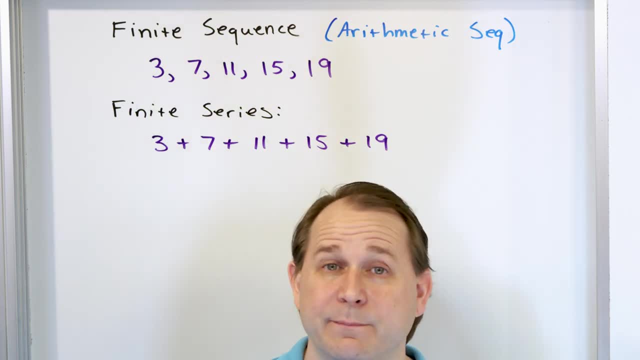 use the concept of a series to do that. I don't want to get into calculus now, But that's basically where you're skating to. That's where you're going to down the road when you learn those advanced things is how to add a bunch of things together. So we have 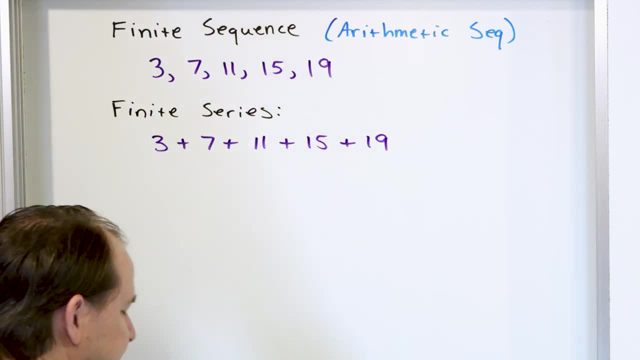 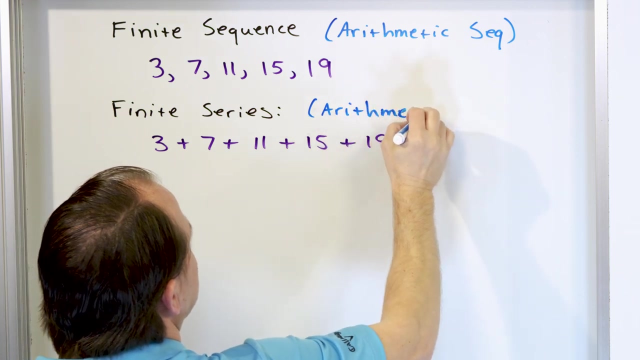 a series to do that Now, because this series is. the terms of the series are listed here, just like the terms of the sequence are here, and the terms of the series are arithmetic in nature. this thing is called an arithmetic series. Arithmetic just means to get the 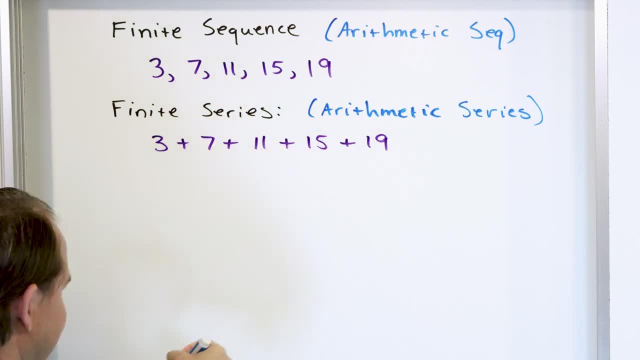 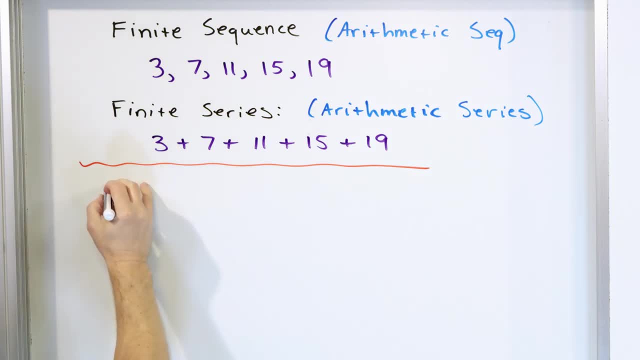 something a little more interesting. Let's talk about an infinite sequence. We haven't really studied infinite sequence too much. I mean, we did do a few examples like that, but I didn't really make a big deal out of it because I knew 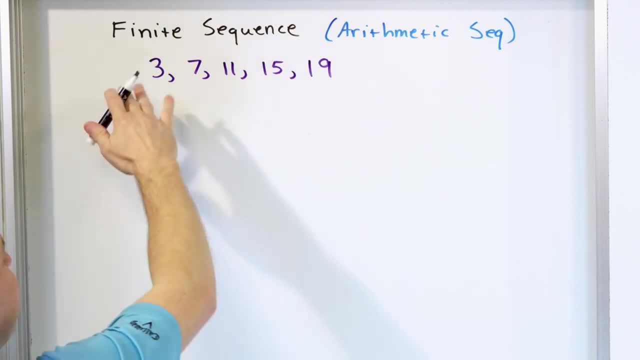 are going to add those numbers together. So, related to this finite sequence, which we now know is an arithmetic sequence, we have an example of a finite series. Now, what do you think this finite series is going to be? I've kind of already given the punchline away. That's fine, It's going to be. 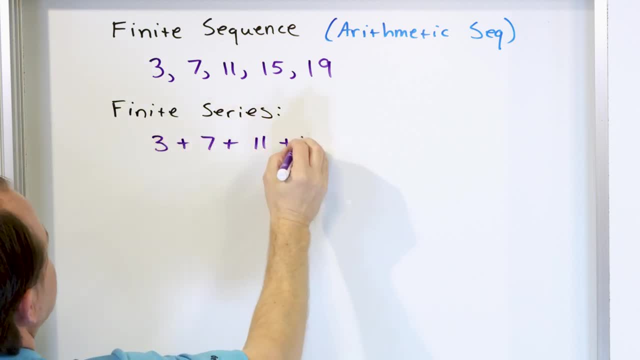 3. Plus 7, plus 11,, plus 15, plus 19.. Now you might look at this and say, well, that's so easy. All you did was put plus signs in between where the commas were. That is the only difference between a. 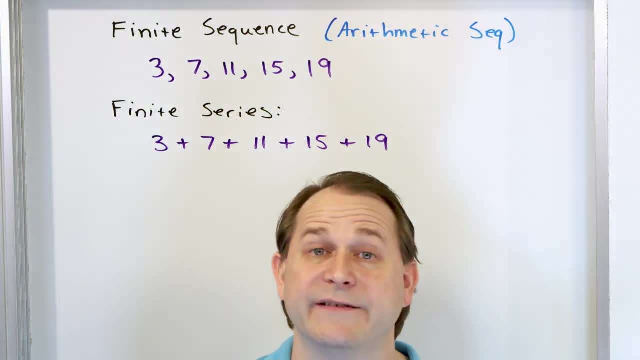 sequence and a series. A sequence is just a listing of numbers and a series is just the addition of those numbers. Try to burn that in your mind. The reason we use series so much in calculus is because most of calculus is trying to figure out how to add lots of things together. So we have to 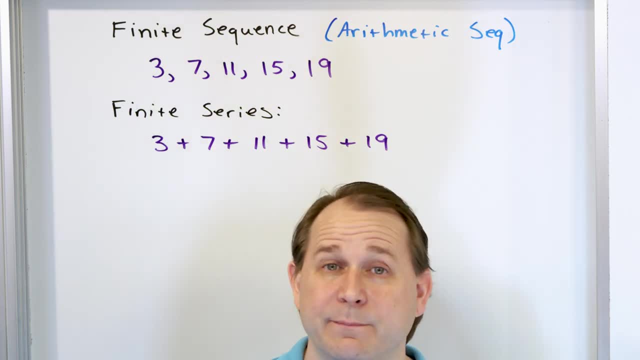 use the concept of a series to do that. I don't want to get into calculus now, But that's basically where you're skating to. That's where you're going to down the road when you learn those advanced things is how to add a bunch of things together. So we have 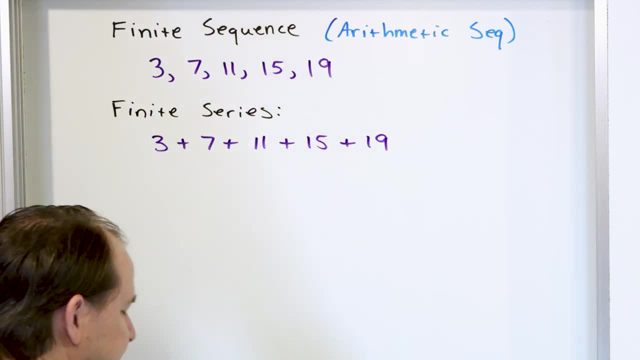 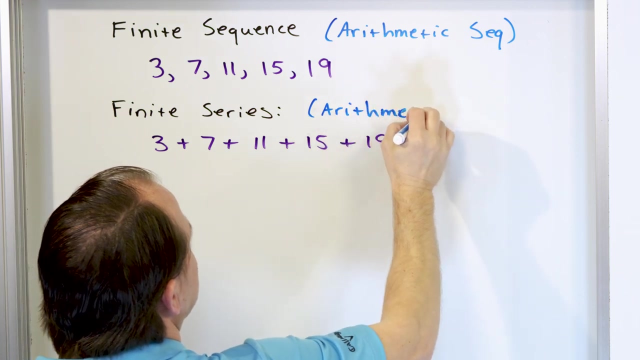 a series to do that Now, because this series is. the terms of the series are listed here, just like the terms of the sequence are here, and the terms of the series are arithmetic in nature. this thing is called an arithmetic series. Arithmetic just means to get the 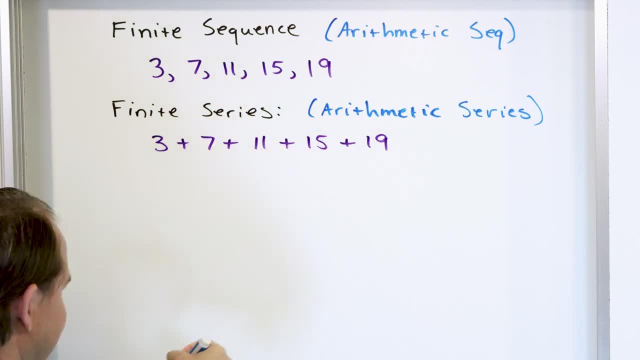 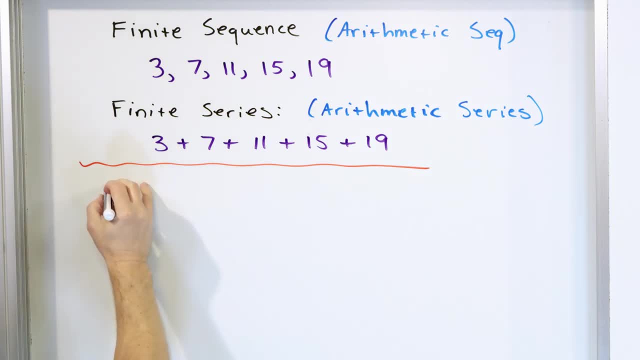 something a little more interesting. Let's talk about an infinite sequence. We haven't really studied infinite sequence too much. I mean, we did do a few examples like that, but I didn't really make a big deal out of it because I knew 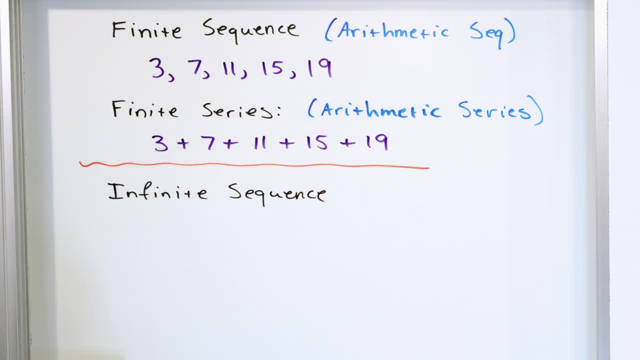 I was going to come to it here. So let's give an example of an infinite sequence. All right, Just an example. What about one half comma, one fourth comma, one eighth comma, one sixteenth comma? dot dot dot? When you see the dot dot dots at the end. 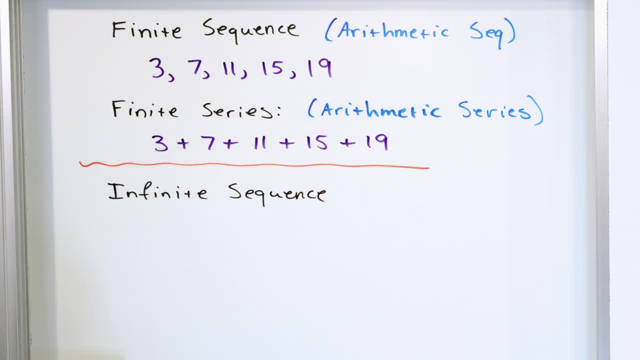 I was going to come to it here. So let's give an example of an infinite sequence. All right, Just an example. What about one half comma, one fourth comma, one eighth comma, one sixteenth comma? dot dot dot? When you see the dot dot dots at the end. 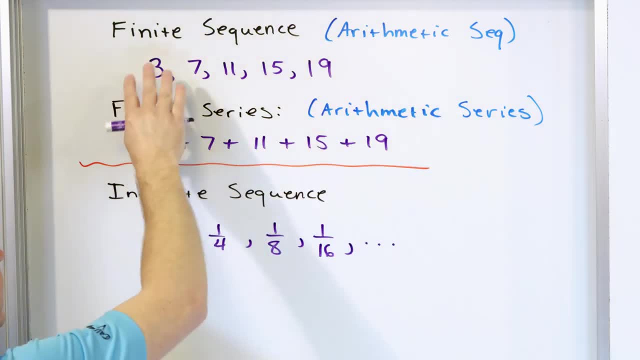 it means the pattern continues and there's no ending to it. These sequences and series ended, but this sequence doesn't end, and that's why it is called an infinite sequence. Now, when you look at the terms of this infinite sequence, you should see a pattern. Notice that. 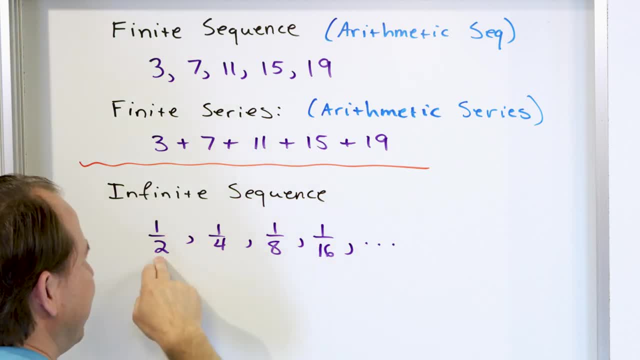 this one to go from this term to this term. we're not adding numbers. We're not just adding a constant number, like we were doing here. This is a little bit more complicated. What we're doing over here is this one: I'm multiplying by a half. If I take this and multiply by a half, 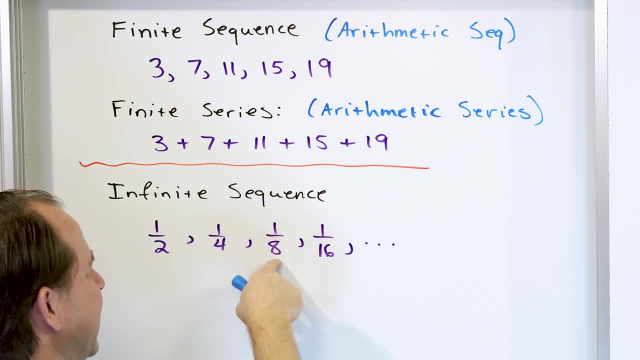 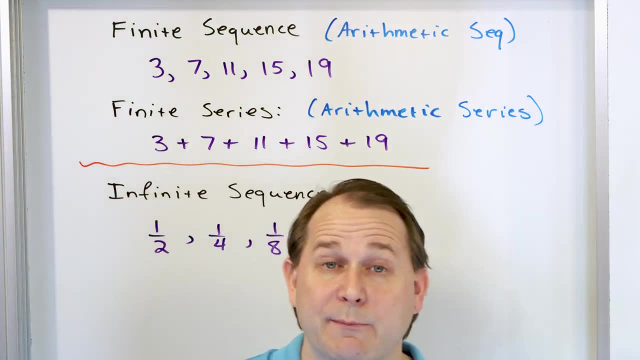 I'm going to get a fourth. If I take this and multiply by one half, I get an eighth. If I take this and multiply by one half, I get one sixteenth. So because I'm multiplying by a common number, a common multiplier, also called a common number, I'm going to get a fourth If I take this and. 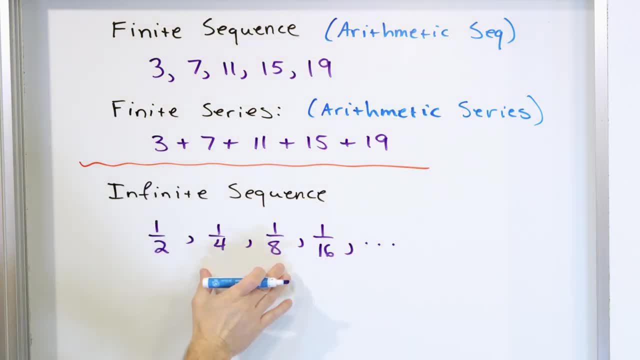 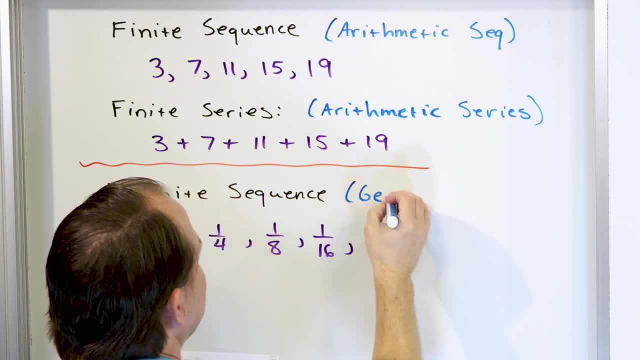 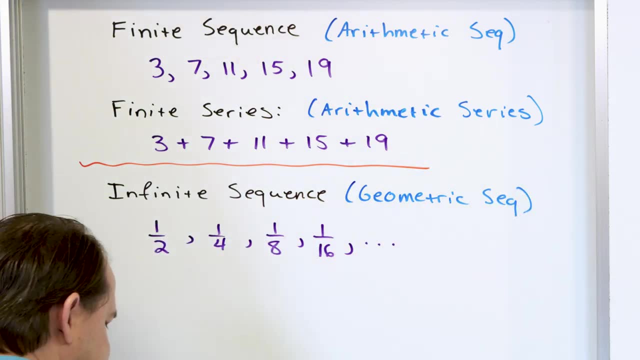 actually called a geometric sequence. So this one is called a geometric sequence. Now what do you think is going to do if we start adding up these terms? Then we're not going to have an infinite sequence, We will have an infinite series. We'll just take the same exact terms, nothing fancy from before. 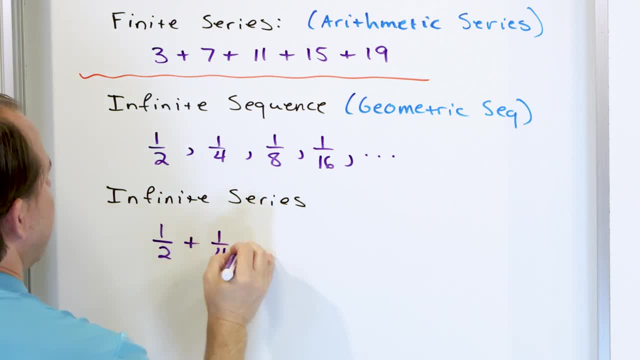 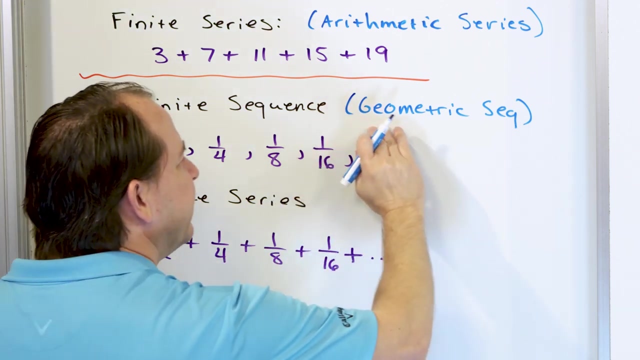 we'll take the one half, add to it one fourth, add to it one eighth, add to it one sixteenth, plus dot, dot dot. We never stop adding. So if this guy was called an infinite sequence of terms, then this thing is called an infinite series, And if this one was called a geometric sequence? 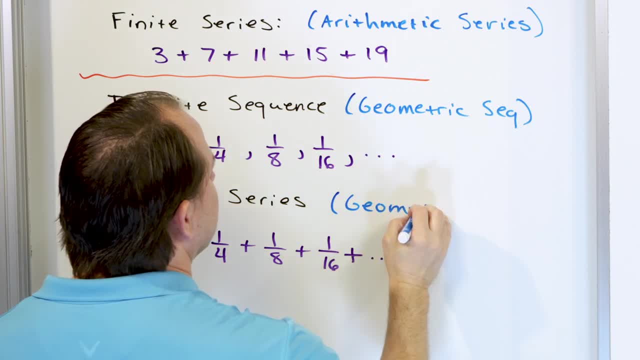 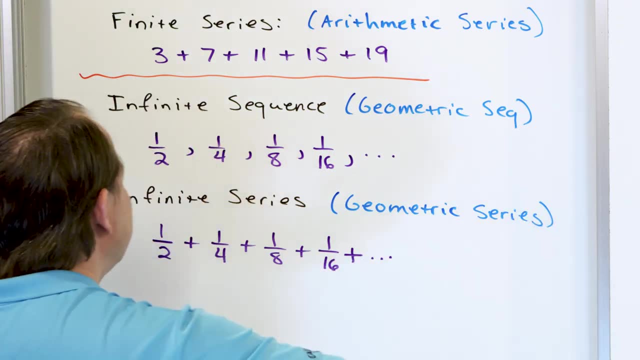 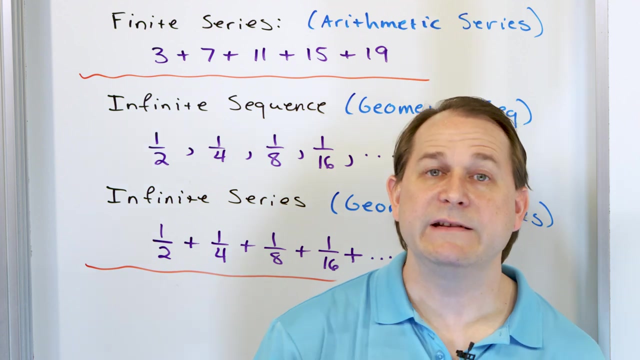 this one is going to be called a geometric series, All right. so anytime you see the word series here, series is here, series is here In your mind, you need to think: well, I'm just adding things up. Anytime you see the word sequence, you need to think: oh, I'm just writing numbers down. 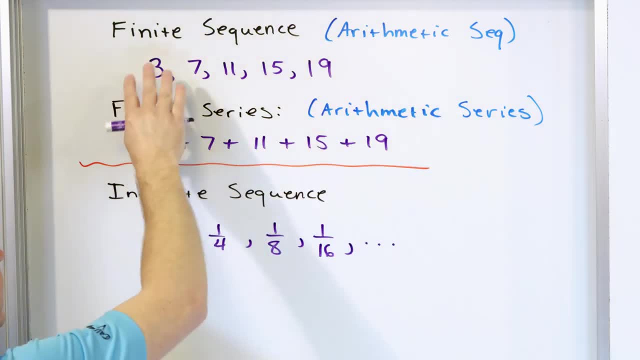 it means the pattern continues and there's no ending to it. These sequences and series ended, but this sequence doesn't end, and that's why it is called an infinite sequence. Now, when you look at the terms of this infinite sequence, you should see a pattern. Notice that. 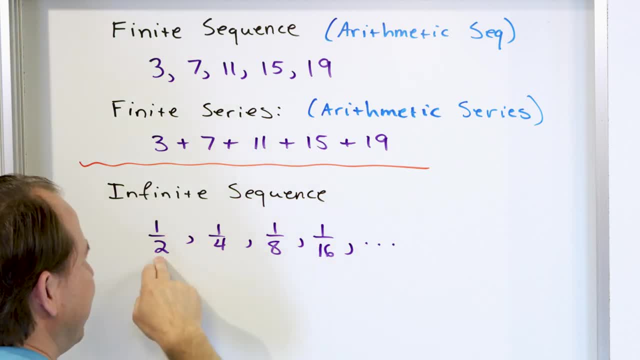 this one to go from this term to this term. we're not adding numbers. We're not just adding a constant number, like we were doing here. This is a little bit more complicated. What we're doing over here is this one: I'm multiplying by a half. If I take this and multiply by a half, 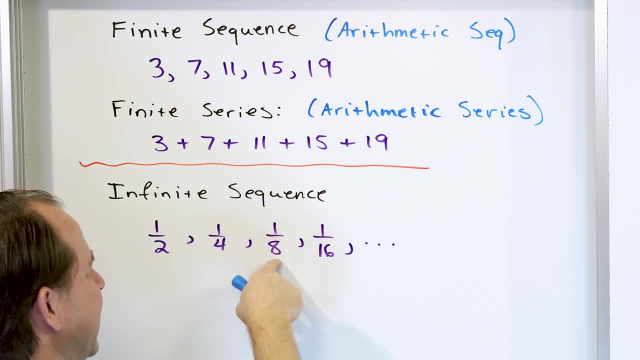 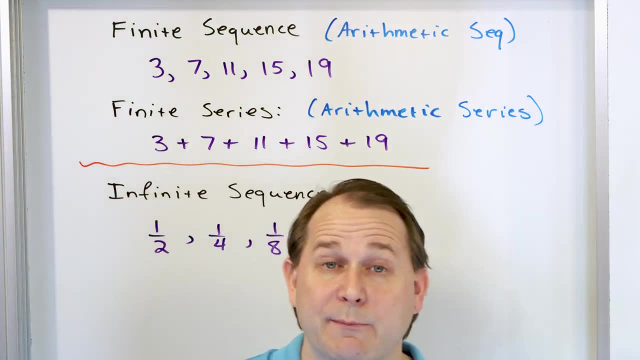 I'm going to get a fourth. If I take this and multiply by one half, I get an eighth. If I take this and multiply by one half, I get one sixteenth. So because I'm multiplying by a common number, a common multiplier, also called a common number, I'm going to get a fourth If I take this and. 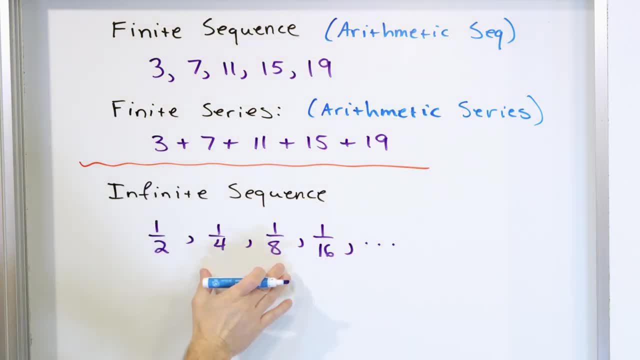 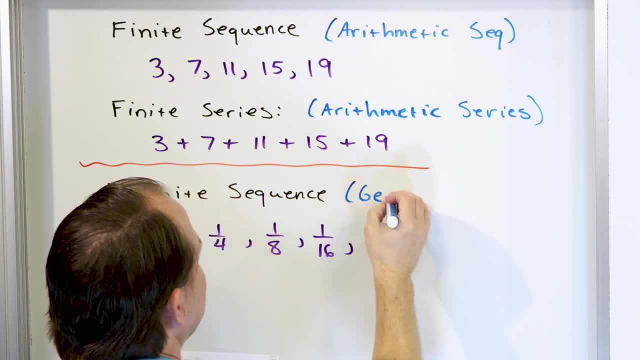 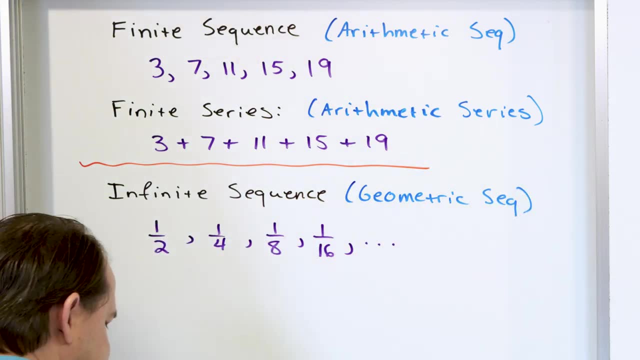 actually called a geometric sequence. So this one is called a geometric sequence. Now what do you think is going to do if we start adding up these terms? Then we're not going to have an infinite sequence, We will have an infinite series. We'll just take the same exact terms, nothing fancy from before. 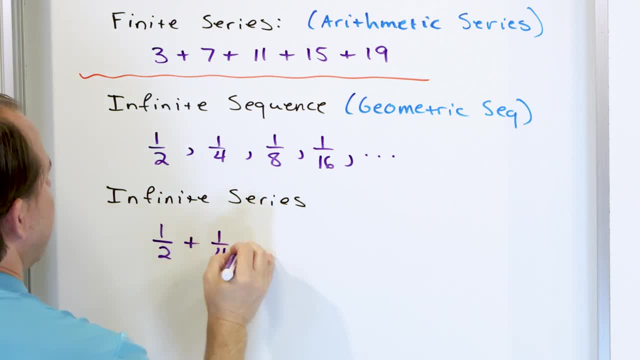 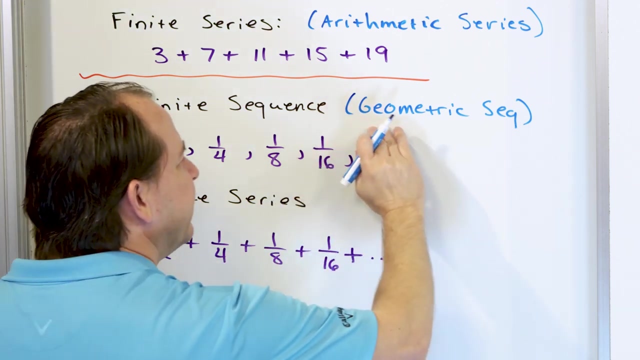 we'll take the one half, add to it one fourth, add to it one eighth, add to it one sixteenth, plus dot, dot dot. We never stop adding. So if this guy was called an infinite sequence of terms, then this thing is called an infinite series, And if this one was called a geometric sequence? 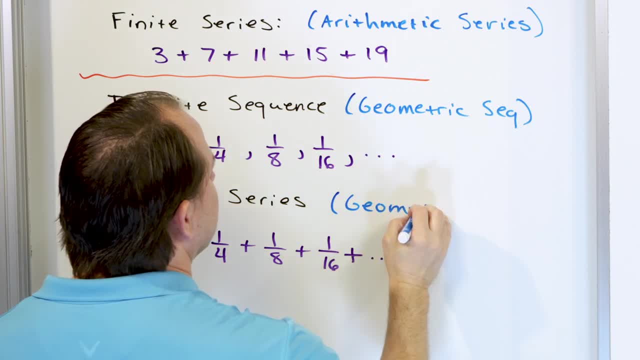 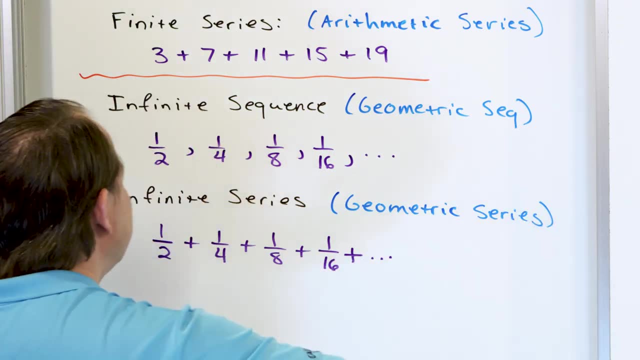 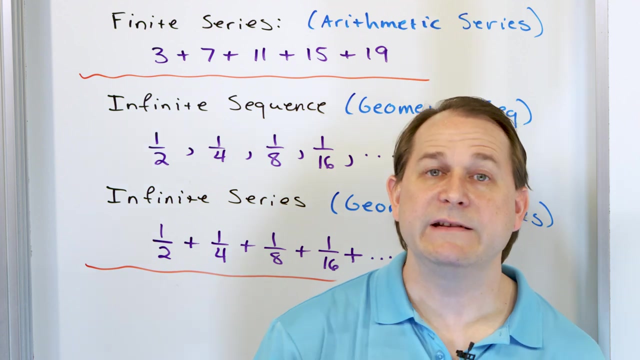 this one is going to be called a geometric series, All right. so anytime you see the word series here, series is here, Series is here In your mind, you need to think: well, I'm just adding things up. Anytime you see the word sequence, you need to think: oh, I'm just writing numbers down. 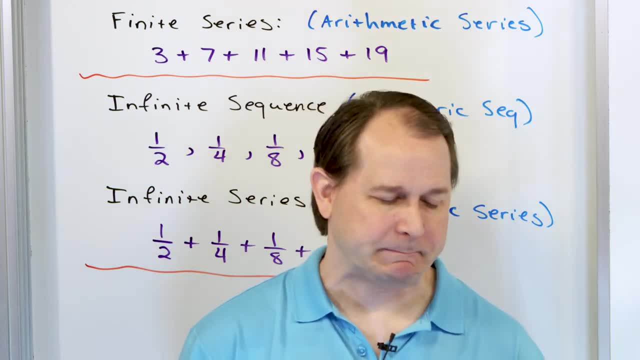 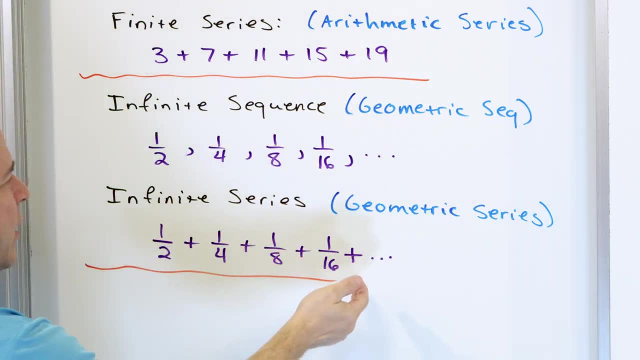 Sequences are important, Series are actually even more important. Okay, now I know what you might be thinking: how can you have an infinite series like this where I'm adding and adding, and adding and adding? like, what am I going to do here? Like, okay, the next term after. 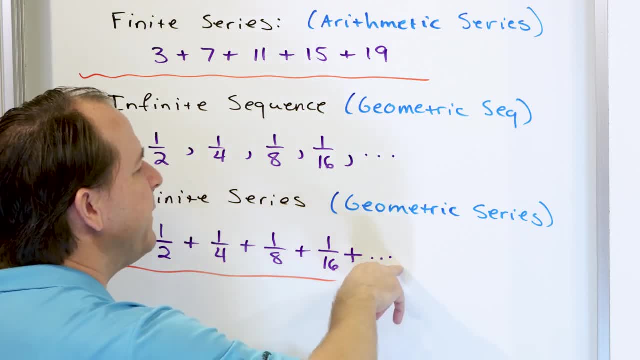 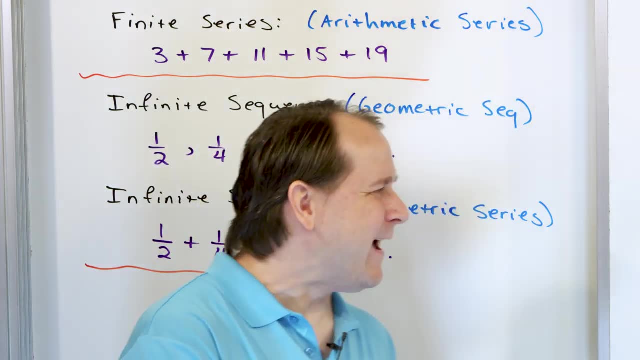 this: if I multiply by a half would be 1 over 32, and then it'd be 1 over 64, and then it'd be 1 over 128.. and I'll just keep on going, and I have more and more and more terms. how can I ever add them? 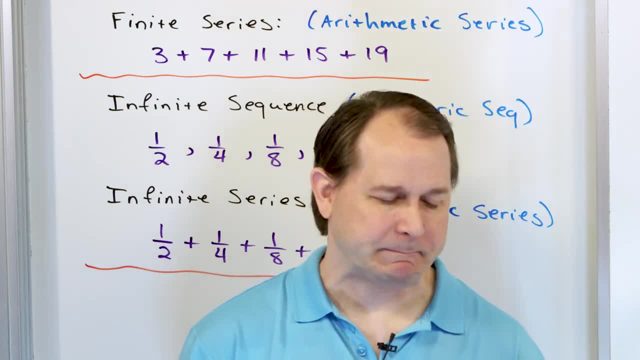 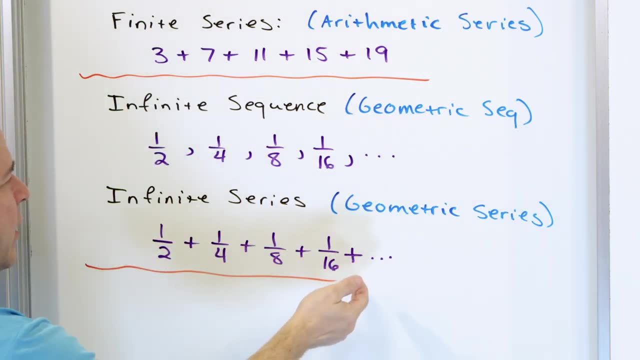 Sequences are important. Series are actually even more important. Okay, now I know what you might be thinking: How can you have an infinite series like this where I'm adding and adding, and adding, and adding, Like, what am I going to do here? Like, okay, the next term after this if I multiply. 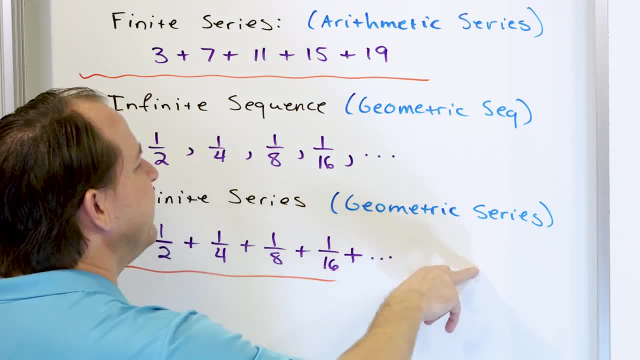 by a half would be one over 32.. And then it'll be one over 64.. And then it'll be one over 128.. and I'll just keep on going, and I have more and more and more terms. how can I ever add them? 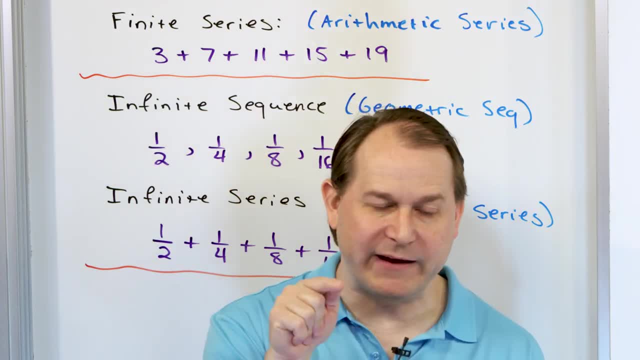 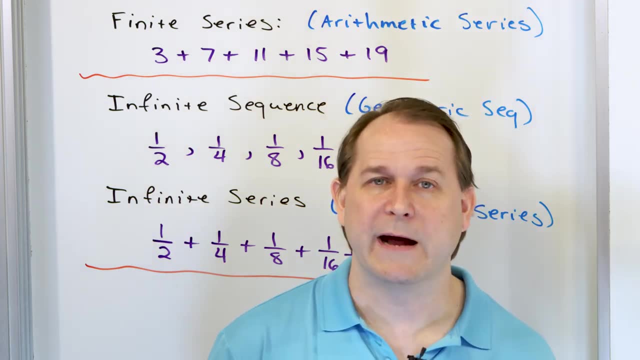 together. I could get my calculator and I can keep pressing the add button and adding the next term, and the next term and the next term. I could go until the sun explodes billions of years from now, until the galaxy disintegrates, I'm still adding numbers. So what is the point of adding up all of? 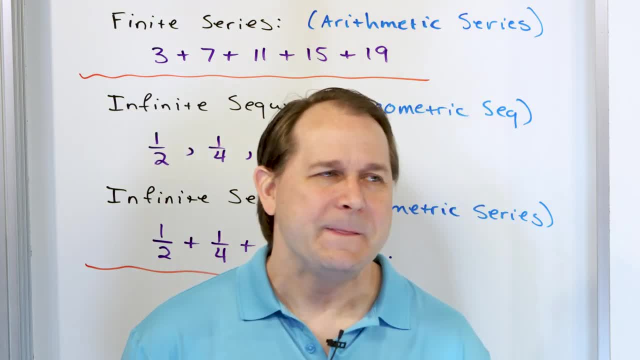 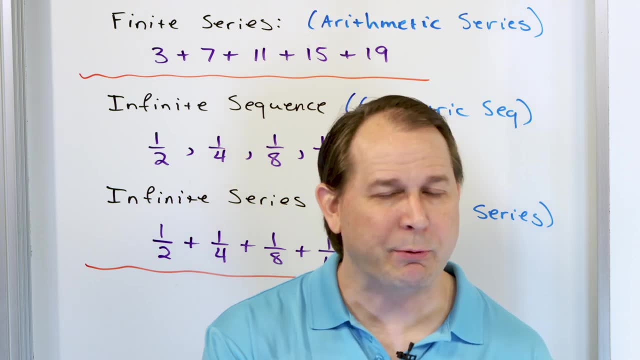 these numbers if I never stop adding? How can I possibly do that? We're kind of getting a little bit touching into the boundaries of calculus. I don't want to get into it right now, but I want to tell you- and this part should blow your mind- that sometimes, even if you add up an infinite 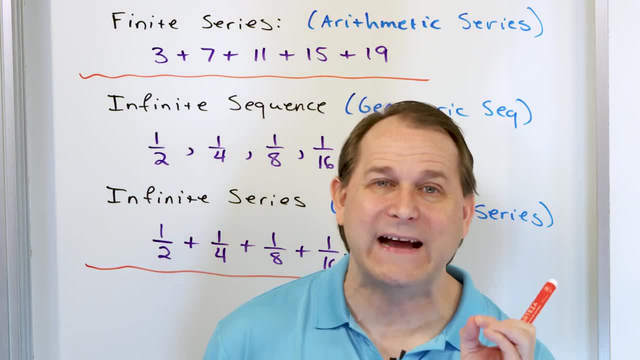 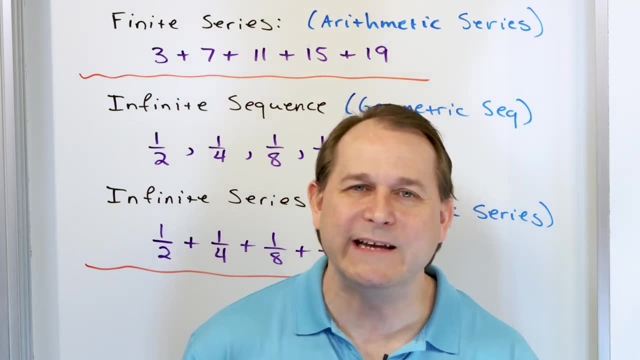 number of things. you can actually still get a finite number as an answer. Now, I'm going to say that one more time because if it goes in one ear and out the other, you're not going to appreciate it. It's really important. What I'm saying is I'm adding up an infinite number of terms, but notice. 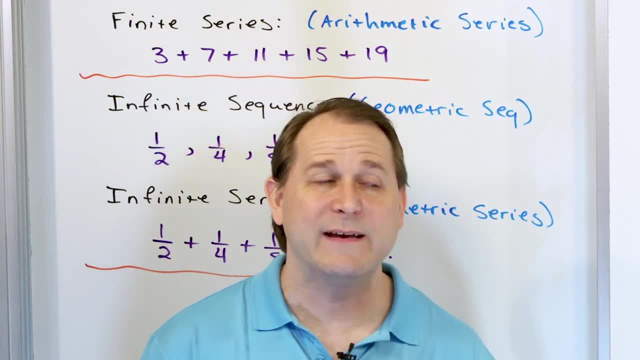 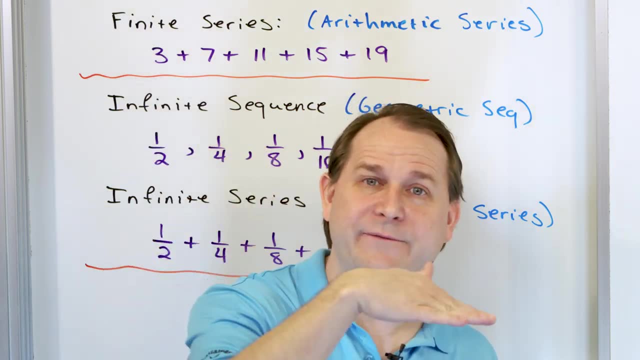 that each term is getting smaller and smaller and smaller. So sometimes- and we will discuss later down the road how you know when you can do this, but sometimes you can't. Sometimes if the terms are decreasing fast enough, even though there's an infinite number of them. 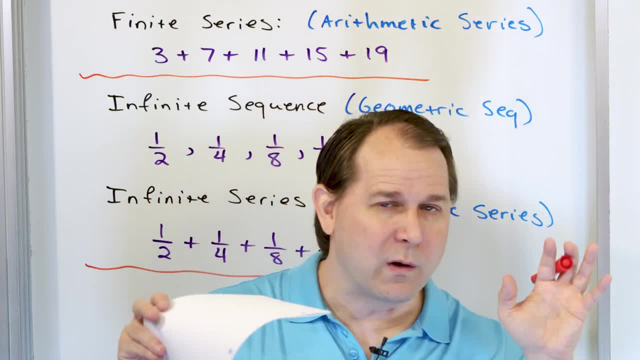 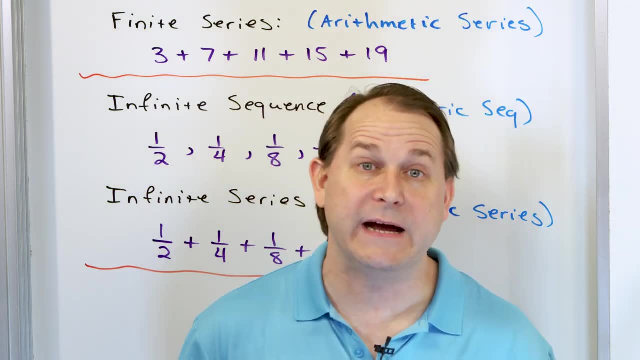 infinite, on and on and on, forever. I can still add them up, quote, unquote and get a finite number, an actual number In other words. most people think if you keep adding and adding and adding, it just goes to infinity. But if the terms are dropping really rapidly, I'll explain later how- 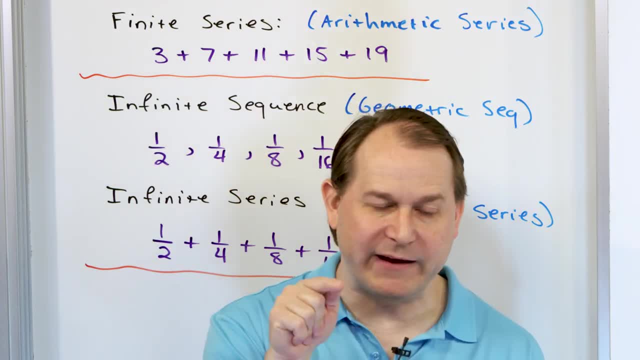 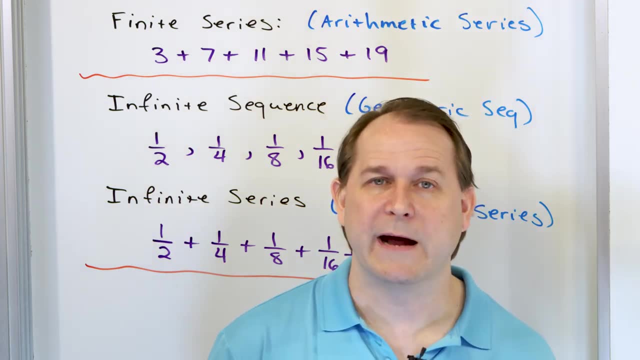 together. I could get my calculator and I can keep pressing the add button and adding the next term, and the next term and the next term. I could go until the sun explodes billions of years from now, until the galaxy disintegrates, I'm still adding numbers. So what is the point of adding up all of? 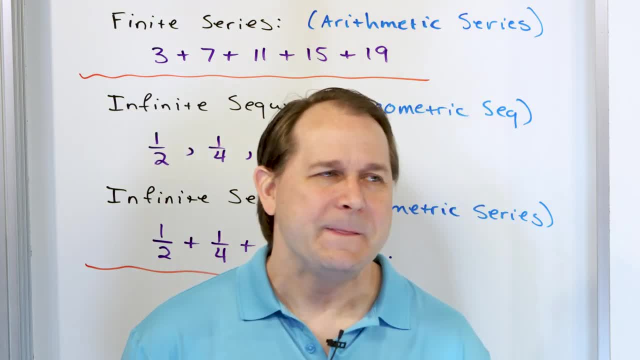 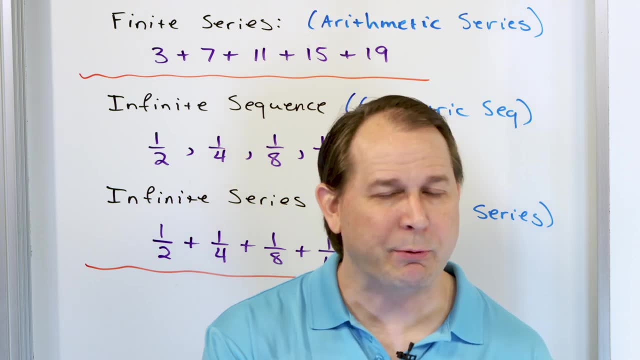 these numbers if I never stop adding? How can I possibly do that? We're kind of getting a little bit touching into the boundaries of calculus. I don't want to get into it right now, but I want to tell you- and this part should blow your mind- that sometimes, even if you add up an infinite 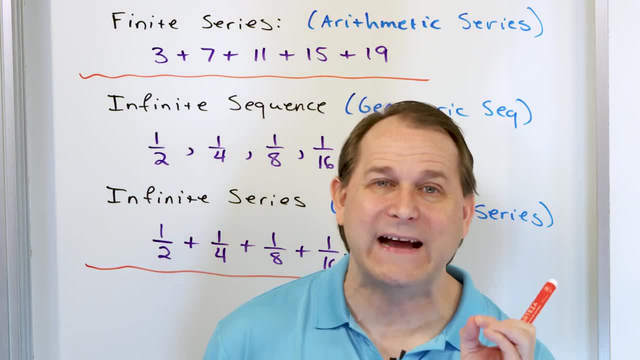 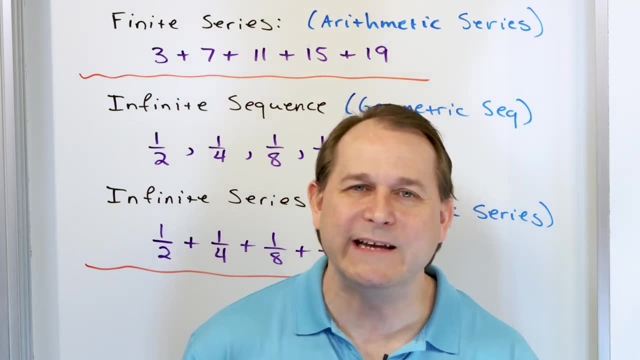 number of things. you can actually still get a finite number as an answer. Now, I'm going to say that one more time because if it goes in one ear and out the other, you're not going to appreciate it. It's really important. What I'm saying is I'm adding up an infinite number of terms, but notice. 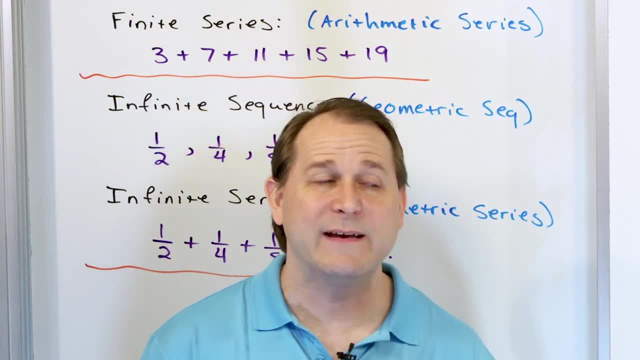 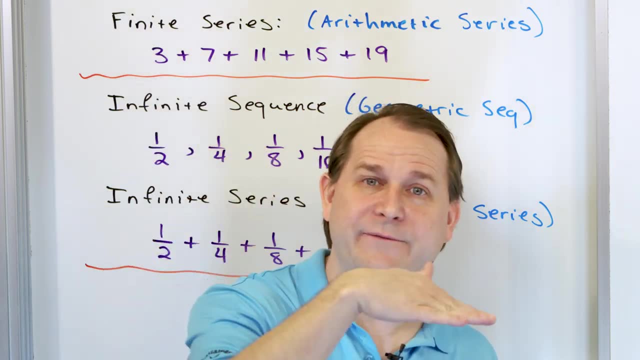 that each term is getting smaller and smaller and smaller. So sometimes- and we will discuss later down the road how you know when you can do this, but sometimes you can't. Sometimes if the terms are decreasing fast enough, even though there's an infinite number of them. 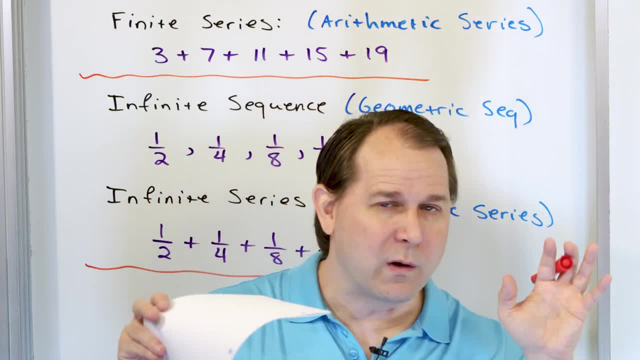 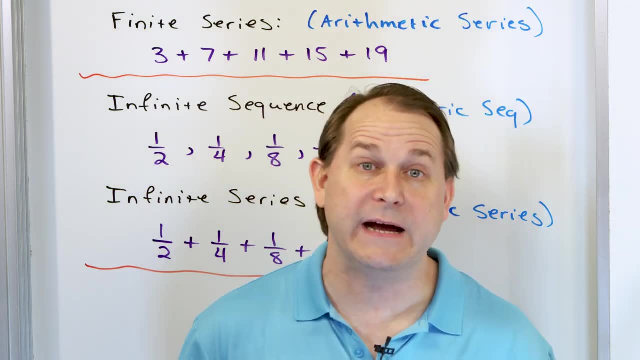 infinite, on and on and on, forever. I can still add them up, quote, unquote and get a finite number, an actual number In other words. most people think if you keep adding and adding and adding, it just goes to infinity. But if the terms are dropping really rapidly, I'll explain later how- 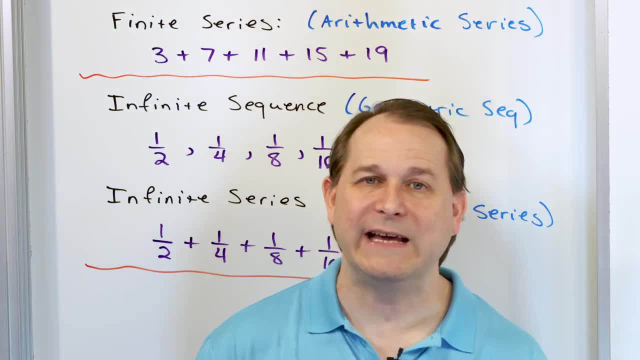 we know when that's happening. If the terms are dropping fast enough, you can actually get an answer- a finite number, even if you're adding up an infinite series like that, And that is actually a protein of calculus. We can talk about that later when we get to that subject, but that's what we're going to be doing here, when we talk about series as well. 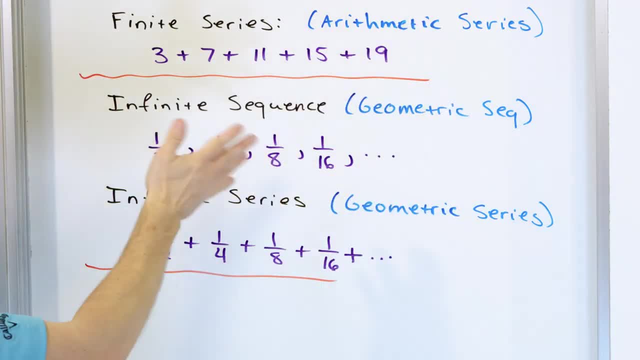 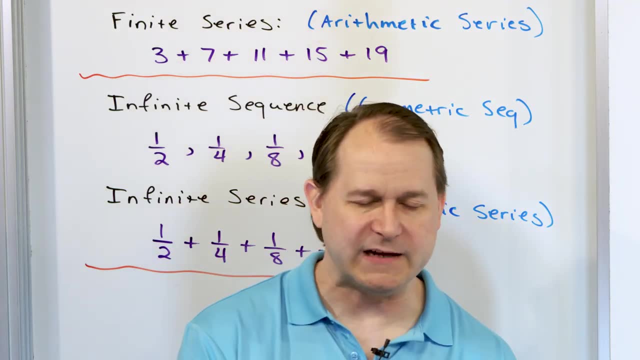 So you have finite sequences, finite series. that's easy to understand. You can add things up. You can have infinite sequences and infinite series And even in the case of an infinite series, you can still add them up and get a number sometimes. 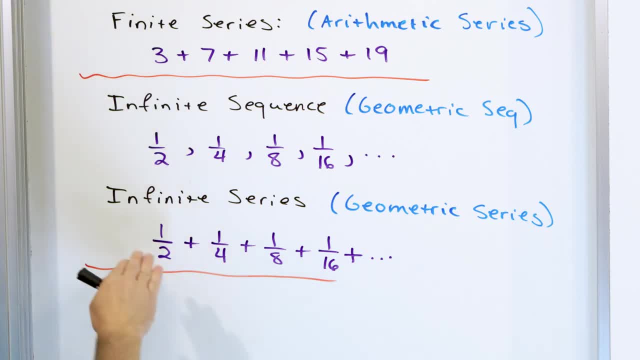 So now we have to switch gears and say: well, it's a real pain to write these numbers down with commas and with plus signs, So we have to have a way of doing it shorthand. We call it sigma notation. Sigma is the Greek word for 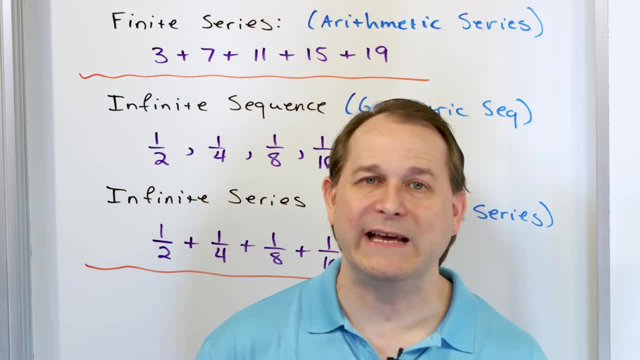 we know when that's happening. If the terms are dropping fast enough, you can actually get an answer- a finite number, even if you're adding up an infinite series like that, And that is actually a very important part of calculus. We'll talk about that later when we get to that subject, but that is what we're going to be doing here, when we talk about series as well. 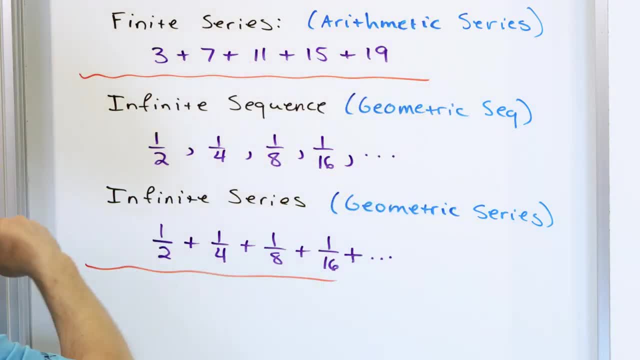 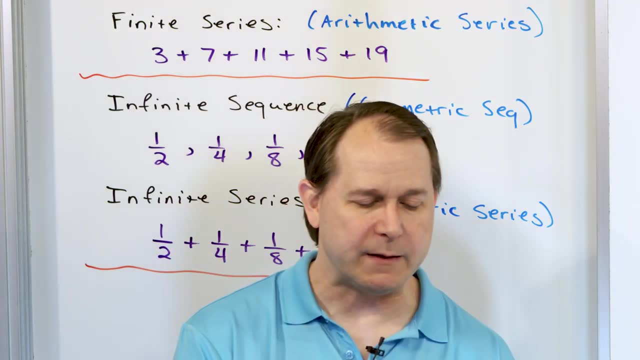 So you have finite sequences, finite series. that's easy to understand. You add things up. You can have infinite sequences, infinite series, and even in the case of an infinite series, you can still add them up and get a number sometimes. 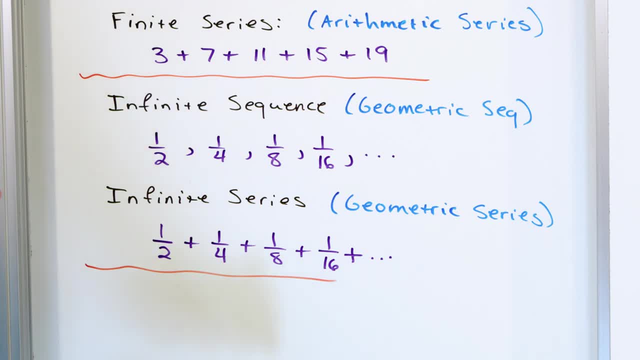 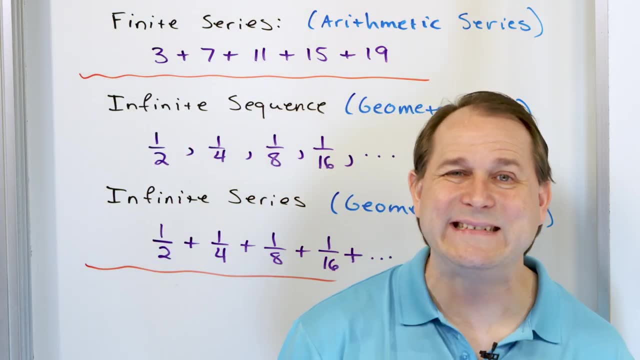 So now we have to switch gears and say: well, it's a real pain to write these numbers down with commas and with plus signs, so we have to have a way of doing it shorthand. We call it sigma notation. Sigma is the Greek word for sigma. 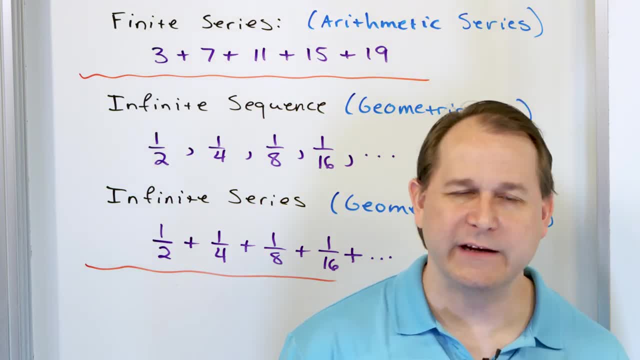 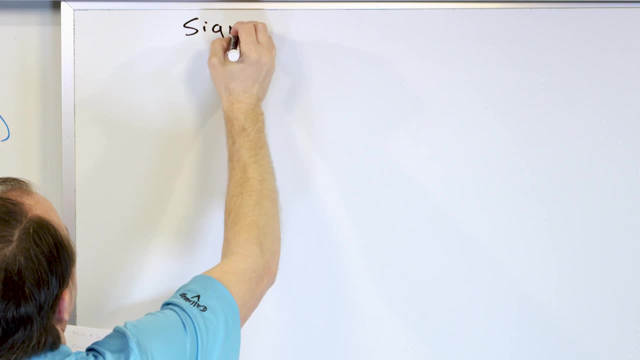 You're going to be using it over and over and over again, So the easiest way to do it is just to do it. I'm going to call it sigma notation. I'll tell you right now that it looks really scary at first, but actually when I explain it it's actually really fun, because it's something that makes your life easier. and it's kind of fun once you get the idea of how to do it. 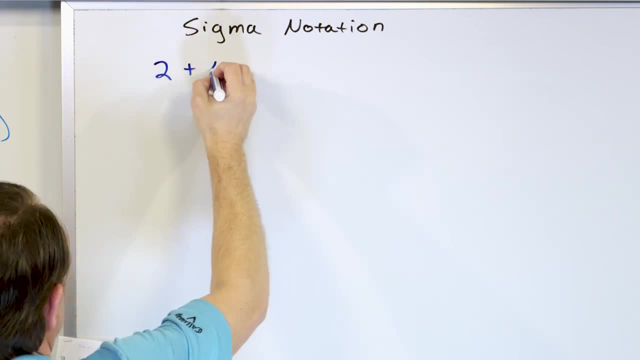 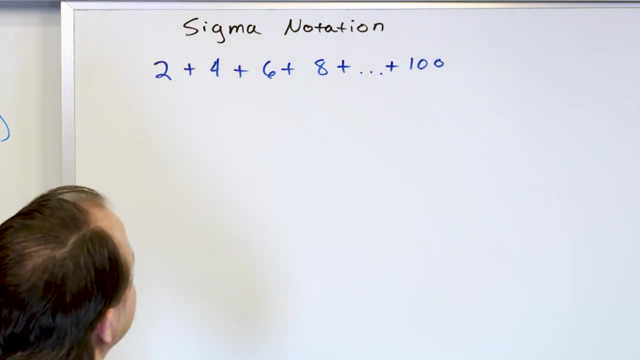 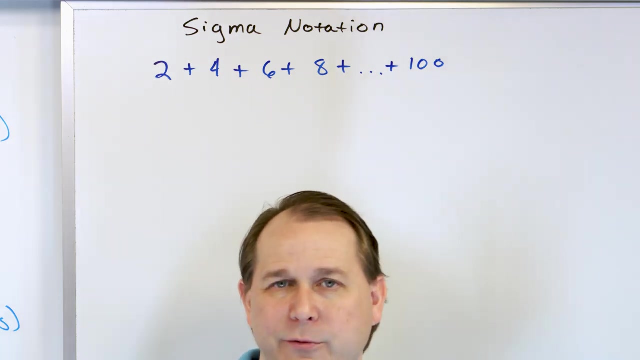 What if we have the series that looks like this: Plus dot, dot, dot, plus 100.. Now, this is not an infinite series. All I've done is put the dots here, because there's a lot of terms between 8 and 100, but 100 is the last term in this series. 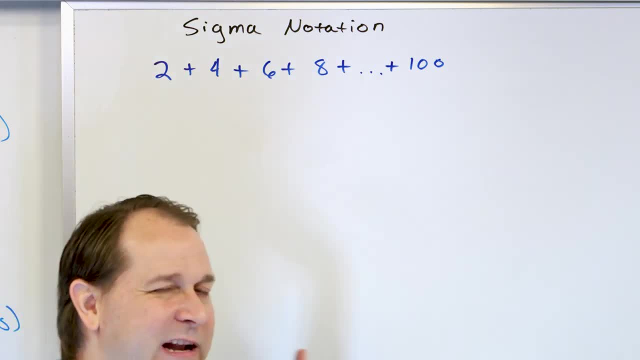 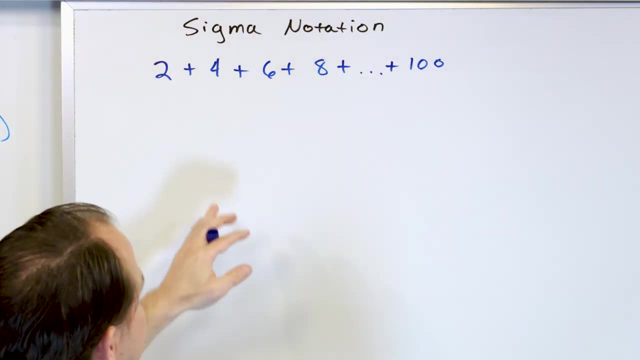 It's a series because I have plus signs everywhere. I'm adding these up And I should ask you a bonus question: What kind of series is it? Is it an arithmetic series? Is it a geometric series? Is it neither? This one is an arithmetic series because, to get the terms, I'm just adding 2 to get 4 and then 2 to get 6.. I'm adding 2 to get 8.. 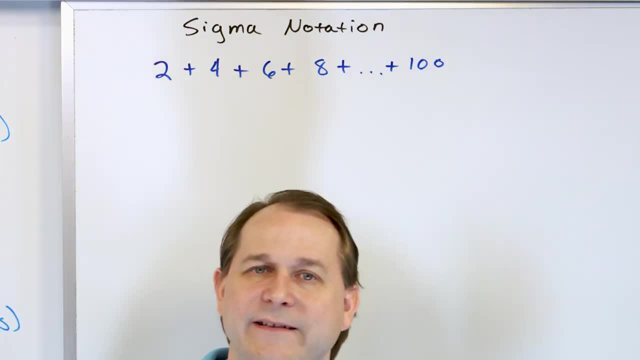 Every term in the series is just adding another number for the related sequence, the arithmetic sequence. So this is called an arithmetic series and it's a finite series because it doesn't go forever, It just stops. So obviously, writing all these terms down to 100 would take a lot of board space. So we want to simplify that. Here's how you do it: I'm just going to write it down and we're going to talk about it. 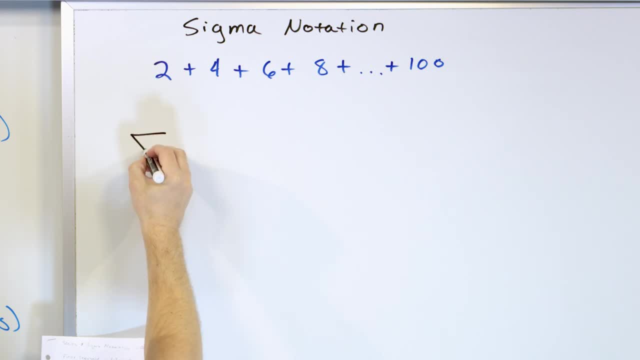 You have to get used to drawing this big little E Horizontal line, down back horizontal line. This is how I want you to write your sigmas. I don't want you to scribble some lines. I don't want you to make an E. I don't want you to do a capital, anything weird. I want it to be horizontal line, diagonal line, diagonal line, horizontal line. 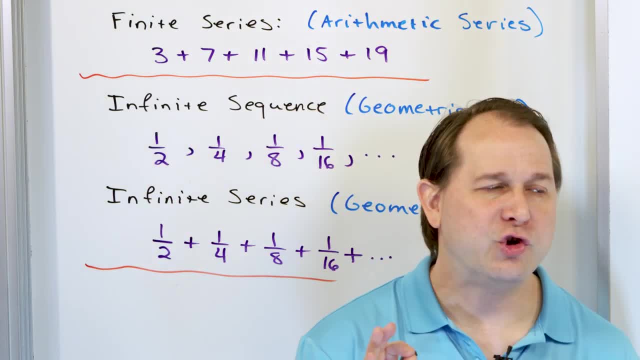 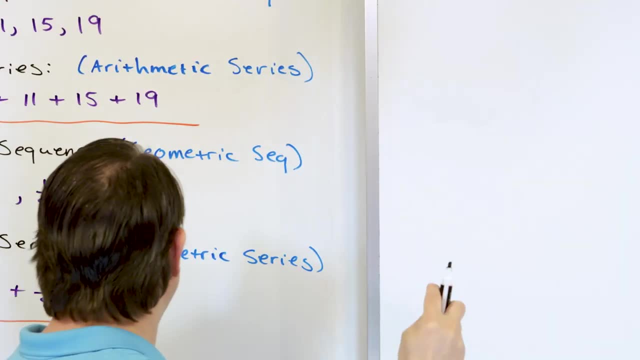 sign or it's similar to the Greek word for hand. Sign is the Greek word for hand, notation. Sigma is the Greek letter, Greek capital letter: sigma. You're going to be using it over and over and over again, So the easiest way to do it is just to do it. I'm going to call. 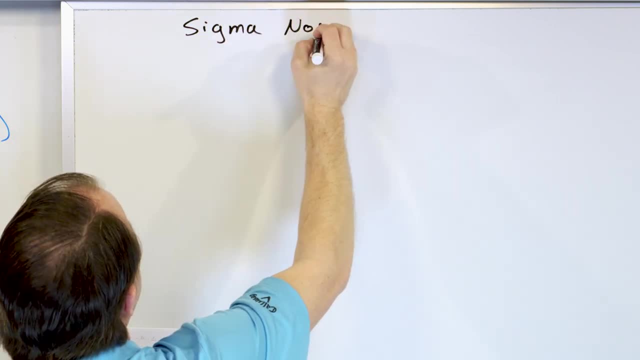 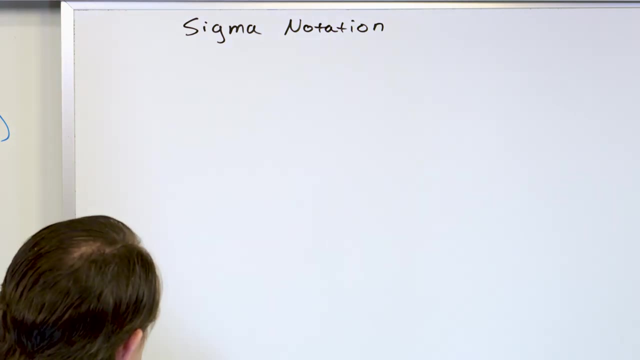 it sigma notation. I'll tell you right now that it looks really scary at first, but actually when I explain it it's actually really fun because it's something that makes your life easier. and it's kind of fun once you get the idea of how to do it. What if we have the series that looks like? 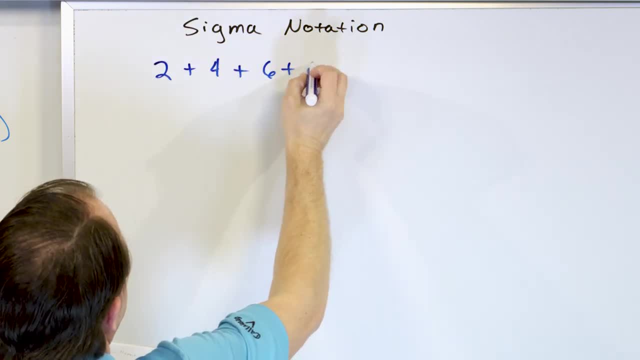 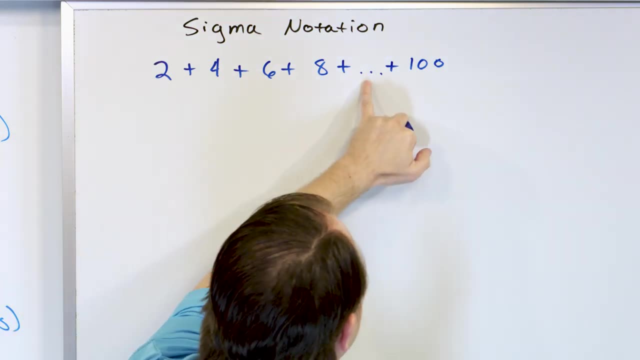 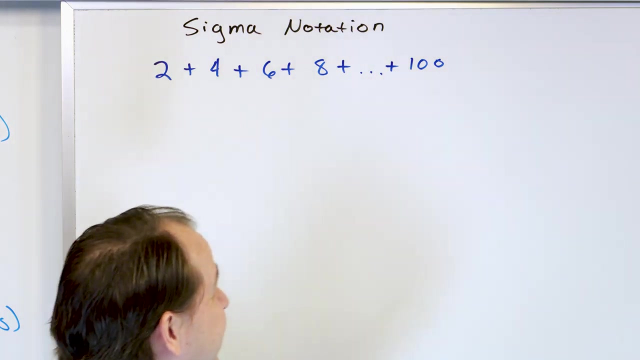 this: Two plus four plus six plus eight, plus dot, dot, dot plus 100.. Now, this is not an infinite series. All I've done is put the dots here, because there's a lot of terms between eight and 100, but 100 is the last term in this series. It's a series because I have plus signs everywhere I'm. 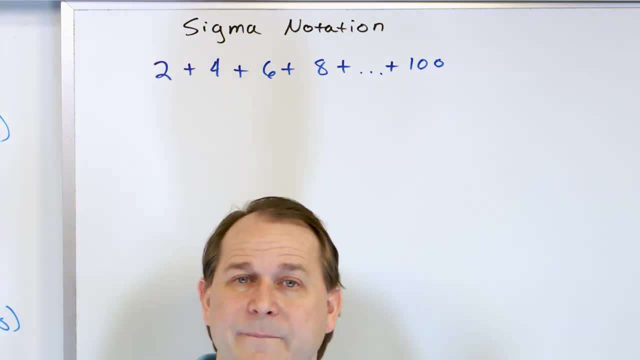 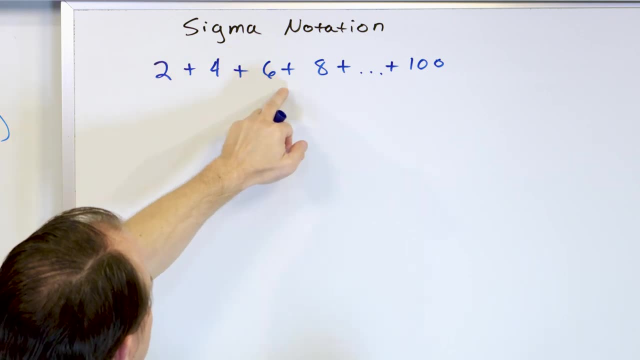 adding these up, And I should ask you a bonus question: What kind of series is it? Is it an arithmetic series? Is it a geometric series? Is it neither? This one is an arithmetic series because, to get the term, I'm just adding two to get four, and then two to get six. I'm adding two to get eight Every term. 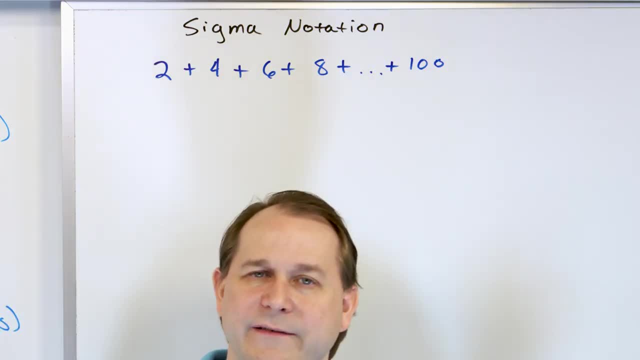 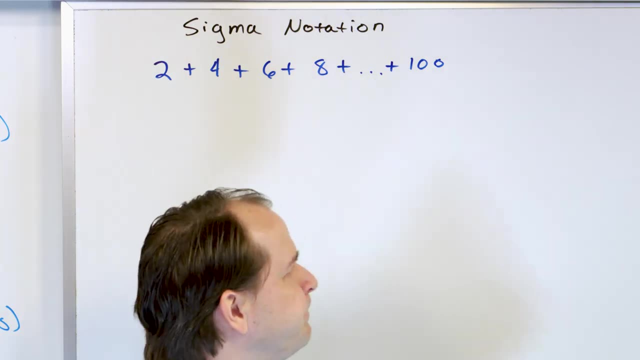 in the series is just adding another number for the related sequence, the arithmetic sequence. So this is called an arithmetic series and it's a finite series because it doesn't go forever, It just stops. So obviously, writing all these terms down to 100 would take a lot of board space. So 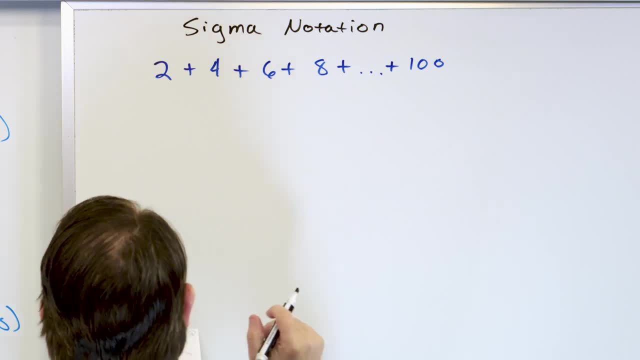 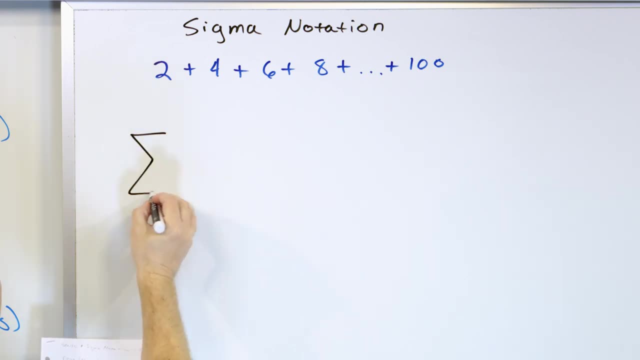 we want to simplify that. Here's how you do it. I'm just going to write it down and we're going to talk about it. You have to get used to drawing this big little E Horizontal line down back horizontal line. This is how I want you to write your sigmas. I don't want you to scribble. 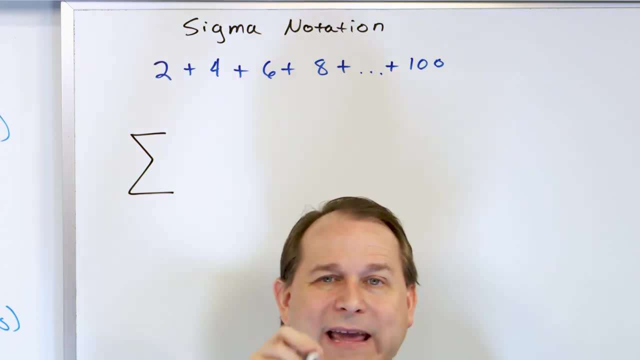 some lines. I don't want you to make an E, I don't want you to do a capital, anything weird. I want it to be horizontal line, diagonal line, diagonal line, horizontal line. That is the proper way that you write a sigma, And here is how we're going to do this. I'll explain in a minute. N is equal to. 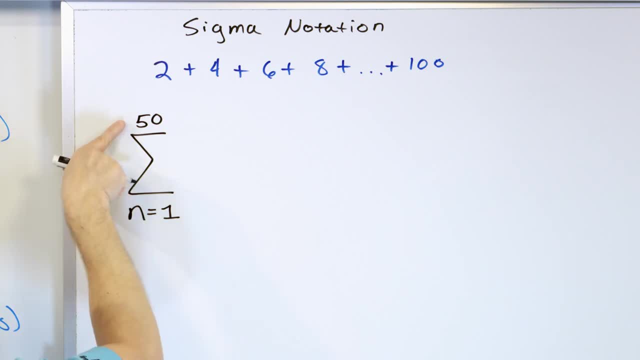 one going up to N is equal to value of 50. So N goes from one to 50. And what we're doing here is we're going to write a sigma of two times N. Now, if you've ever done any computer programming, 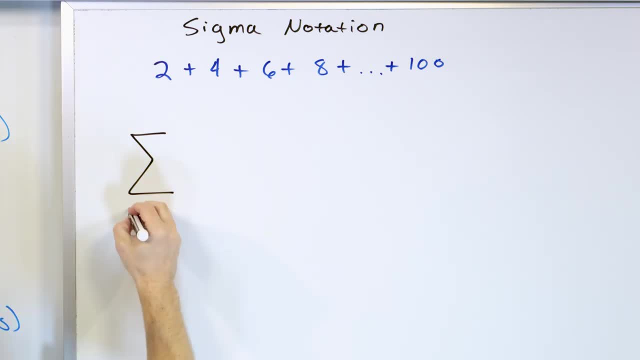 That is the proper way that you write a sigma, And here is how we're going to do this. I'll explain in a minute. N is equal to 1. going up to N is equal to value of 50. So N goes from 1 to 50. And what we're doing here inside of the sigma is 2 times N. 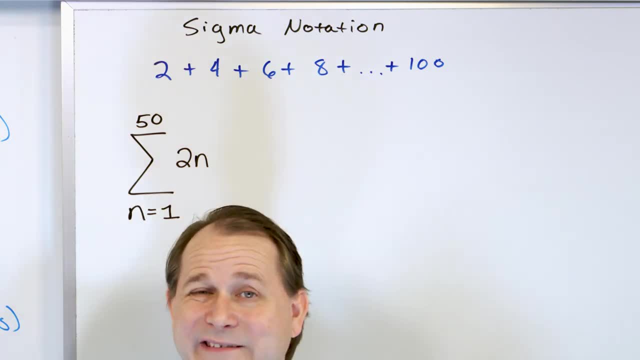 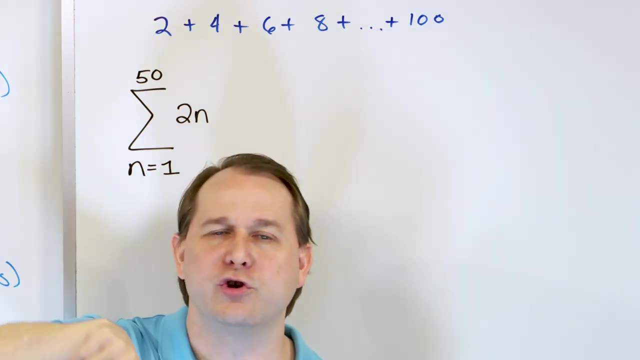 Now, if you've ever done any computing, Computer programming, it's going to actually be a lot easier for you to understand this. What I want you to see when you look at that sigma is I want you to see it as a loop. It's like a loop. You go through this little mathematical loop. 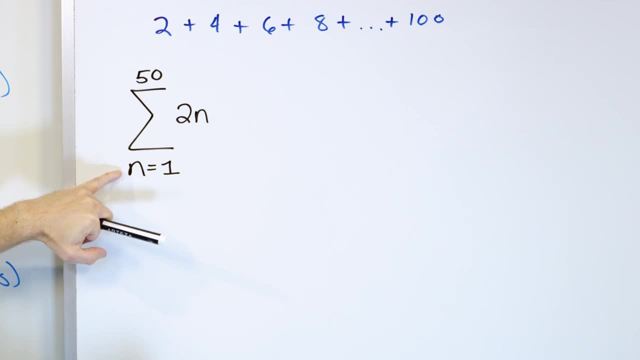 How many times do you do it? You're going to do it 50 times because what is on the bottom and what is on the top are the boundaries of the loop You start. you have to. this variable N is just a placeholder for kind of a counter that goes through the loop. 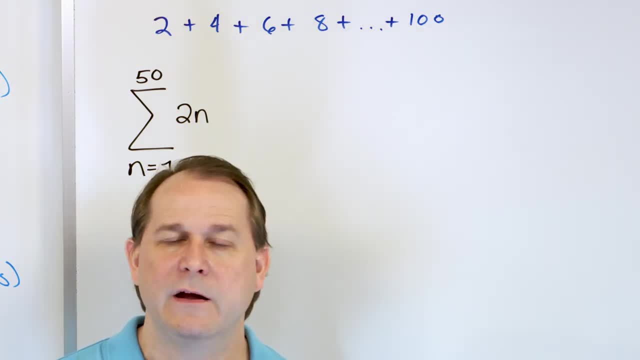 When N starts at 1,- that's the value of N- You go through the loop and then, eventually, N is 2, and then N is 3, N is 4,, 5,, 6,, 7,, all the way to N is equal to 50, and then the loop is stopping. 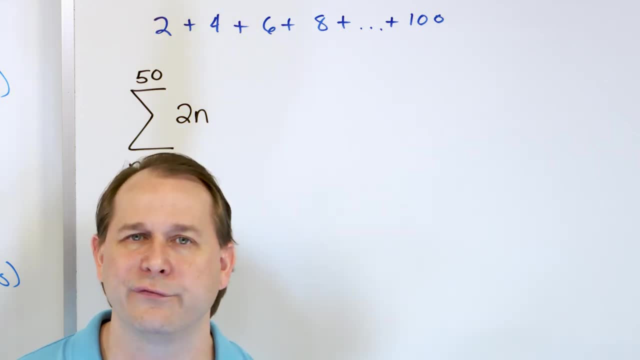 So the numbers on the top and the numbers on the bottom just tell you how many times you go through the loop. Now, what do you do in the loop? What you do is what's in here. This is what you do every time you go through the loop. 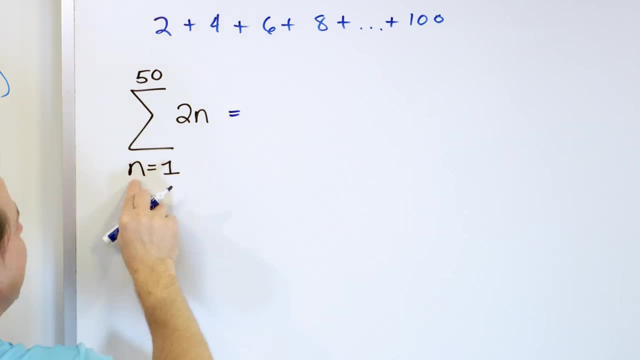 So here's how you figure it out. What you say is the first time through the loop: N is equal to 1.. What I have here is 2 times N. So what I'm going to have is 2 times N is equal to 1.. That's the first term. 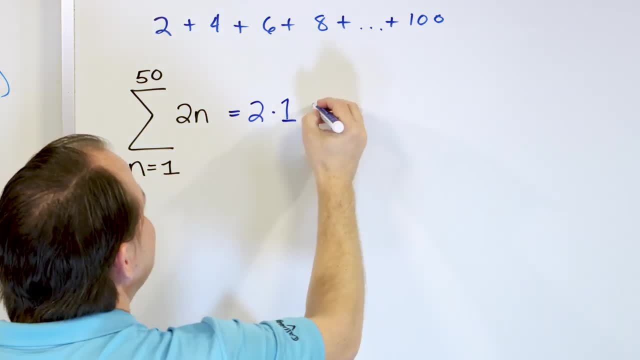 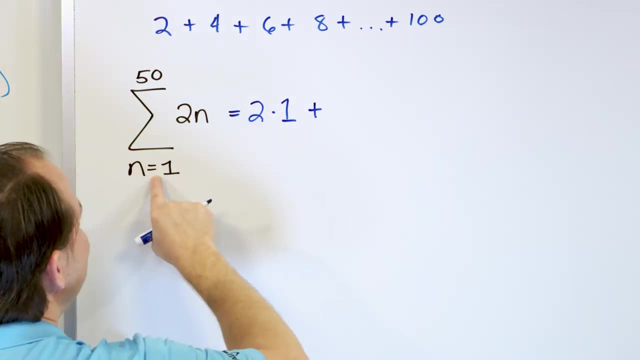 The sigma means every time. Every little term here is added together, So the plus signs are automatically included, because this is a sigma. Then I go through the next time through the loop. N is now 2.. 2 times N being 2 is going to be written like this: 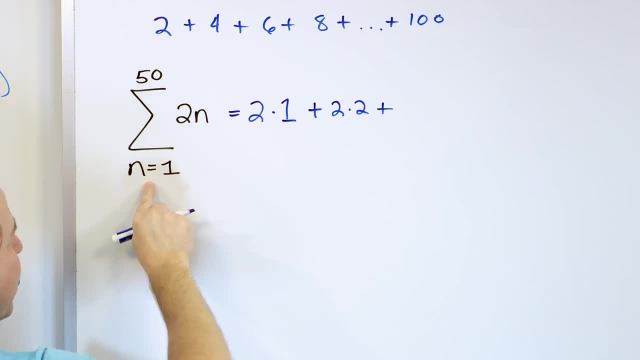 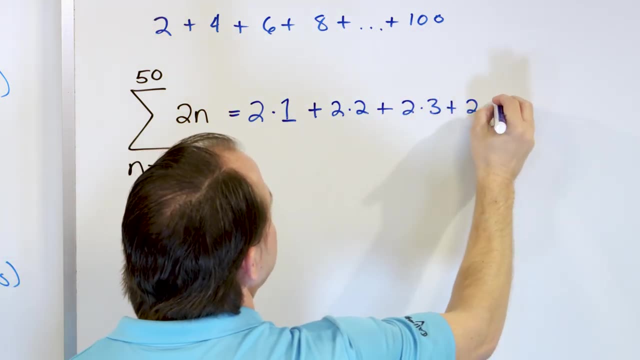 And I go back through the loop and then it's going to be: N is equal to 3, 2 times 3, so I write as 2 times 3.. I go back through the loop: N is equal to 4, 2 times 4, 2 times 4.. 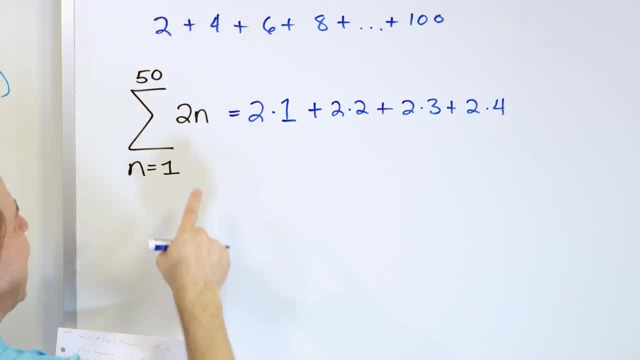 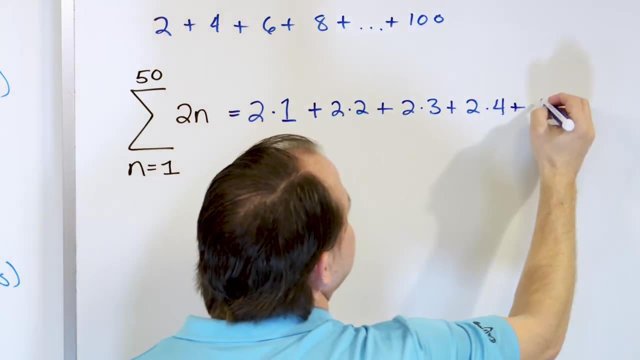 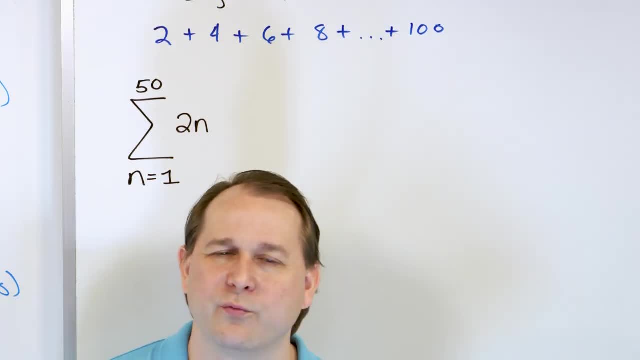 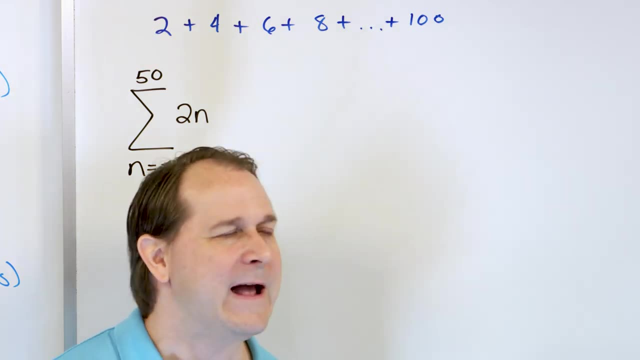 it's going to actually be a lot easier for you to understand this. What I want you to see when you look at that sigma is I want you to see it as a loop. It's like a loop. You go through this little mathematical loop. How many times do you do it? You're going to do it 50 times, because what is? 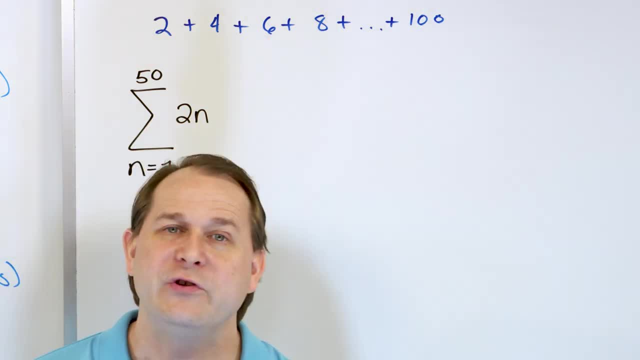 on the bottom, and what is on the top are the boundaries of the loop You start. you have to. this variable N is just a placeholder for kind of a counter that goes through the loop. N starts at one. That's the value of N. You go through the loop and then eventually N is two. 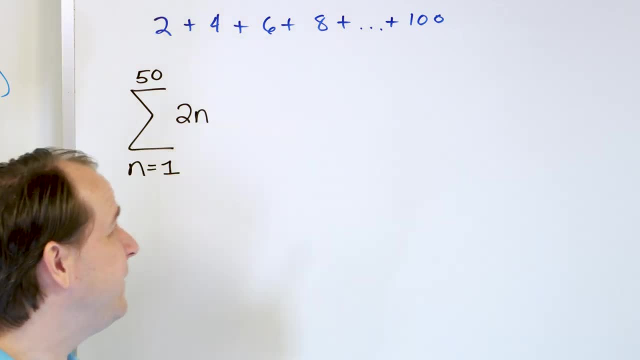 and then N is three, N is four, five, six, seven, all the way to N is equal to 50. And then the loop is stopping. So the numbers on the top and the numbers on the bottom just tell you how many times. 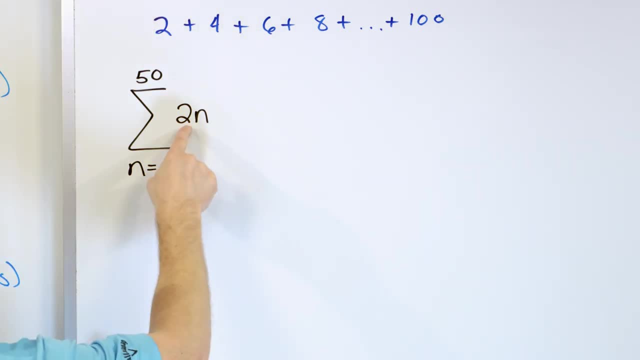 you go through the loop. Now, what do you do in the loop? What you do is what's in here. This is what you do every time you go through the loop. So here's how you figure it out. What you say is: 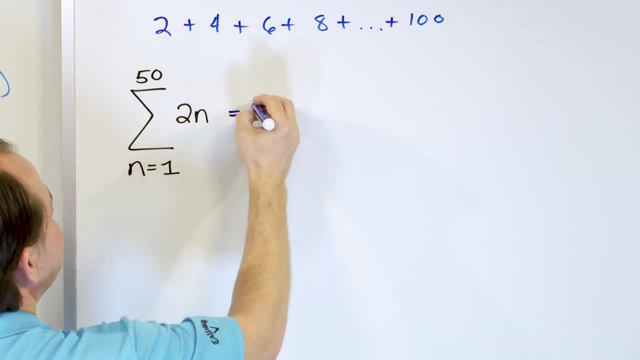 the first time through the loop, N is equal to one. What I have here is two times N, So what I'm going to have is two times N is equal to one. That's the first time through the loop. And then the sigma means every little term here is added together, So the plus signs are automatically. 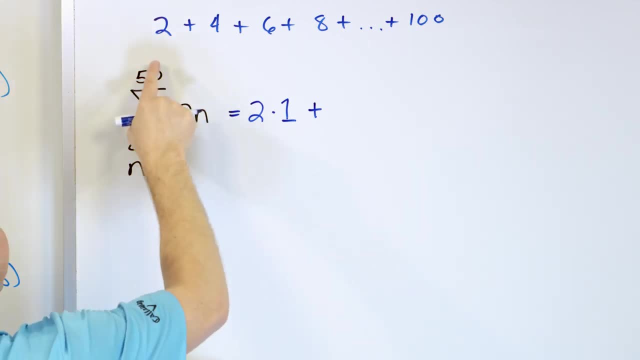 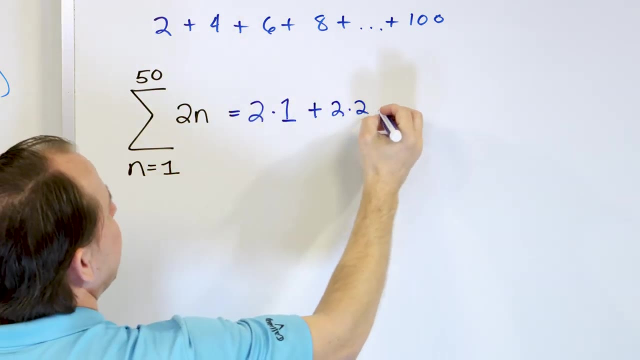 included because this is a sigma. Then I go through the next time through the loop. N is now two, Two times N being two is going to be written like this: And I go back through the loop and then it's going to be: N is equal to three, two times three. So I write as two times three. I go back. 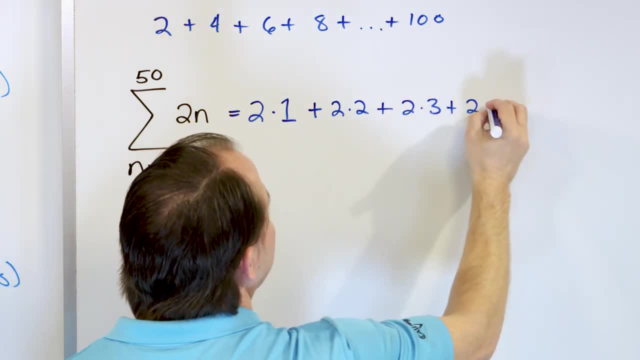 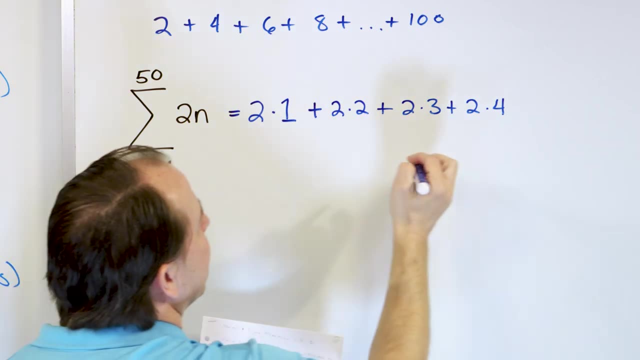 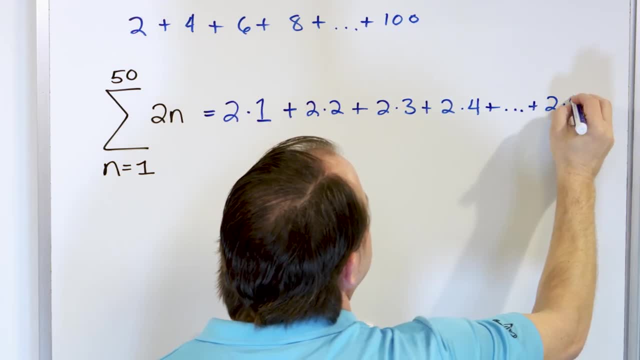 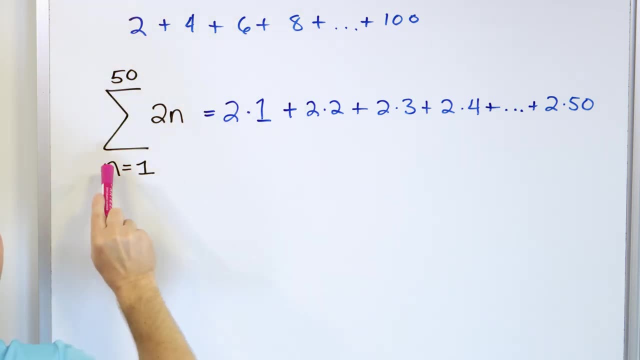 N is equal to 50, dot, dot, dot, two times 50.. All right, So what's happening is you're going through and you're doing this mathematical calculation as N goes bigger, bigger, bigger, bigger. Now, what does this do for us? What it does for us is the following thing: Two times one. 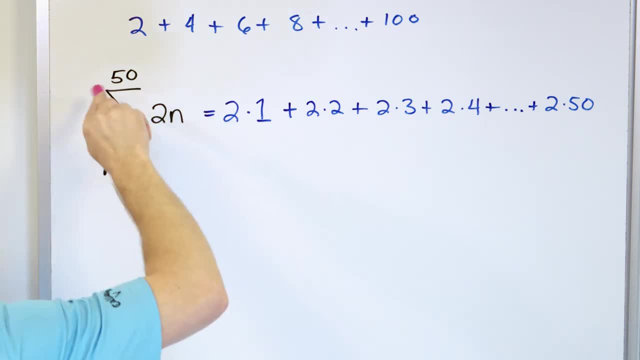 All right. So what's happening is you're going through and you're doing this mathematical calculation as N goes bigger, bigger, bigger, bigger. Now, what does this do for us? What it does for us is the following thing: 2 times 1 is 2.. 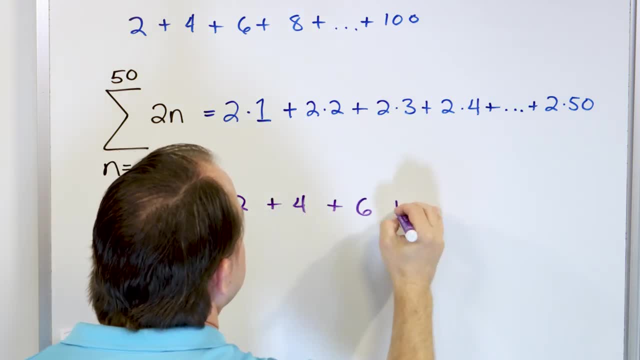 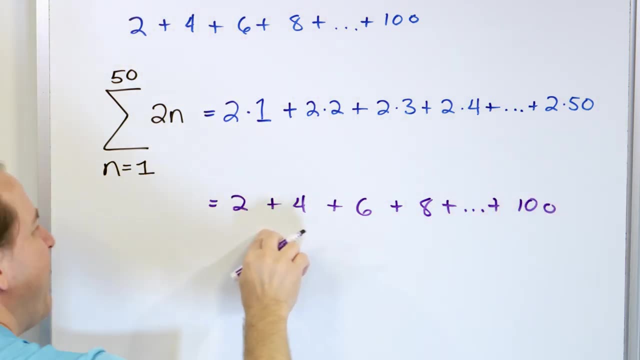 Then we have 4.. Then we have 6., Then we have 8, dot, dot, dot, And then we have 100.. Notice that the series that comes back out of this calculation is the same series I started with. So what I'm trying to say is that you can write these series down with plus signs if you want to. 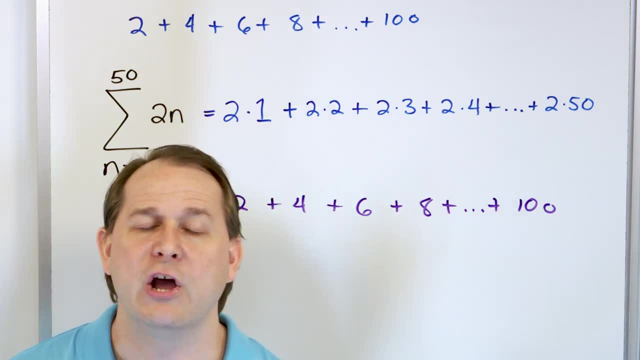 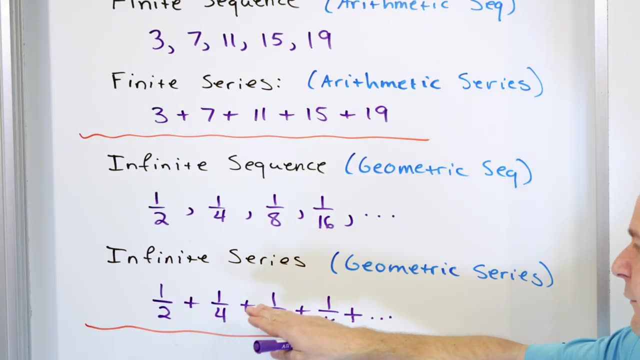 but what's going to happen is you might have a series with 100 or 200 terms, You might have 3,000 terms, You might even have infinity terms, because, guess what? Later on, when we have an infinite series, we're going to have infinite terms that need to be added together. 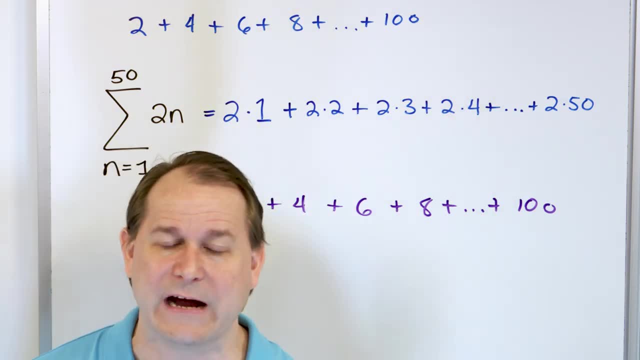 So we don't want to spend our whole page writing all this. We want to write all these terms down, so we have a shorthand way of putting it. This is a little calculational loop that represents the entire series, So I don't have to write all this stuff down every time. 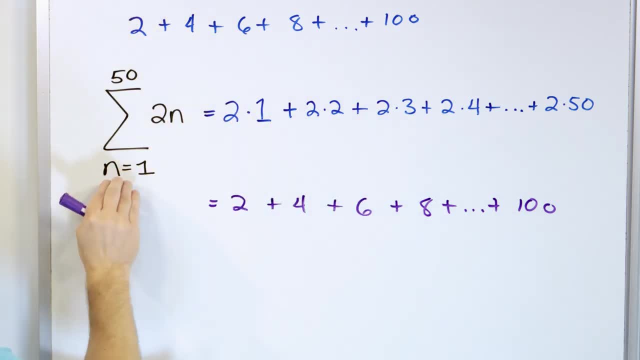 This thing right here, this black stuff right here, represents the series, Because, as N goes from 1 to 50, when I do this calculation I recover all of these terms that are existing in the original thing. So the title of the lesson was called Series in Sigma Notation. 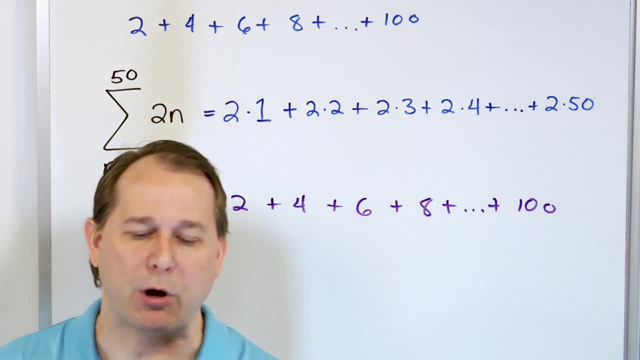 The first part of the lesson is for me to explain what a series is, but the second part is the Sigma Notation. That's this part. So the rest of the lesson, all we're going to do is I'm going to show you how to use the Sigma Notation. 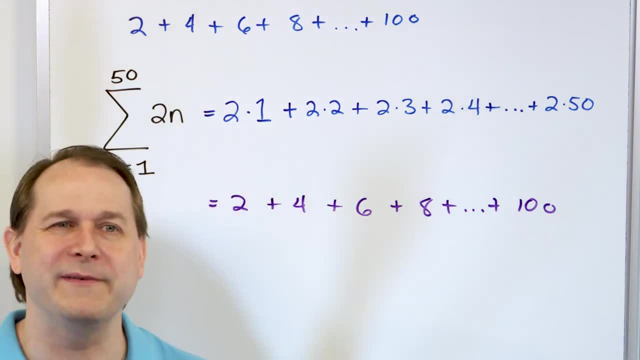 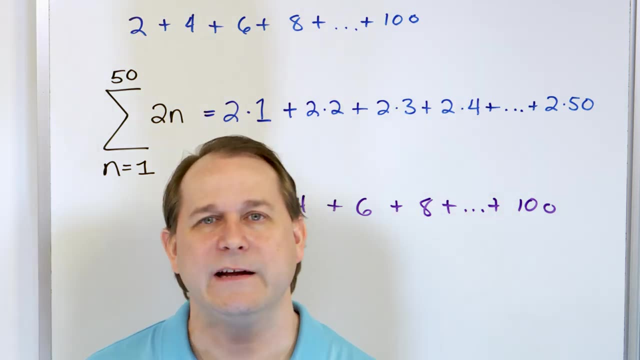 We're going to do a lot of examples. I'll show you how to get the terms. I'll show you how to take the terms and write down the Sigma Notation. That's all we're doing. You have to get comfortable with that, because we're going to be using that in future lessons. 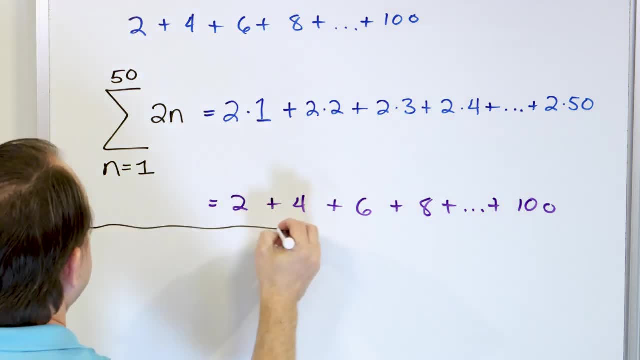 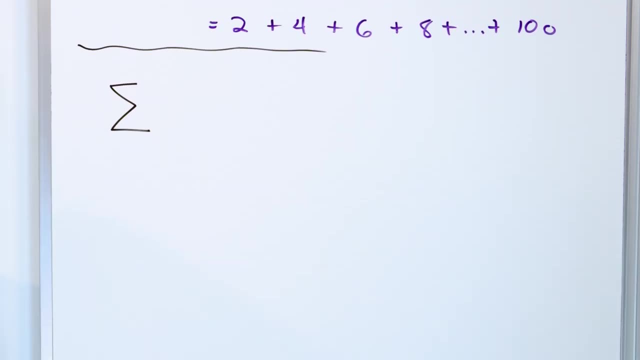 So that was our first little example of Sigma Notation. Let's do another one. Here's another series. Here it goes. My Sigmas are not perfect, but that's more or less how I want you to write it. Let's say that n goes from 1 up to. 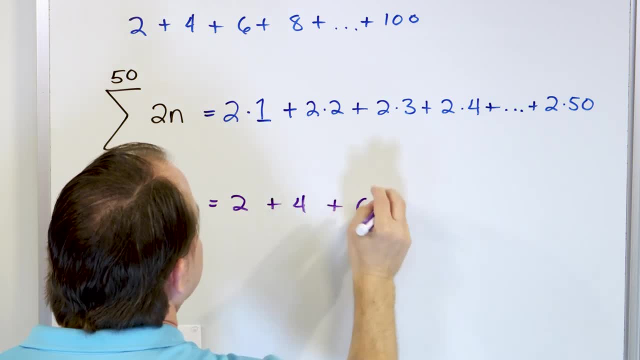 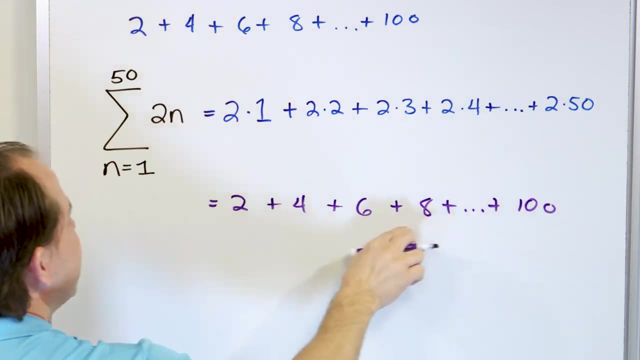 is two, Then we have four, Then we have six, Then we have eight, dot, dot, dot, And then we have 100.. Notice that the series that comes back out of this calculation is the same series I started with. So what I'm trying to say is that you can write the series down with plus signs if you want. 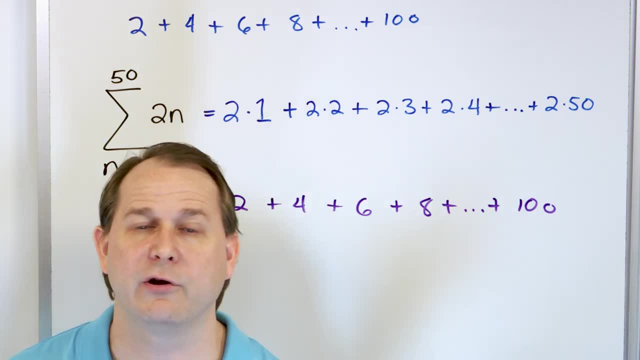 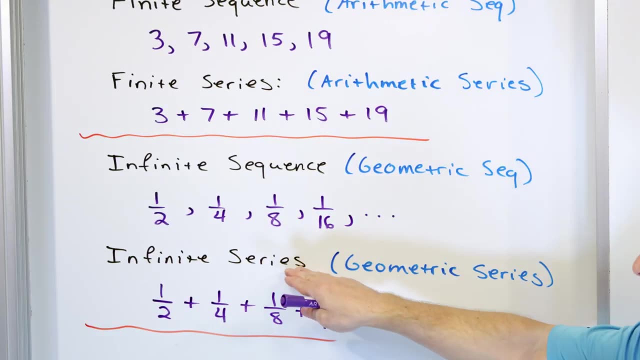 to. but what's going to happen is you might have a series with a hundred or 200 terms, You might have 3000 terms, You might even have infinity terms, because, guess what, Later on you're going to have an infinite series. We're going to have infinite terms that need to be added together. So we don't 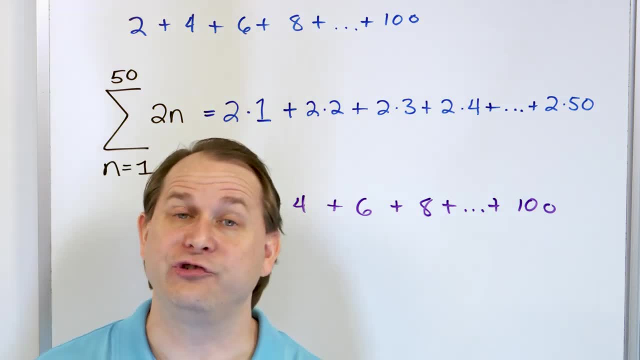 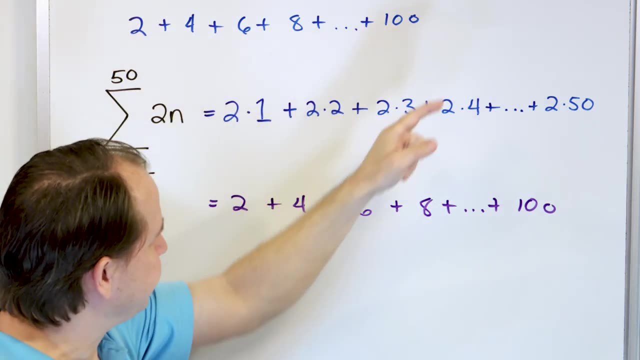 want to spend our whole page writing all these terms down, So we have a shorthand way of putting it. This is a little calculational loop that represents the entire series, So I don't have to write all this stuff down every time. This thing right here, this black stuff right here. 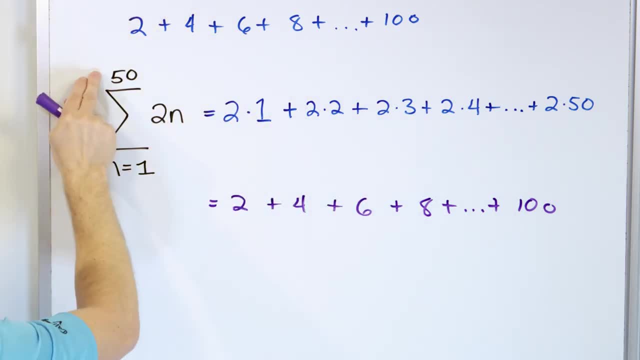 represents the series because, as N goes from one to 50, when I do this calculation I recover all of these terms that are existing in the original, So the title of the lesson was called series and sigma notation. The first part of the lesson is: 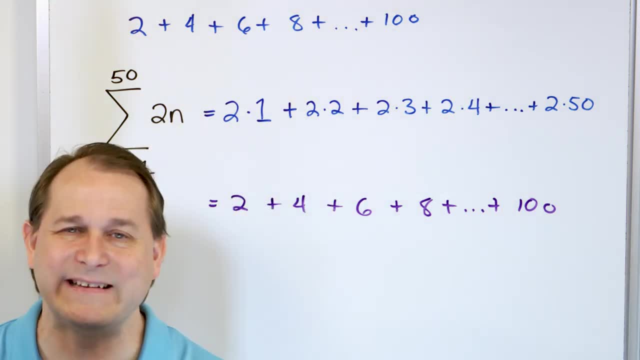 for me to explain what a series is, which I've done. The second part is the sigma notation. That's this part. So the rest of the lesson, all we're going to do is I'm going to show you how to use the sigma notation. We're going to do a lot of examples. I'll show you how to get the terms. 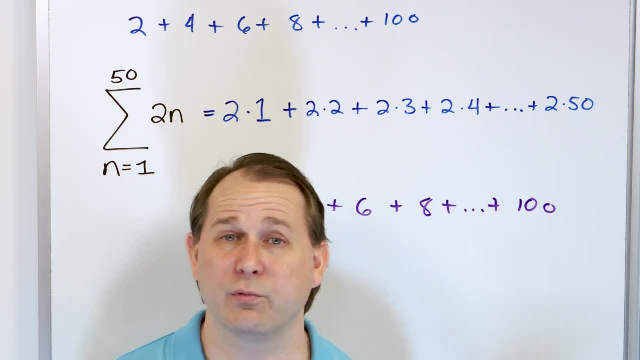 I'll show you how to take the terms and write down the sigma notation. That's all we're doing. You have to get comfortable with that, because we're going to be using that in future lessons. All right, So that was our first little example. 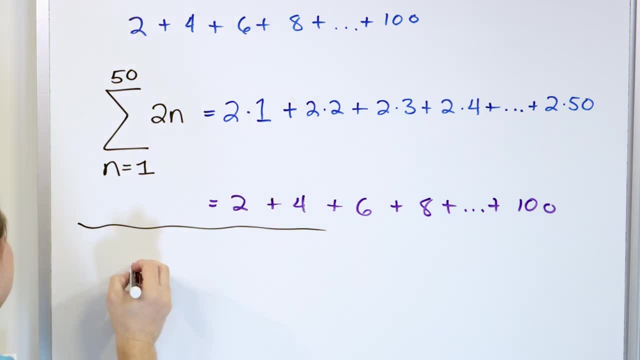 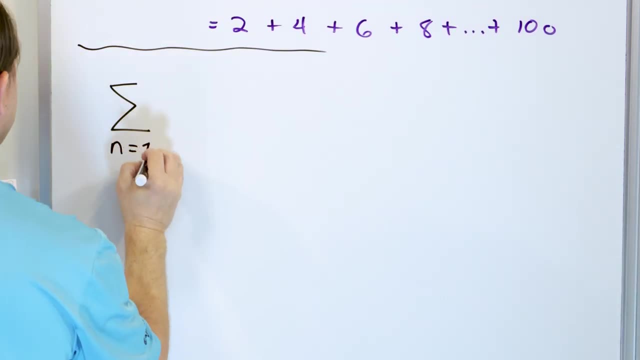 Of sigma notation, Let's do another one. Here's another series. Here goes My sigmas are not perfect, but that's more or less how I want you to write it. Let's say the N goes from one up to, instead of 50, we're going to only go to up to 10.. And let's say the little calculation: we're 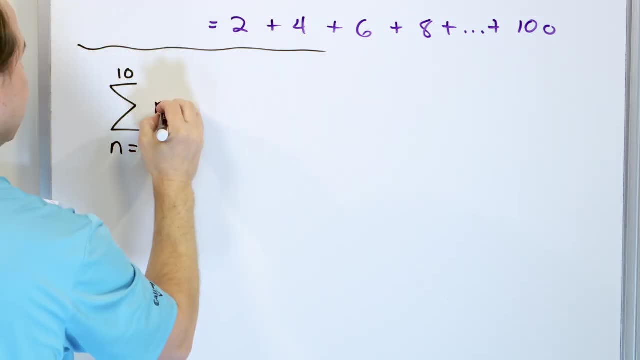 doing every time we go through the loop is not this: It's going to be N squared into the power of two. So this loop, how many times do you think we go through that loop? We only go through this loop 10 times, because N goes from one up to 10.. 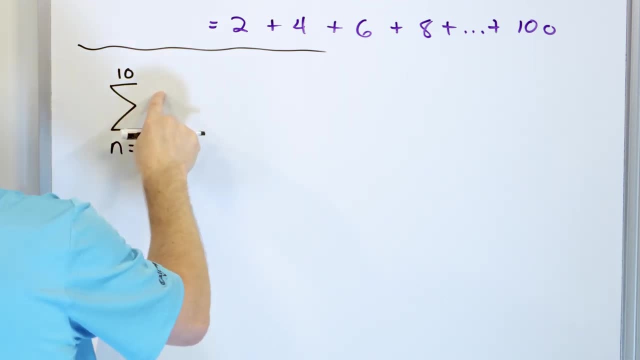 Instead of 50,, we're going to only go up to 10.. And let's say, the little calculation we're doing every time we go through the loop is not this: It's going to be n squared n to the power of 2.. 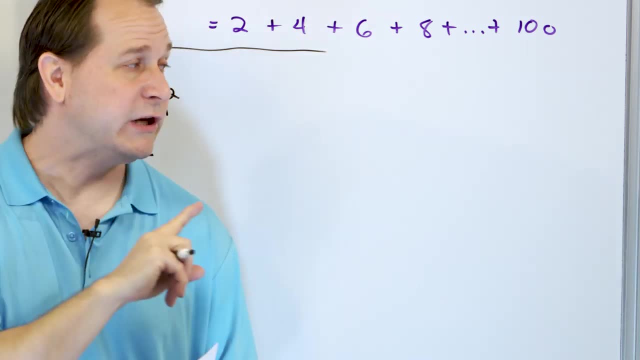 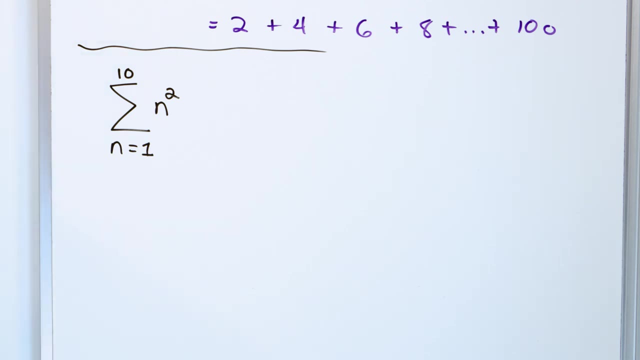 So this loop? how many times do you think we go through that loop? We only go through this loop 10 times, because n goes from 1 up to 10.. In fact, it's probably a good idea for me to label a few things for you here. 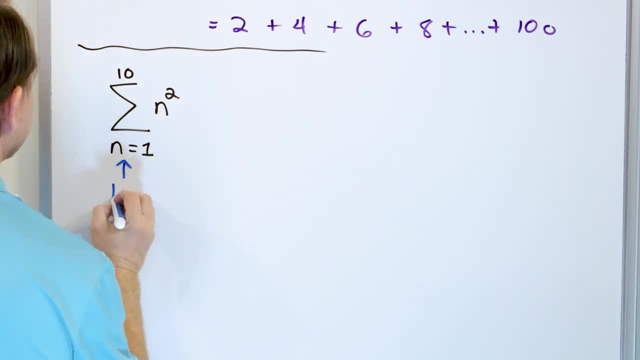 Label a few things. So this thing is called the lower limit of the sum. This thing right here is called the upper limit. These things together are called the limits. These things together are called the limits of the sum. This thing right here, the actual calculation that we do. 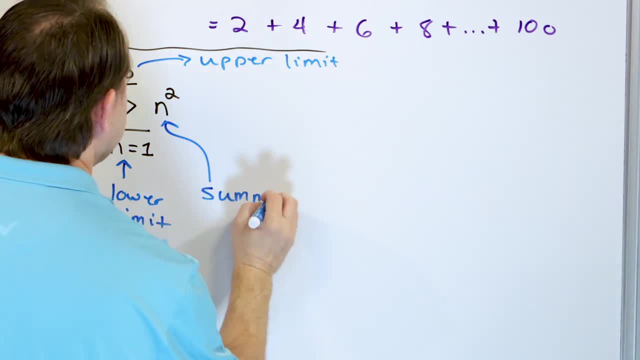 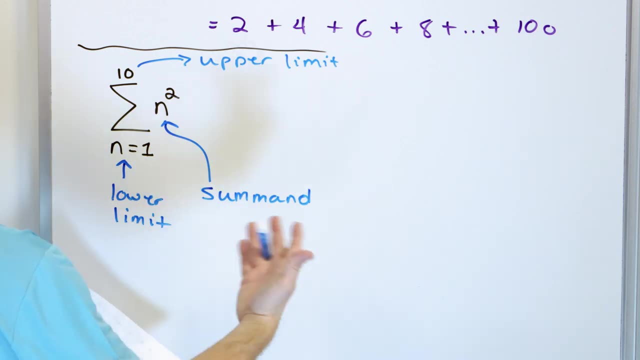 this thing is called the sum end, Sum end. Some problem says: hey, write down a sigma where the sum end is equal to whatever That word just means. that's the calculation you're doing in there. So we have the upper limit, we have the lower limit. 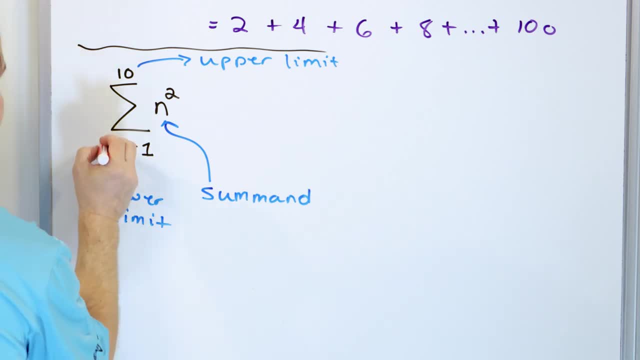 and then specifically this variable that we're using. In this case it's n, This variable right here. this thing is called the index, So if I were to write it in words, I might say: this series can be written with the variable n as the index. 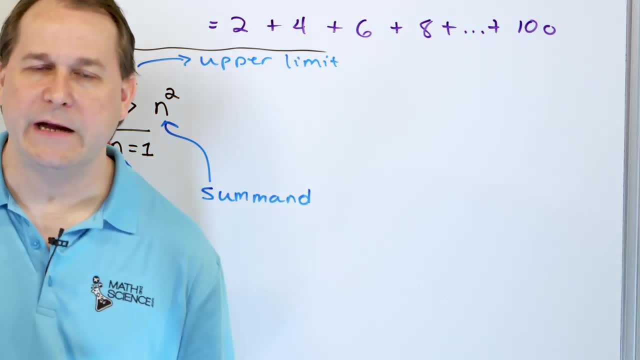 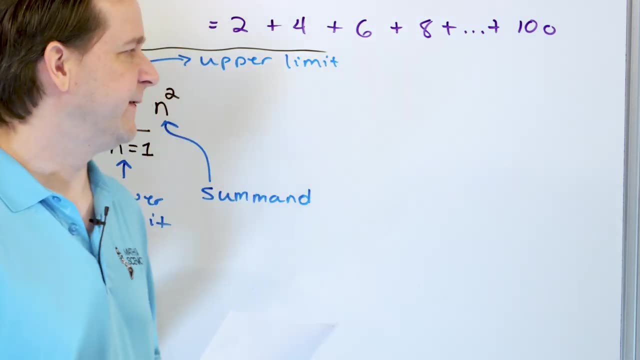 with a lower limit of 1 and an upper limit of 10, where the sum end is equal to n squared. Now. would I ever really write that down? No, but that's what those words mean in context. So how do we then proceed? 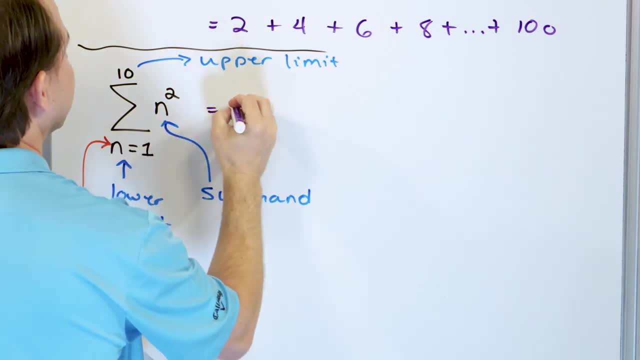 What we're gonna have is: n is gonna be 1, then we're gonna square it, so it's gonna be 1 squared, Then we're gonna go through again. n is gonna be 2, then we're gonna square it. 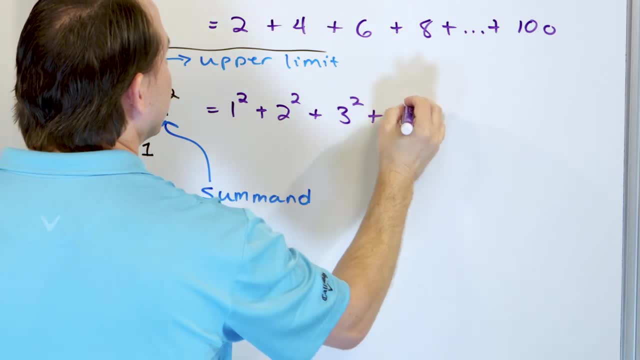 Then n is gonna be 3, then we're gonna square it. You see the pattern: n is gonna be 4, then we're gonna square it. We're gonna go all the way through dot, dot, dot, to the final value of n, which is 10,. 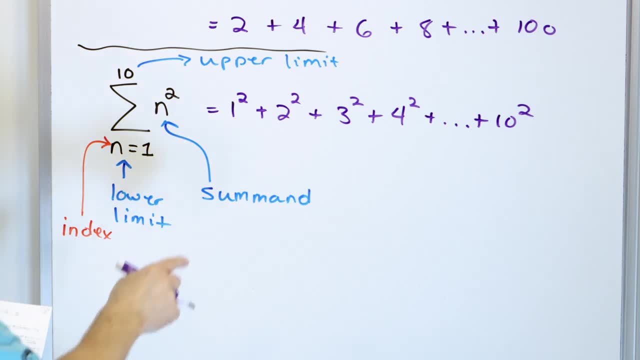 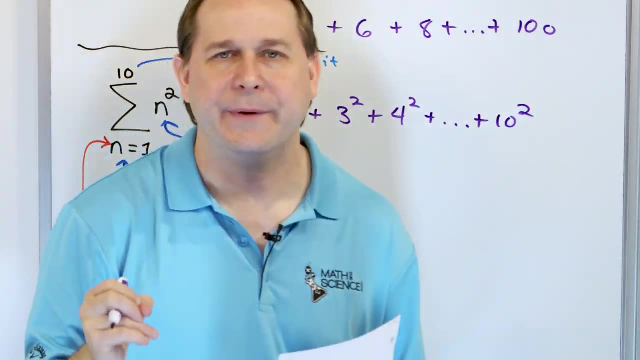 then we're going to square it. Now, of course, I can square these numbers and I can then actually add them up, just like I could add them up here. I don't actually care about finding the sum right now. Right now, we're just learning. 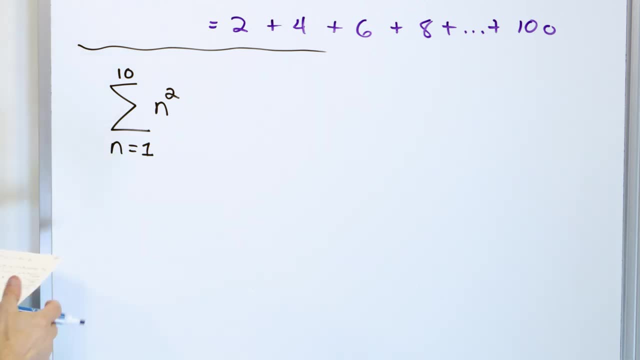 In fact, it's probably a good idea for me to label a few things for you Here. Label a few things for you. So. this thing is called the lower limit of the sum, This thing right here is called the upper limit. These things together are called the limits. These things together are called the. 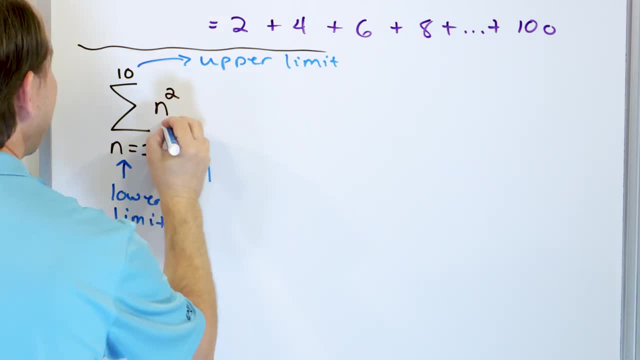 limits of the sum. This thing- right here, the actual calculation- is called the upper limit of the sum. This thing is called the sum end. So when you say some problem says hey, do a, write down a sigma where the sum end is equal to whatever, that word just means. that's the calculation you're doing in. 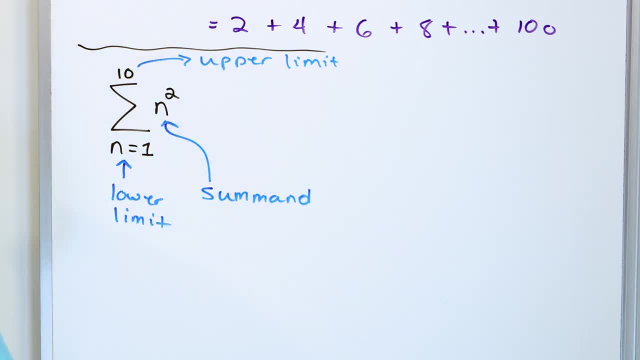 there. So we have the upper limit, We have the lower limit And then, specifically, this variable that we're using- in this case it's N, This variable right here, this thing is called the index. So if I were to write it in words, I might say this series: 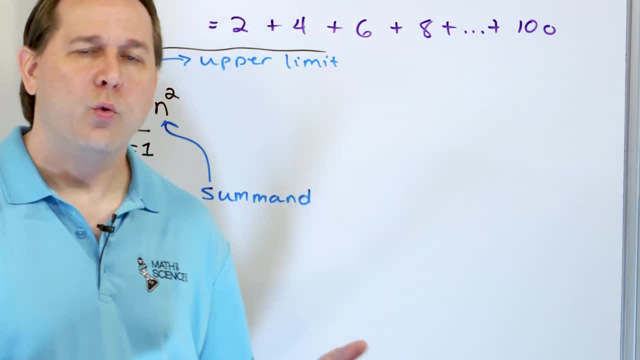 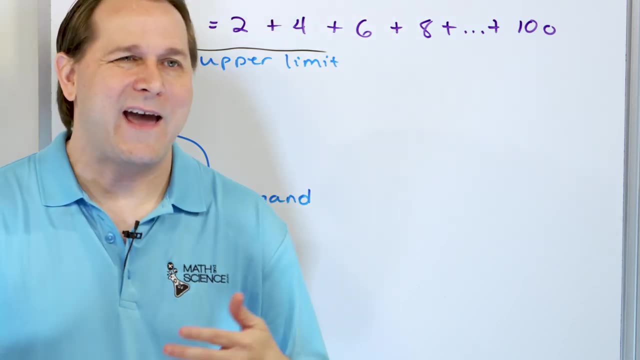 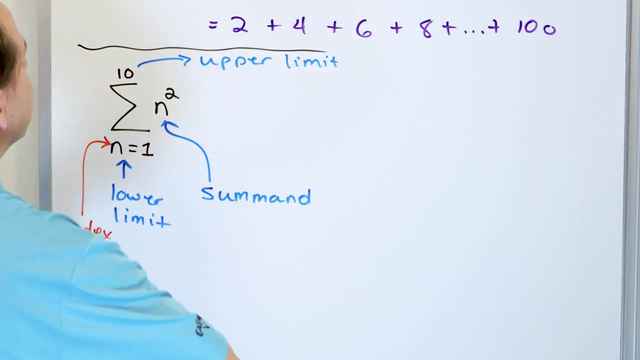 can be written with the variable N as the index, with a lower limit of one and an upper limit of 10, where the sum end is equal to N squared. Now, would I ever really write that down? No, but that's what those words mean in context. So how do we then proceed? What we're going to have, 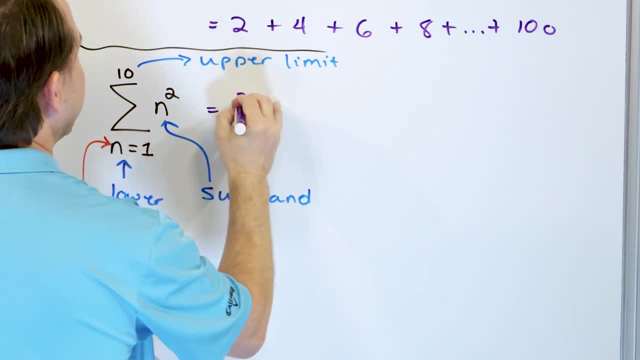 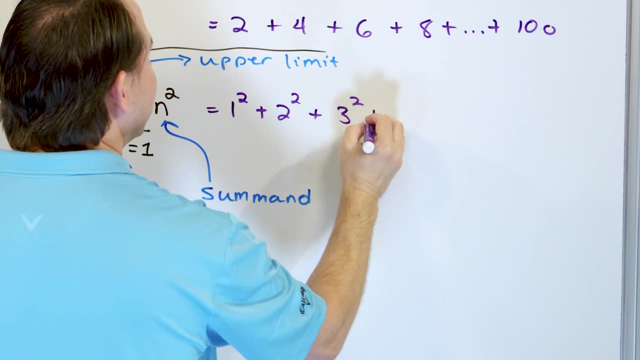 is: N is going to be one, then we're going to square it. So it's going to be one squared, Then we're going to go through again. N is going to be two, then we're going to square it. Then N is going to be three, then we're going to square it. You see the pattern. 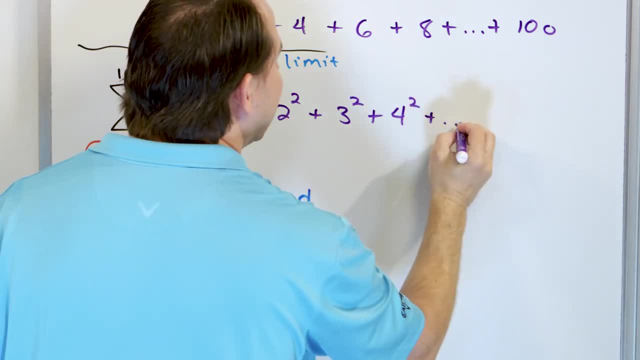 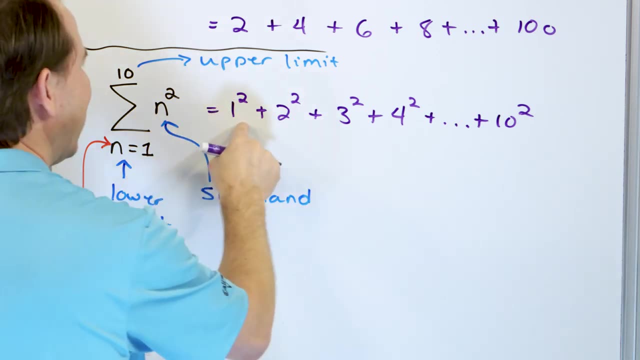 it's going to be four, then we're going to square it. We're going to go all the way through dot, dot, dot, to the final value of N, which is 10. Then we're going to square it. Now, of course, I can square these numbers and I can then actually add them up, just like I could. 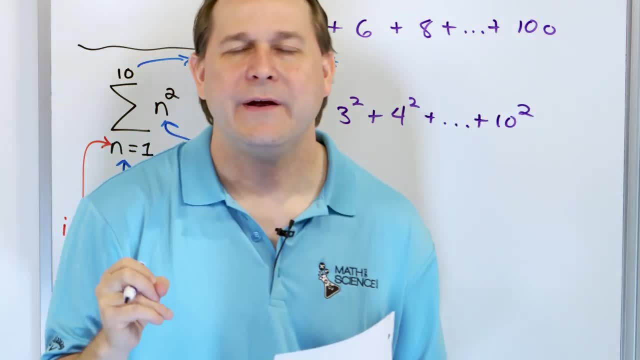 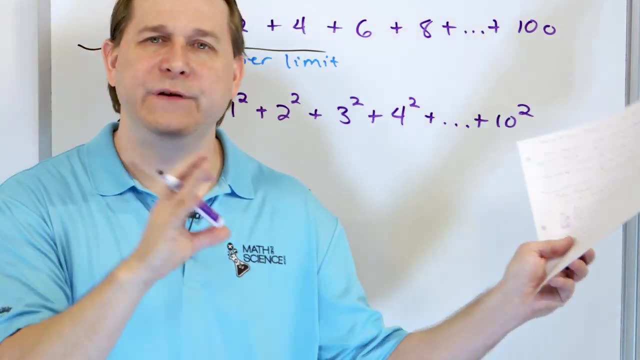 add them up here. I don't actually care about finding the sum right now. Right now, we're just learning how to write down the sigma notation. We're going to write down how to represent the sum. In a future lessons we'll talk about how to calculate the sum, because there's actually 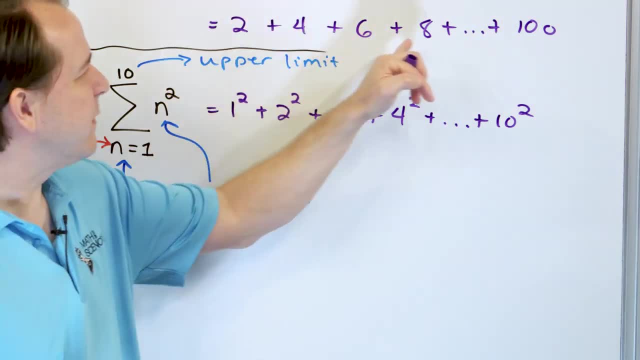 shortcut ways to actually add up. If you had to add up all these numbers to 100, it would take a long time. You'd have to use a calculator. There are quick ways to add up the numbers. Don't worry about finding the sum right. 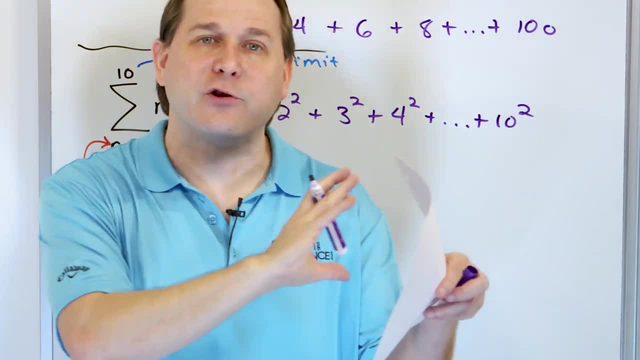 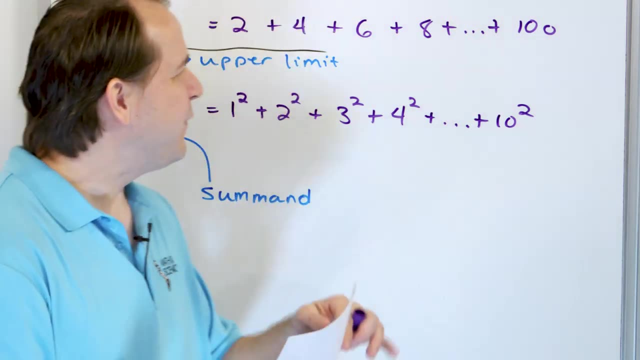 how to write down the sigma notation. We're gonna write down how to represent the sum. In a future lessons we'll talk about how to calculate the sum, because there's actually shortcut ways to actually add up. If you had to add up all these numbers to 100,. 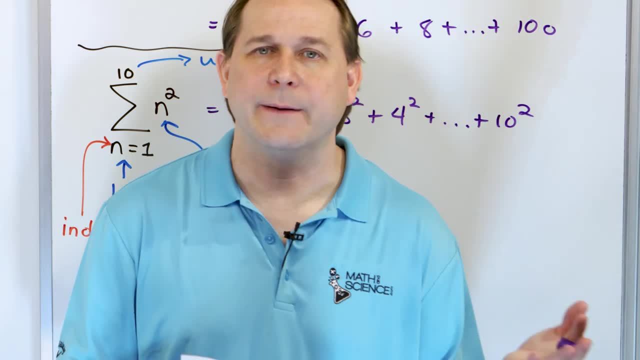 it would take a long time. You'd have to use a calculator. There are quick ways to add up the numbers. Don't worry about finding the sum right now. Right now, we're just writing down how to represent the sum, right. 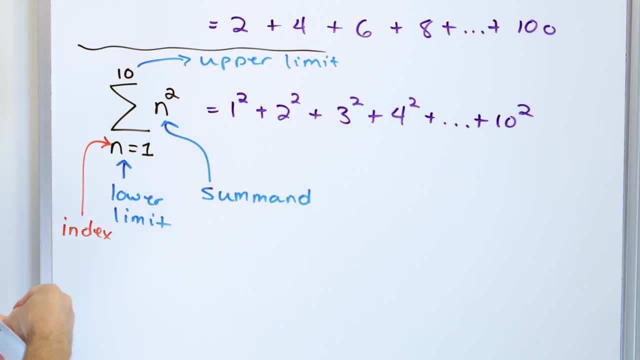 So I don't care about squaring the stuff and adding it, I just care about you knowing that this equals this. One thing that I wanna make absolutely crystal clear is that this index that we're using, this n, this variable n, it's what we call a dummy variable. 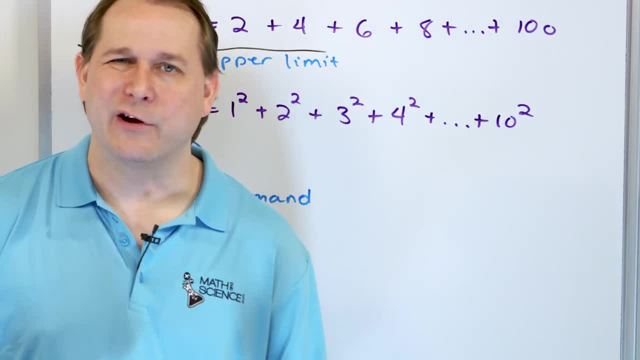 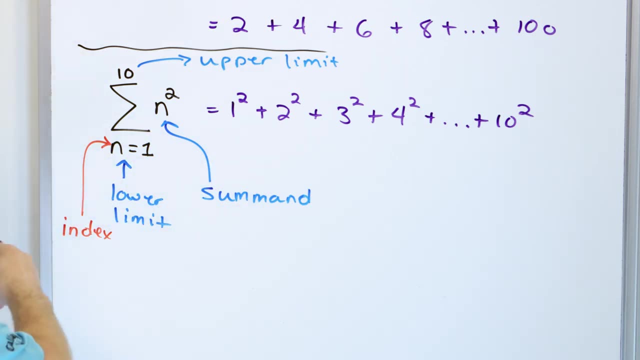 or a dummy index. The actual letter n doesn't matter, because- notice what's going on is- I'm just using n to rotate through and do this calculation. It doesn't matter what letter I use for this, It's just like a placeholder. 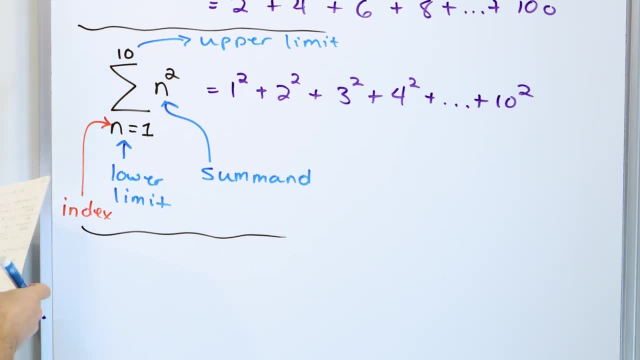 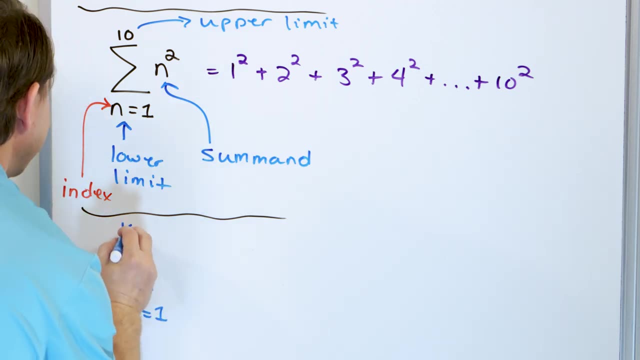 So, for instance, I can change this to the following: if I wanted to, I could make sigma right. I could say: variable k can go from one up to 10, and then what I'm gonna calculate here is gonna be k squared. 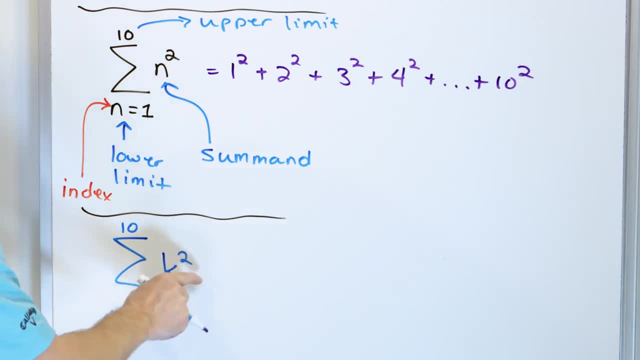 So whatever my index is, it must be involved in the calculation that's going on inside of the sum here. Otherwise it doesn't make any sense. So I have n here and n here. I have n here and n here. I have to have k and k. 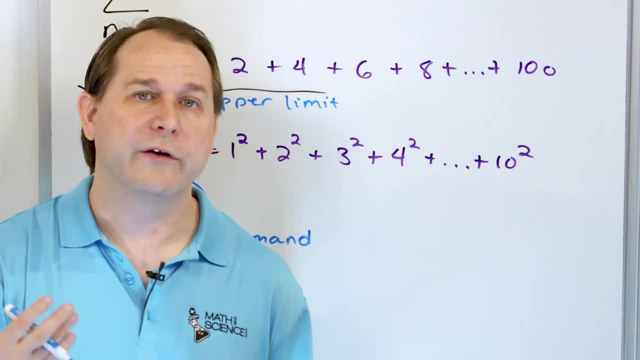 I could use different number of variables. I could use j- J is very common. Also i- j is very common. You can use any number, any letter you want, but usually n or i or j or k are usually the ones. 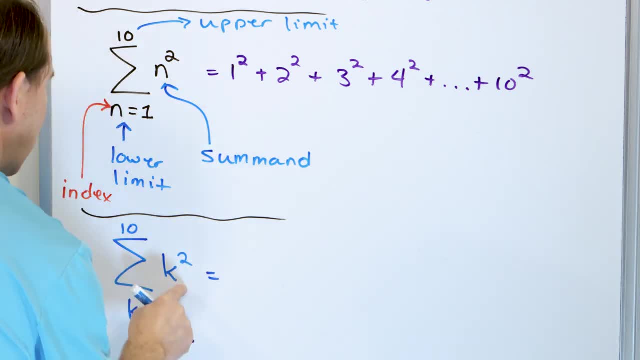 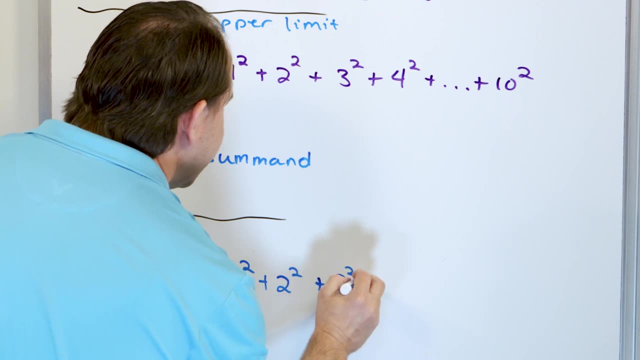 you'll see mostly in the books. But if I'm gonna use this k, I'm gonna say: k is one, k squared, one squared, then k is two, two squared, then k is three, three squared, and then plus, dot, dot, dot. 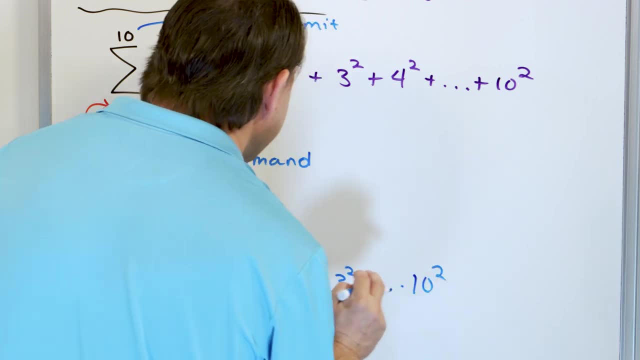 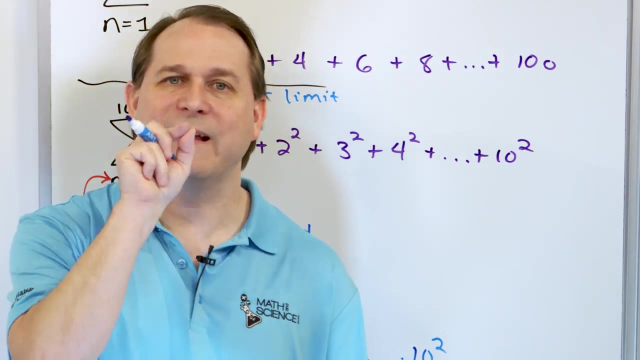 up to the maximum value of k, which is 10 squared right. So the actual variable that you use, whether it's i or j, or k or n, none of it matters. All that matters is that you use that variable to loop through the calculation. all right. 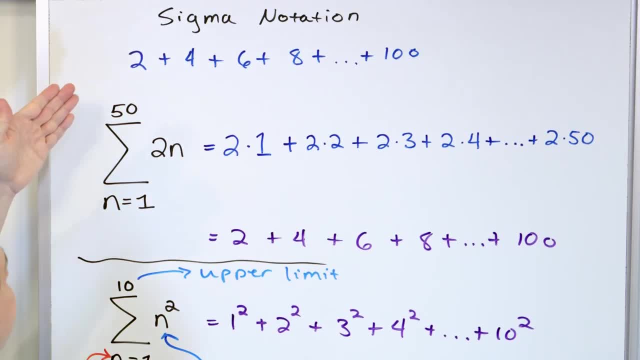 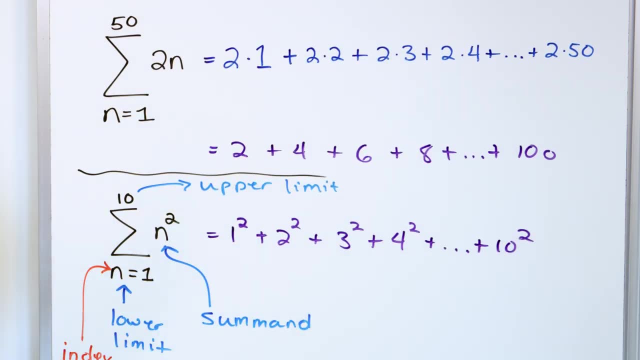 Now, so far for these examples on the board. these are what we call finite series, because it goes from one to 50. That's a finite number of terms. It goes from one to 10, one to 10.. Those are finite number of terms. 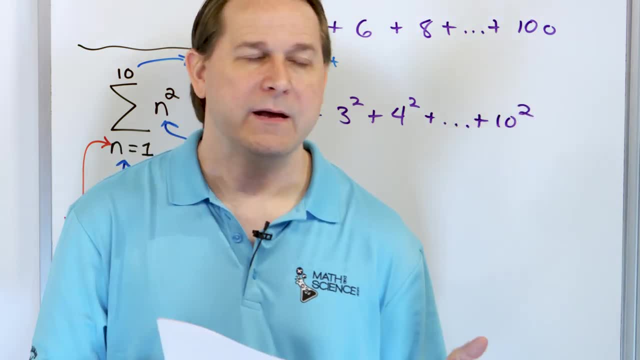 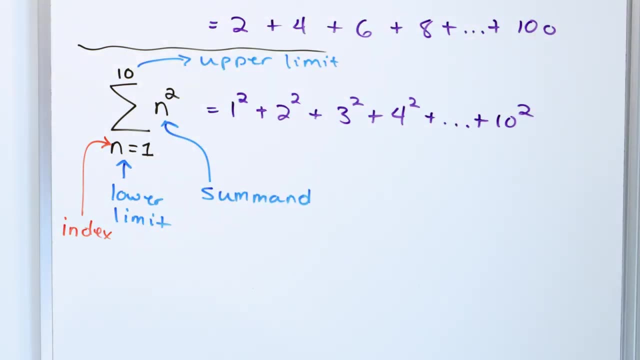 now. Right now, we're just writing down how to represent the sum, So I don't care about squaring the stuff and adding it, I just care about you knowing that this equals this. One thing that I want to make absolutely crystal clear is that this index that we're using, this N, this variable N. 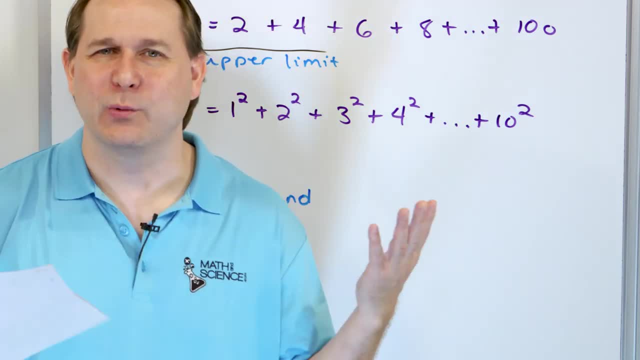 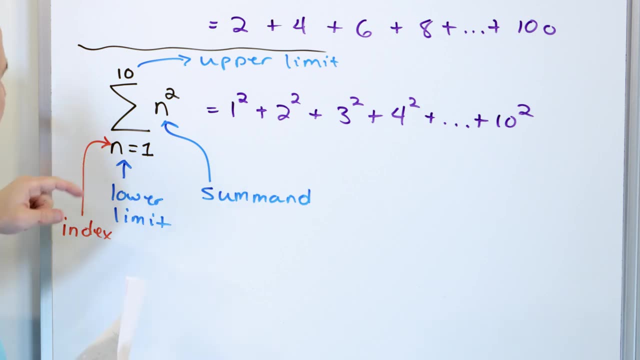 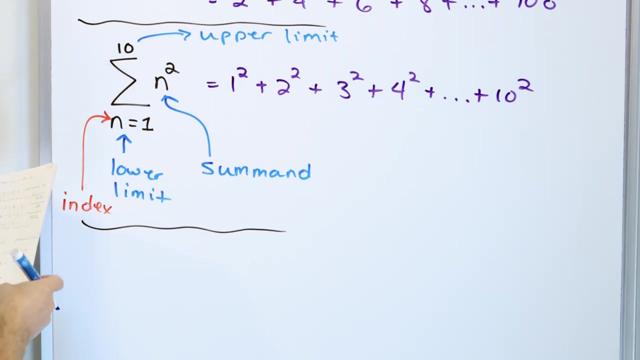 it's what we call a dummy variable or a dummy index. The actual letter N doesn't matter, because I'm just using N to rotate through and do this calculation. It doesn't matter what letter I use for this, It's just like a placeholder. So, for instance, I can change this to the following, if I 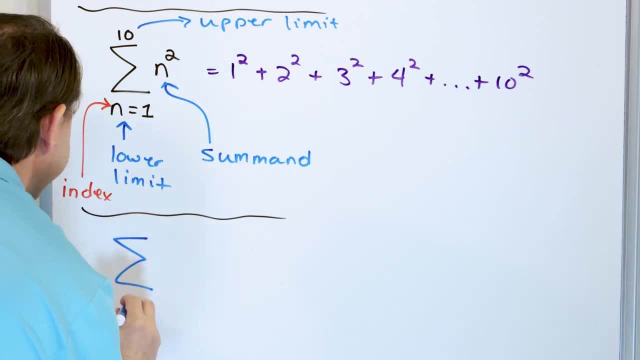 wanted to, I could make sigma right. I could say: variable K can go from 1 up to 10. And then what I'm going to calculate here is going to be K squared. So whatever my index is, it must be involved in the calculation that's going on inside of the sum here, Otherwise it doesn't make any. 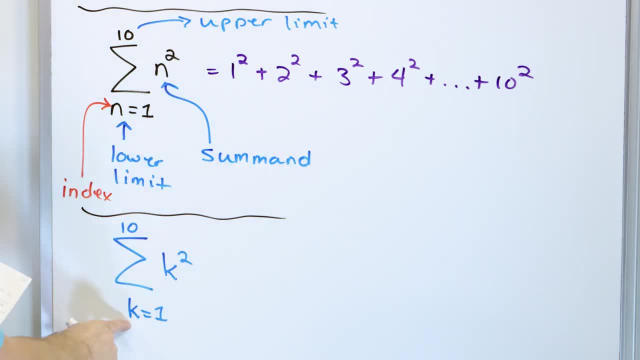 sense. So I have N here and N here, I have N here and N here. I have to have K and K. I could use different number of variables. I could use J- J is very common. Also I, I is very common, You know. 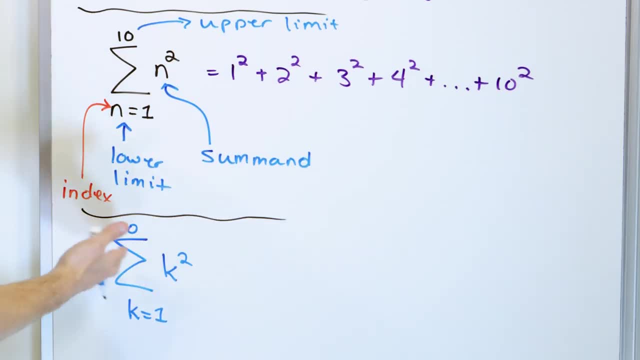 you can use any number, any letter you want, but usually N or I or J or K are usually the ones you'll see mostly in the books. But if I'm going to use this K, I'm going to say K is 1, K squared. 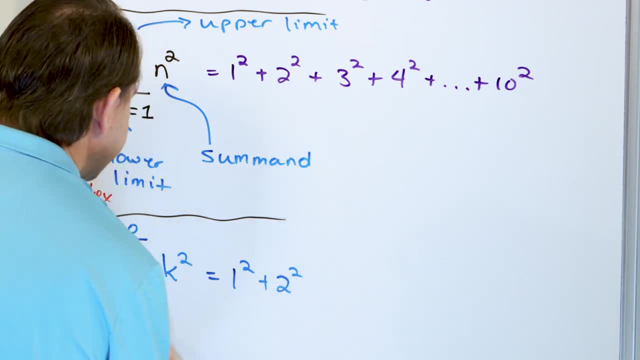 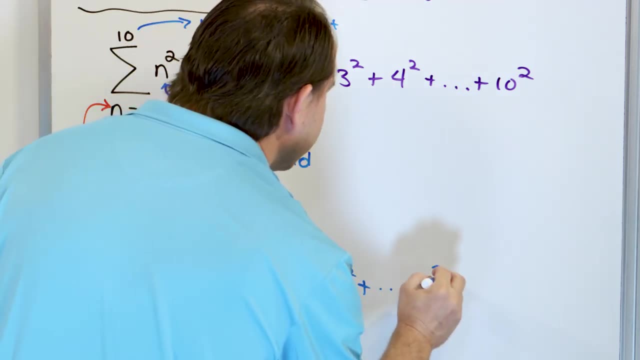 1 squared, Then K is 2, 2 squared, Then K is 3, 3 squared, And then plus, dot, dot, dot up to the maximum value of K, which is 10 squared right. The actual variable that you use, whether it's I or J, or K or N, none of it matters All that. 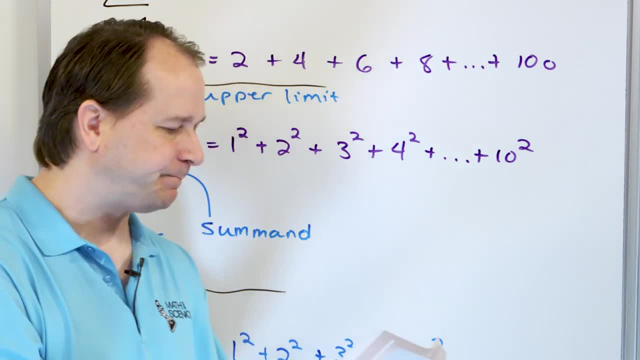 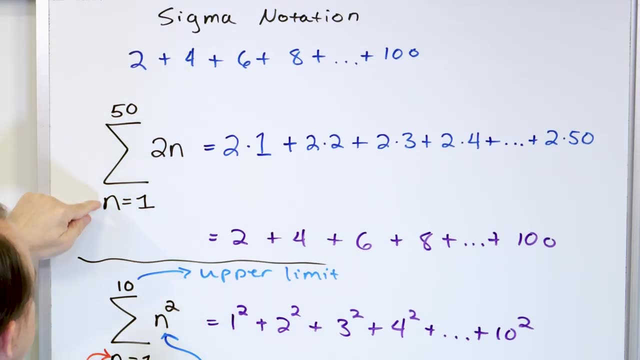 matters is that you use that variable to loop through the calculation. All right Now, so far for these examples on the board. these are what we call finite series, because it goes from 1 to 50. That's a finite number of terms. It goes from 1 to 10, 1 to 10.. Those are finite number of terms. 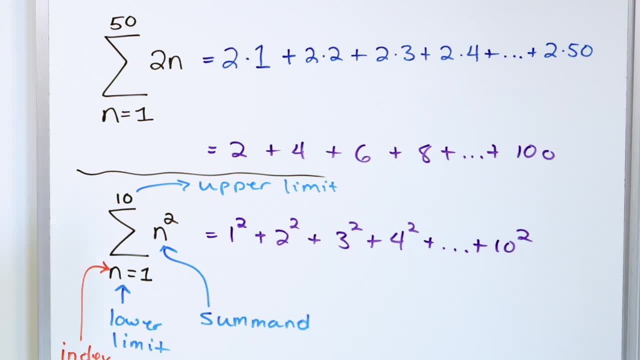 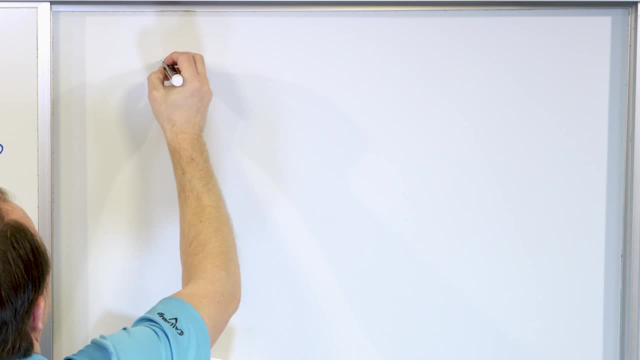 But we already talked about that. we can have infinite series which has an infinite number of terms, And so how do we write down something Like this? So an infinite series might look something like this: Write down my little sigma here, from K is equal to 1.. Now what do you think is going to happen? The upper limit is not going. 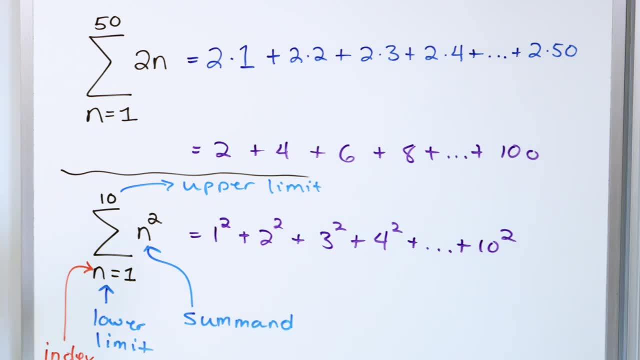 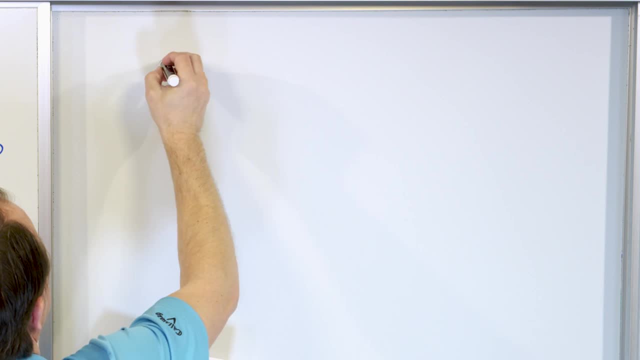 But we already talked about that. we can have infinite series, which has an infinite number of terms, And so how do we write down something like this? So an infinite series might look something like this: Write down my little sigma here: From k is equal to one. 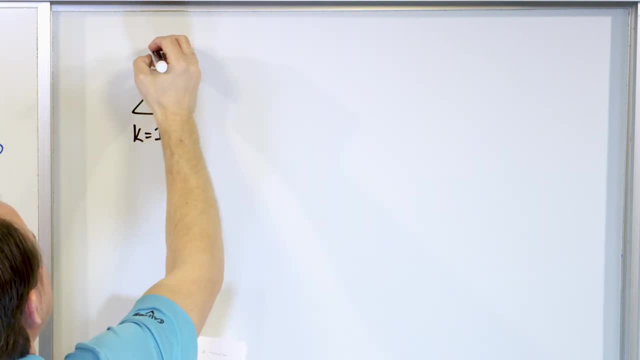 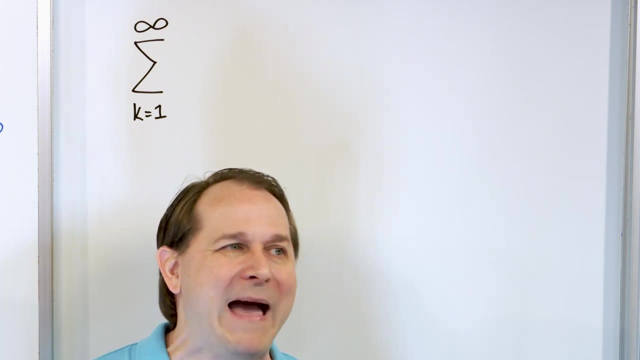 Now what do you think's gonna happen? The upper limit is not gonna be a number, The upper limit is going to be an infinity. So that's where you put the infinity symbol at the top, because the upper limit never ends The maximum term. it never comes. 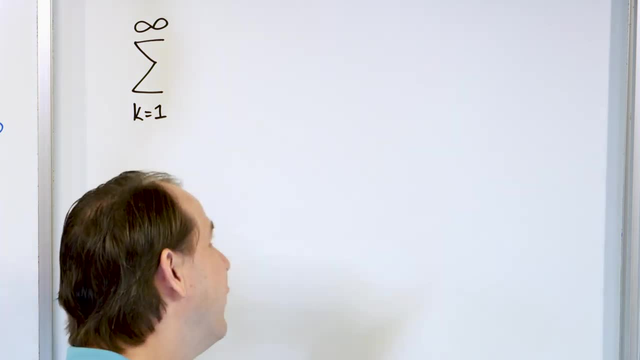 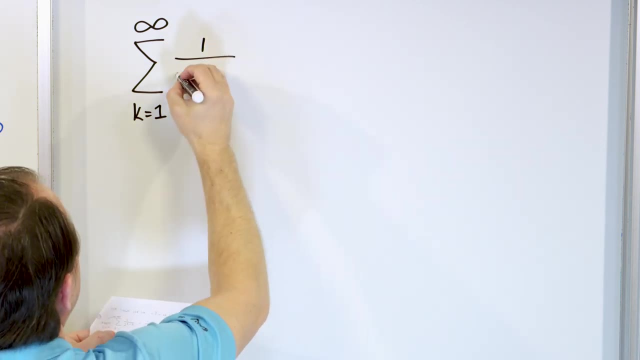 It's always out there. Infinity never actually happens. It's still going and going and going. So if I have k is equal to one to infinity, then maybe my terms might be something like, just as an example: two to the power of k minus one right. 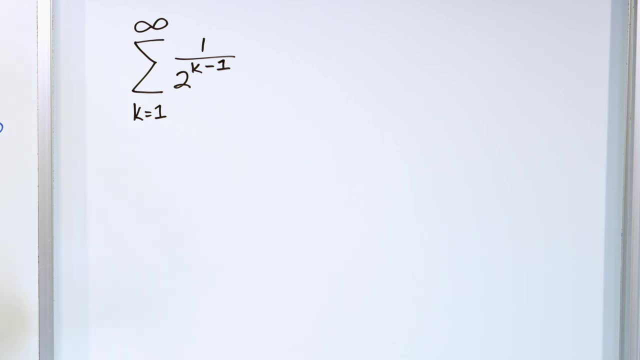 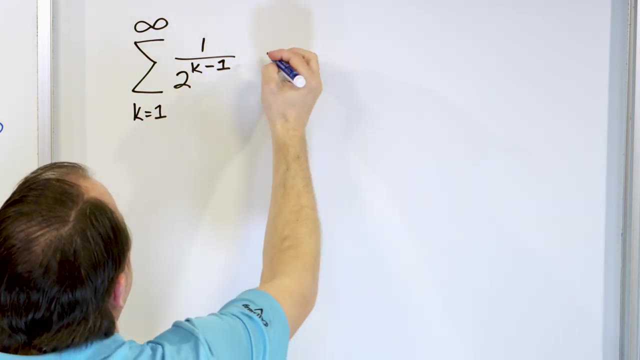 That looks really complicated, right, But what you have to do is kind of get rid of that in your mind because it isn't really complicated. All you're doing is starting at k is one and you're putting it in here. So what would these terms look like? 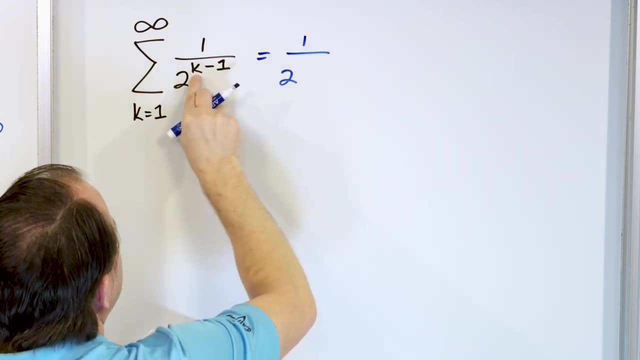 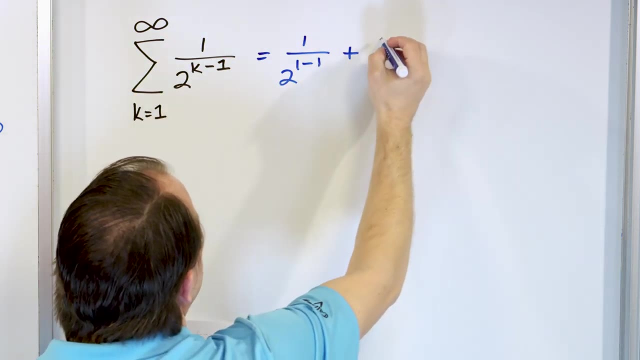 When k is one, it'd be one over two to the power of k is one. Let's write it as one minus one And we're gonna add to that looping around when k is two, Then it will be two to the power of two minus one. 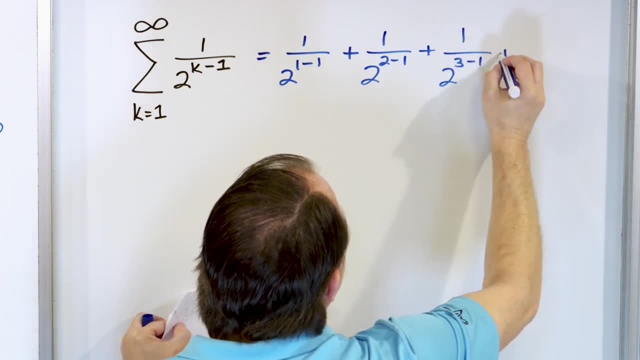 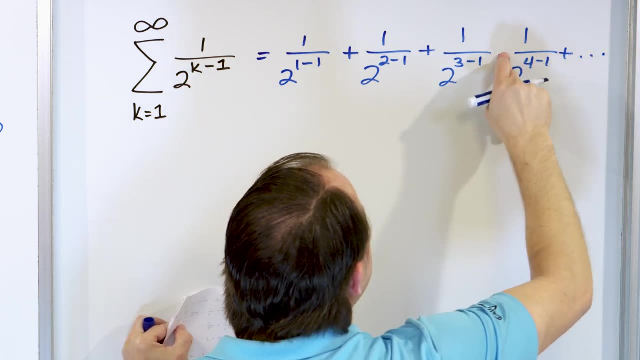 Then it'll be one over to the power of three minus one, One over two to the power of four minus one plus. and here's where you go: dot, dot, dot, because it never, ever ends. So what you have is k is one, then k is two. 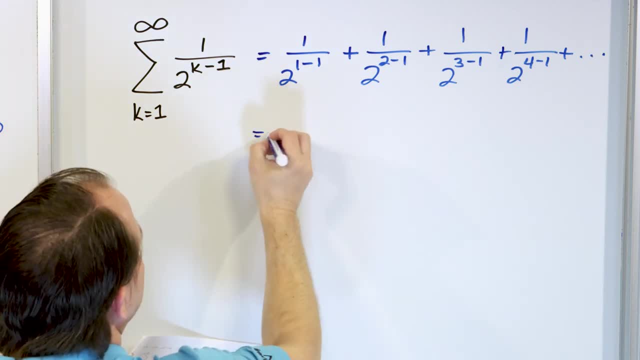 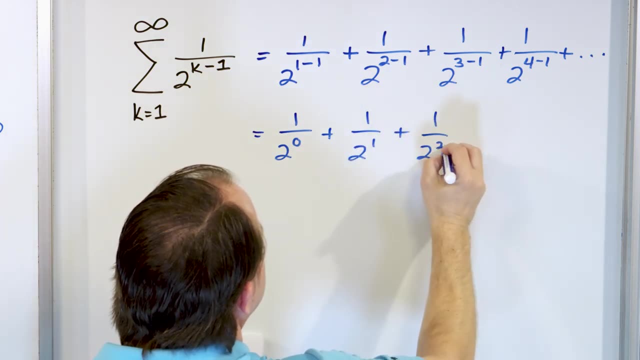 then k is three, then k is four, and it never ends. So what does this thing really look like? On the bottom, it's gonna be one over two to the zero, One over two to the one, One over two to the two. 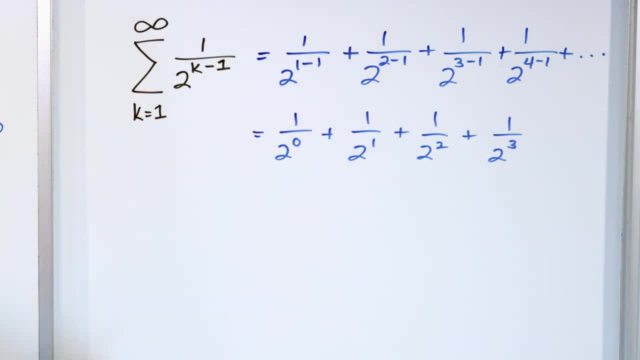 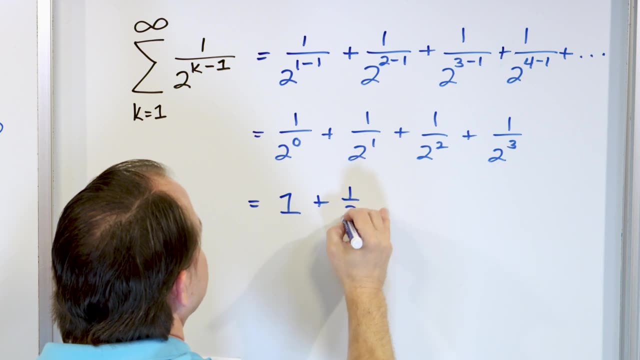 One over two to the three. All I'm doing is doing the subtraction here, And what does this come out to? Two to the zero is one. One over one is one. This is gonna be one half. This one over two squared is gonna be one. fourth: 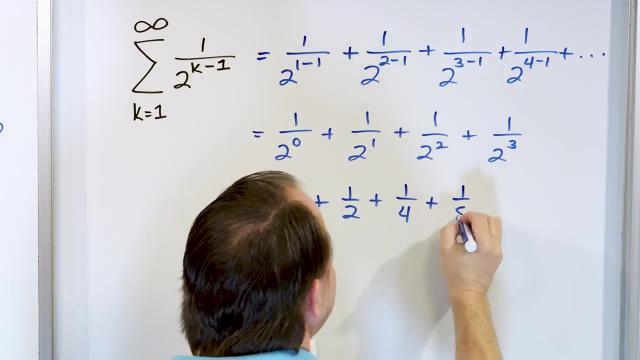 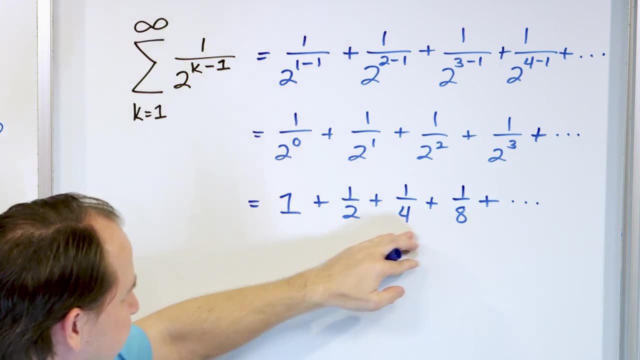 This is gonna be one over two cubed, but that's eight, so it's gonna be one over eight plus dot dot dot- I forgot right here- plus dot dot dot as well, So this series here can be represented. 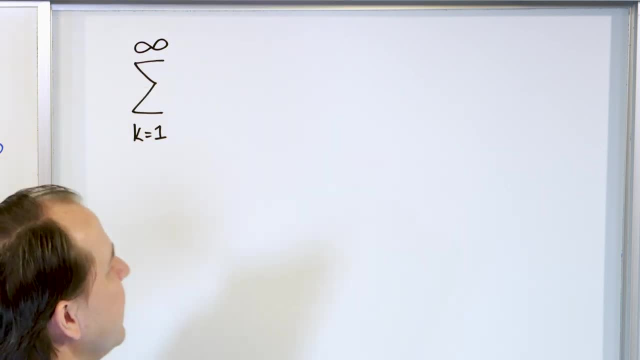 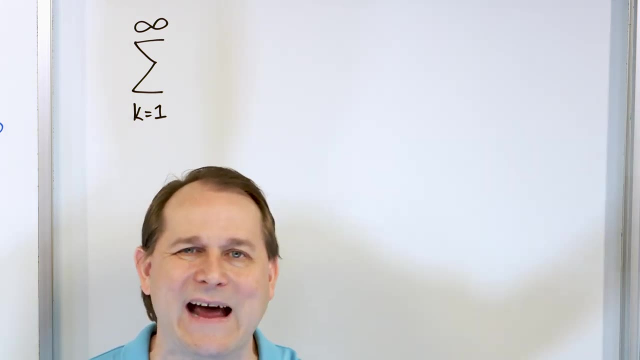 to be a number. The upper limit is going to be an infinity. So that's where you put the infinity symbol at the top, because the upper limit never ends The maximum term. it never comes, It's always out there. Infinity never actually happens. It's still going and going and going. 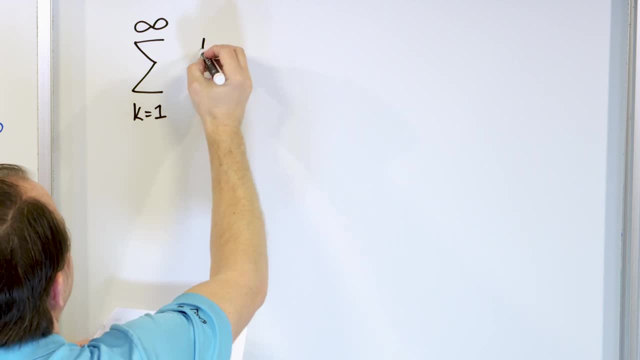 So if I have K is equal to 1 to infinity, then maybe my terms might be something like this: So I'm going to write down my little sigma here And I'm going to write down my simple formula in thegreen box as well. right now We're going to do the simple formula: we. 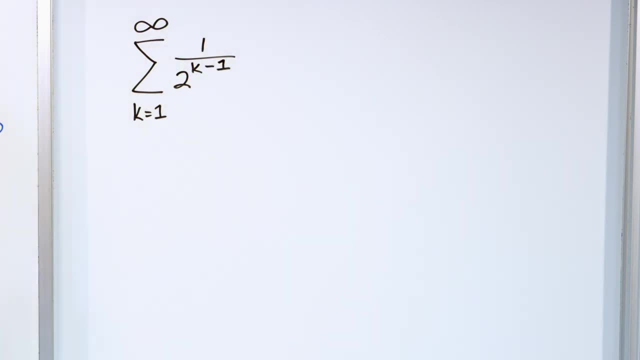 thought about, And we actually have you write downatti here. first, This is 1 at k and point 1 is 0. And then we're going to double our numbers over 1.. Let's do some math here And we're going to write down that are constant terms. 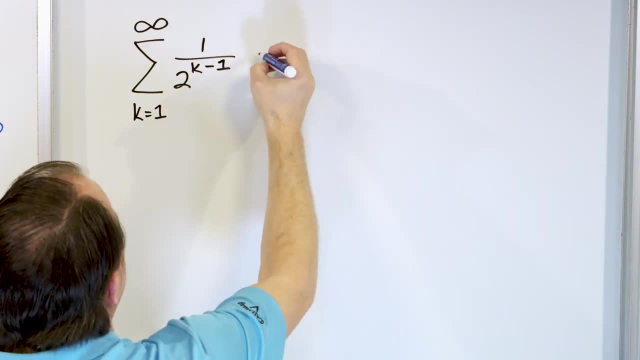 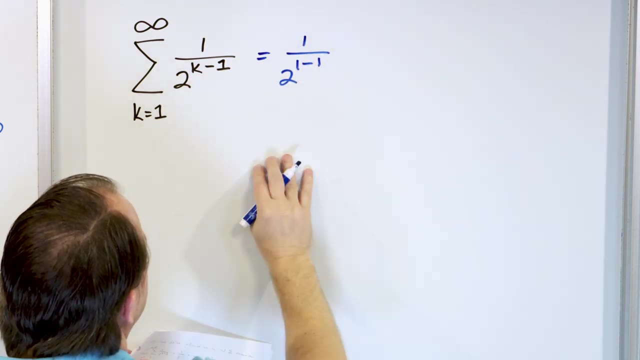 or is that 1? 3 by 3.. 0 plus 2 is 1.. 1 minus 1 plus 1 is 2.. So what? what? what are we going to write down here? We're going to write down that you have K is equal to 1 and K is spun down. 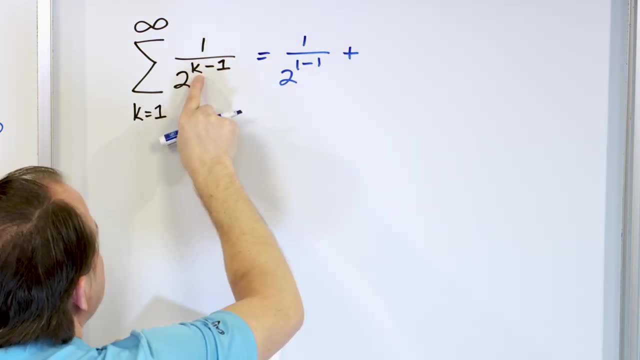 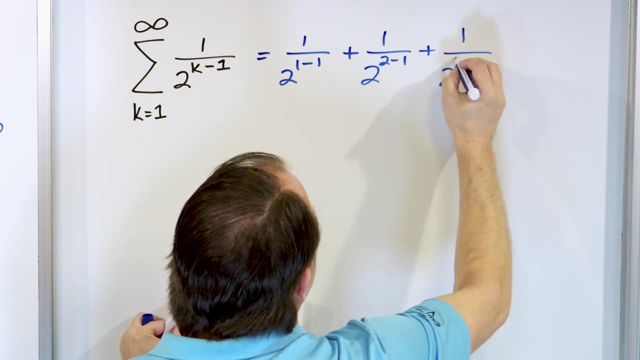 All right crying, I'm click function every any. Look at this rick, это 1, we write it down in thewe без1.. one, Then it'll be one over to the power of three minus one, Then one over two to the power of four. 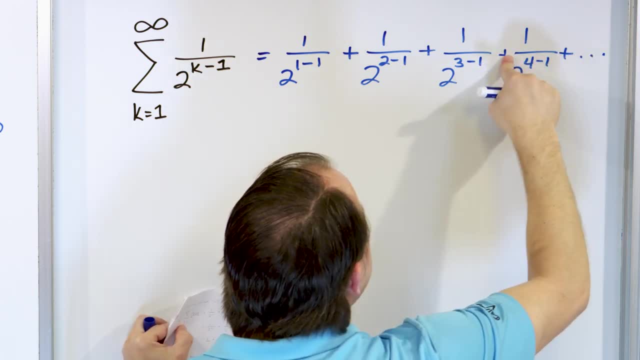 minus one plus. and here's where you go: dot, dot, dot, because it never, ever ends. So what you have is: k is one, then k is two, then k is three, then k is four, and it never ends. So what does this? 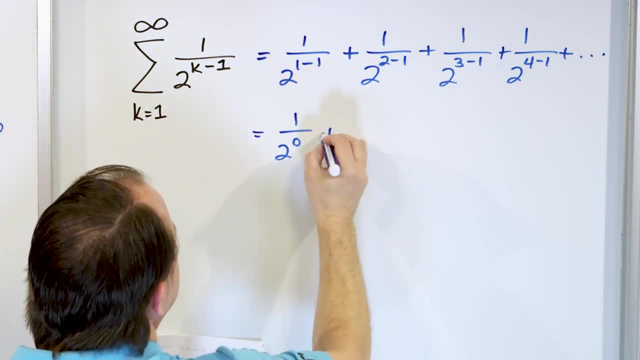 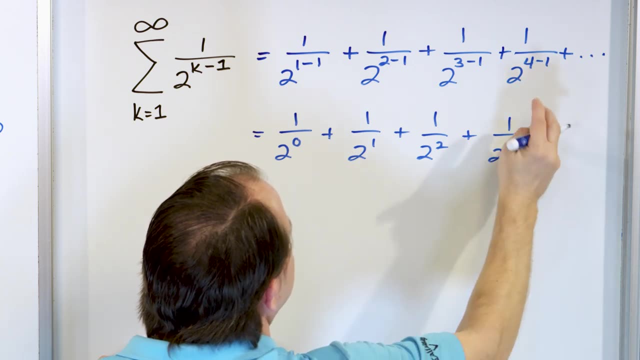 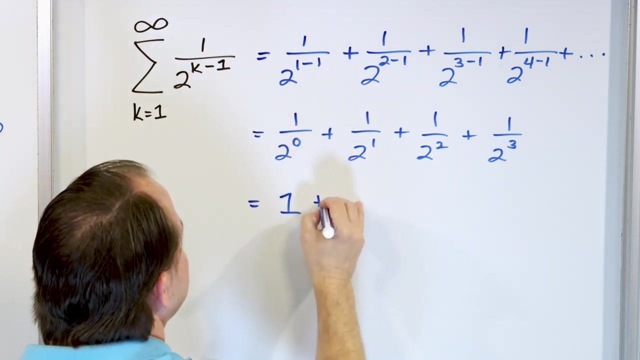 thing really look like On the bottom. it's going to be one over two to the zero, One over two to the one, One over two to the two, One over two to the three. All I'm doing is doing the subtraction here, And what does this come out to? Two to the zero is one. One over one is one. This is going. 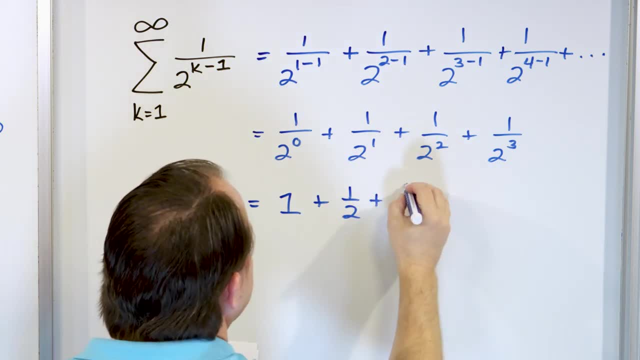 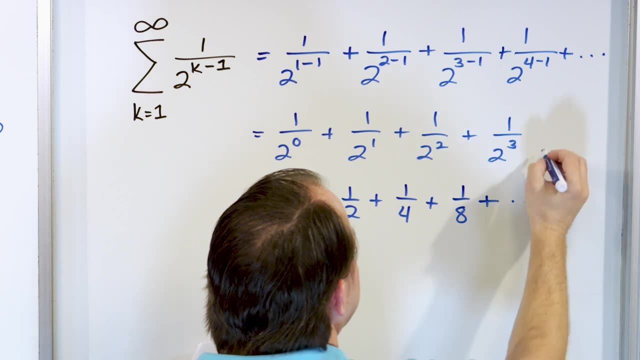 to be one half. This one over two squared is going to be one. fourth, This is going to be one over two cubed, but that's eight. so it's going to be one over eight, plus dot dot dot. I forgot. 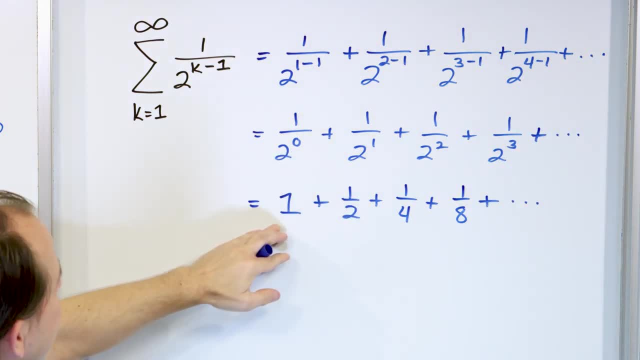 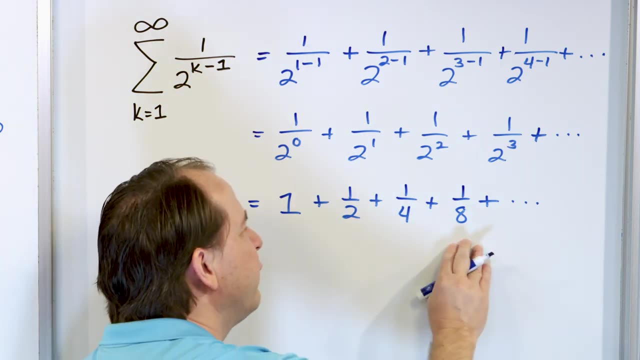 right here, plus dot, dot dot as well. So this series here can be represented as this sigma notation. It's an infinite series, which means you can see the pattern: one over two, one over four, one over eight, you know, one over 16, and so on Going. 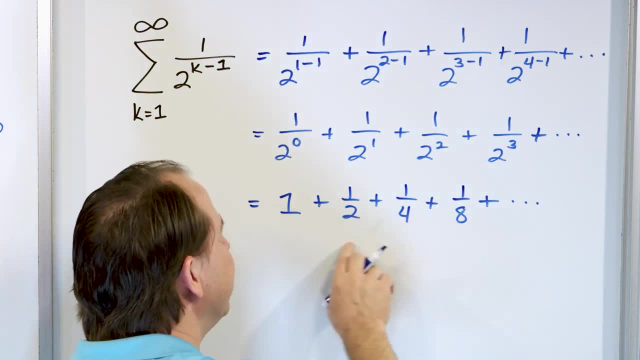 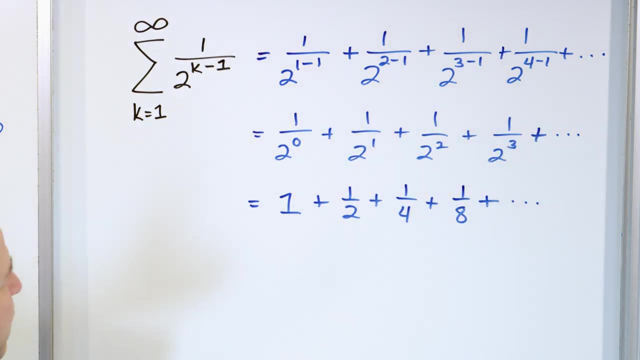 as this sigma notation. It's an infinite series, which means you can see the pattern: one over two, one over four, one over eight, you know one over 16 and so on going down there. Basically, what's going on is: I'm multiplying by one half. 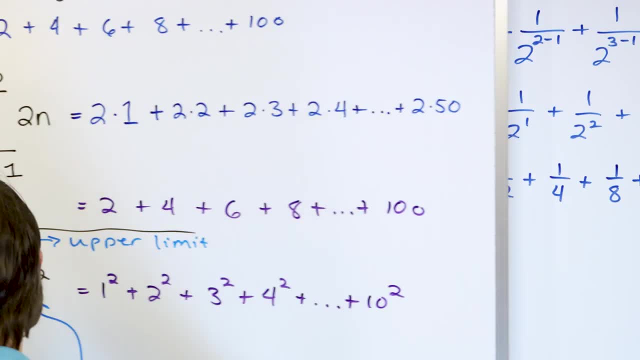 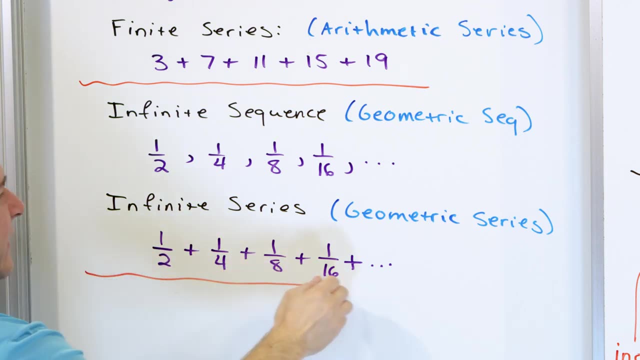 every time to get the remaining terms, which is kind of like what I started with here. This is an infinite series here, where I just started with one half, So one half, one, fourth, one, eighth, one, 16.. This is the same series, except the first term is not one half. 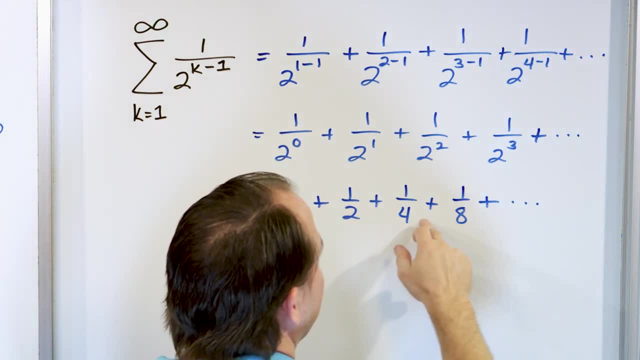 The first term is one, So one, then one half, then one fourth, then one eighth, then one 16th, then one 32nd, and so on. It's gonna keep going. So, instead of writing all these things out, 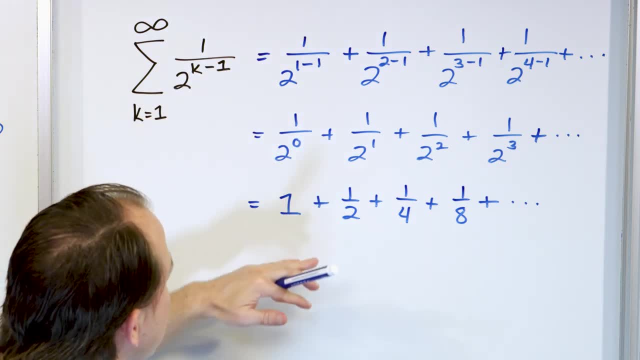 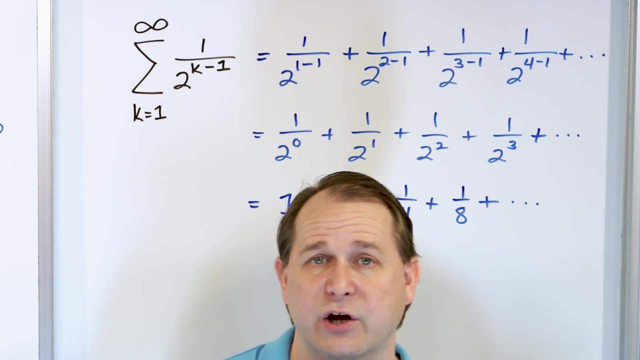 I just write the sigma notation Now. There's two things to skills here. First skill is looking at the sigma notation and writing down the series. That's what we're focusing on now. Later on we're gonna reverse it, where I will give you the series. 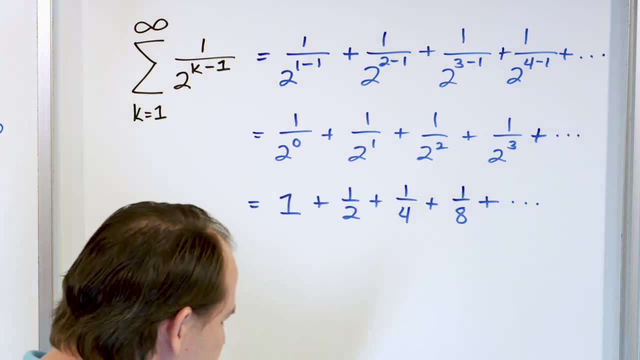 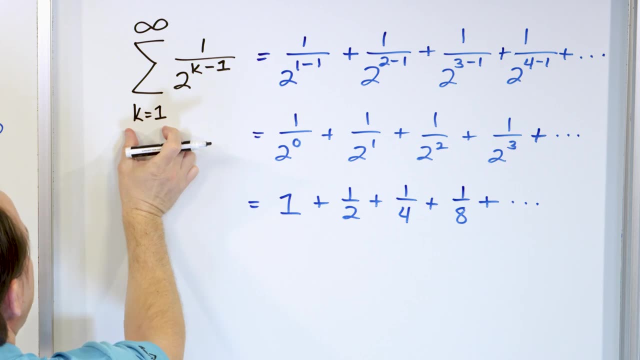 and you have to come up with the sigma notation right Now, before we get there. I want to make. one other thing that's important for you to know is that here I have k going from one to infinity, and here are the terms, the sumand that yields this thing: 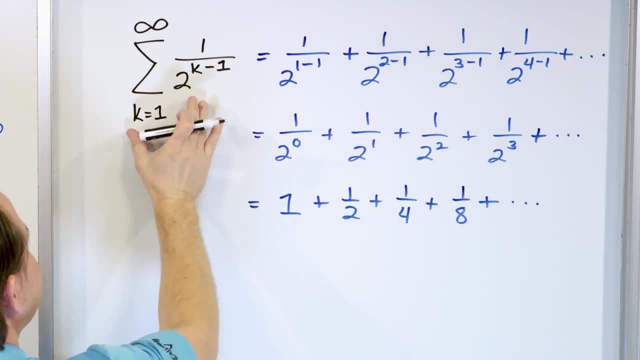 There's more than one way usually to write the summation notation. to give you the same series, For instance, let me go down here and drop down below. Just explore this with me a little bit. What if, instead of this, what if we get the summation? 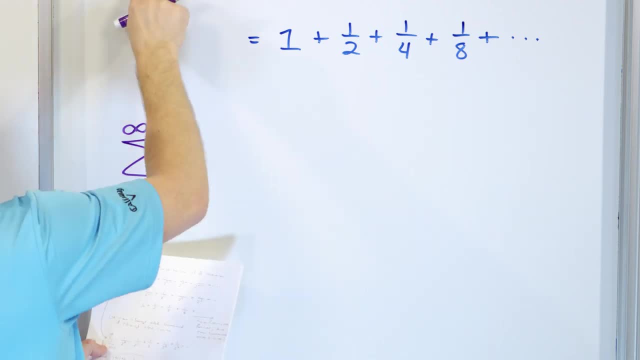 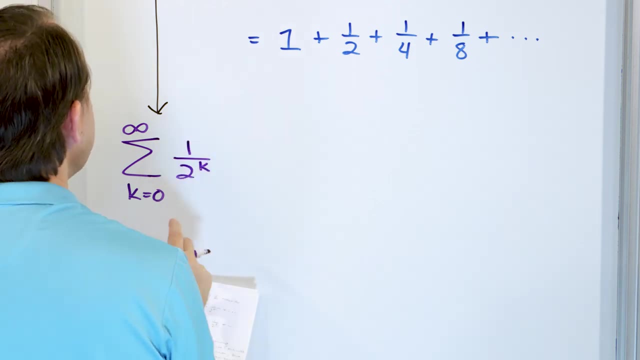 of k is zero up to infinity. Notice I'm not going from one to infinity. I change the limits and I go from zero to infinity, of one over two to the k. Notice that this is really similar to this. What's going on here is this: is in the exponent. 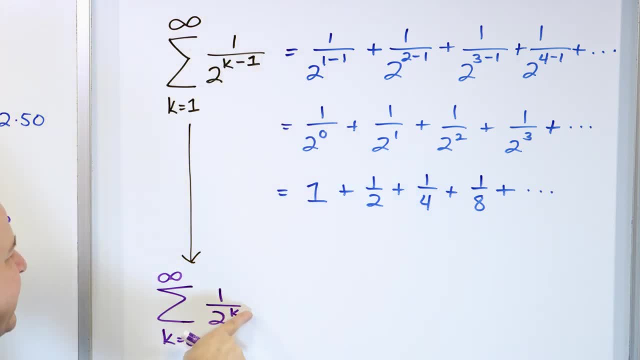 I have a k minus one, but I change the calculation so it doesn't say k minus one. What happens is I add one in the exponent up here and because I've advanced one in the exponent, I compensate for that by subtracting one in the index. 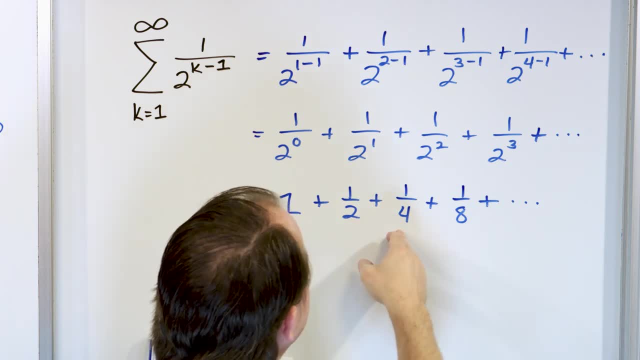 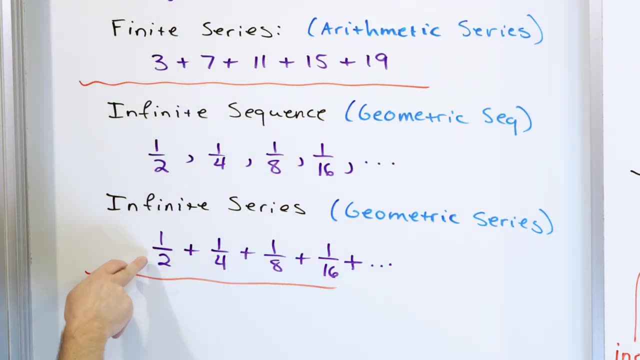 down there. basically, what's going on is I'm multiplying by one half every time to get the remaining terms, which is kind of like what I started with here. This is an infinite series here, where I just started with one half. so one half, one fourth, one, eight, one, sixteen. This is 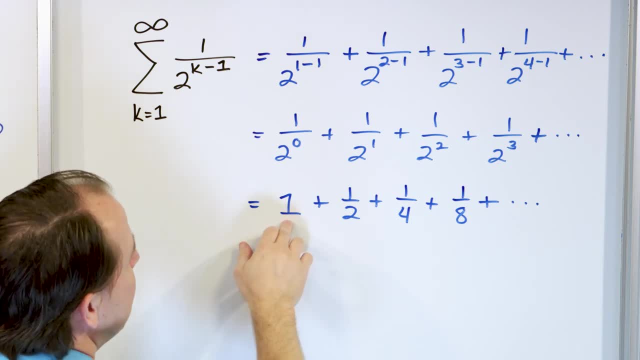 the same series, except the first term is not one half. The first term is one. So one, then one half, then one fourth, then one eighth, then one sixteenth, then one thirty-second, and so on. It's going to keep going. So instead of writing all these things out, I just write. 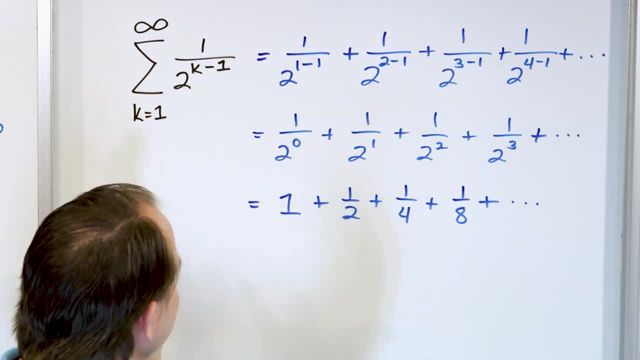 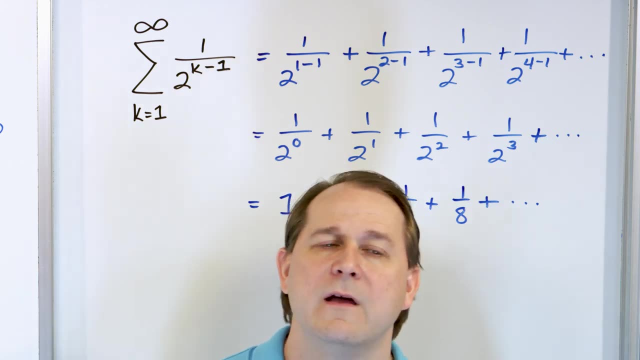 the sigma notation. Now there's two things to skills here. First skill is looking at the sigma notation and writing down the series. That's what we're focusing on now. Later on we're going to reverse it, where I will give you the series and you have to come up with the sigma notation. 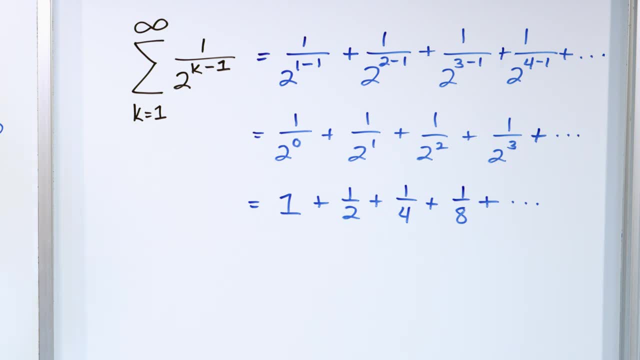 right Now, before we get there, I want to make. one other thing that's important for you to know is that here I have k going from one to infinity, and here are the terms, the sumand that yields this thing. There's more than one way usually to write the summation. 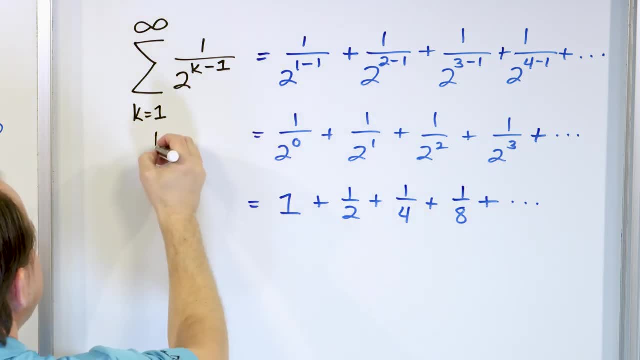 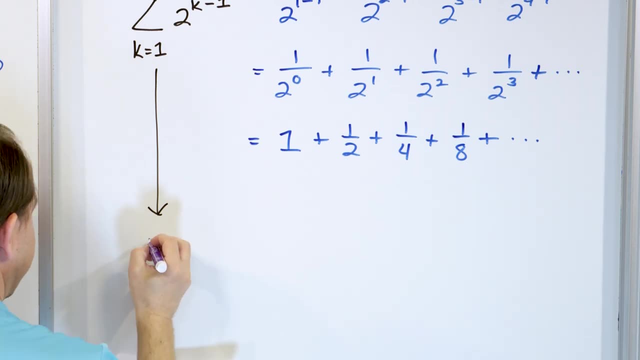 notation to give you the same series, For instance. let me go down here and drop down below. Just explore this with me a little bit. What if, instead of this, what if we get the summation of k is zero up to infinity? Notice, I'm not going from one to infinity. I. 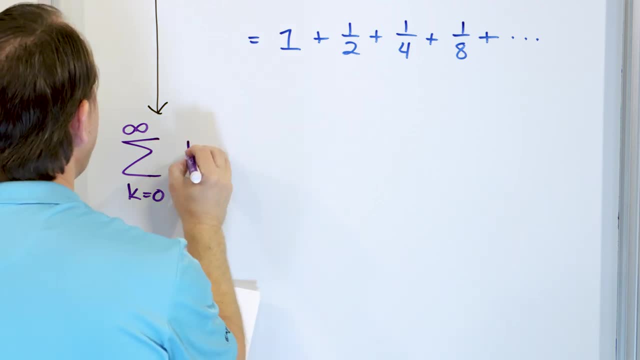 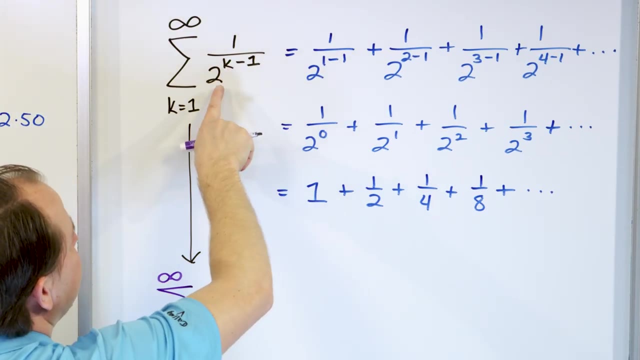 changed the line. I'm going from one to infinity, I'm going from one to infinity, I'm going from limits and I go from zero to infinity, of one over two to the k. Notice that this is really similar to this. What's going on here is this: is in the exponent, I have a k minus one, but I changed the. 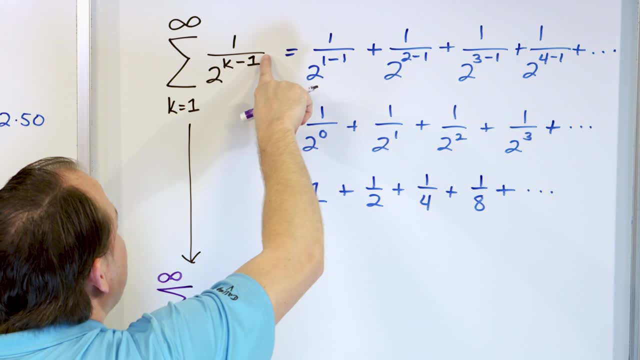 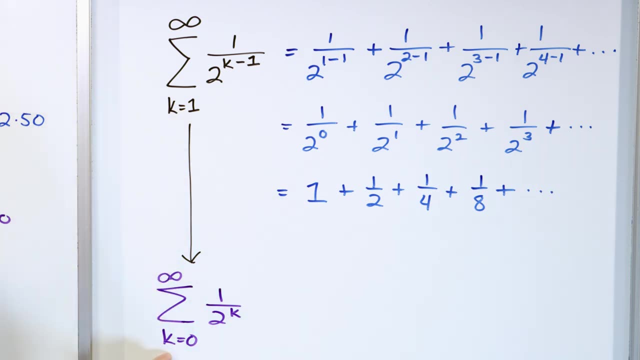 calculation so it doesn't say k minus one. What happens is I add one in the exponent up here and because I've advanced one in the exponent I compensate for that by subtracting one in the index. If I mess around with the sumand, with the calculation there and change the exponent or 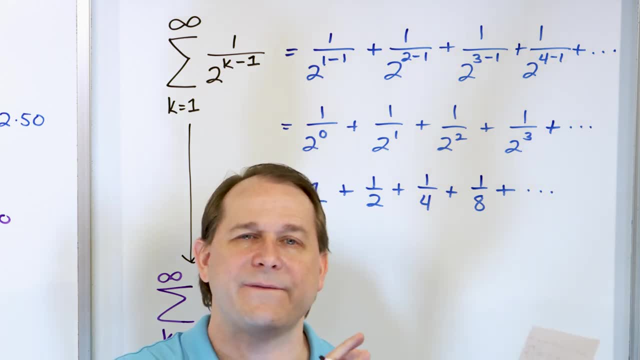 change something related to the index, the variable, then if I change anything regarding that, I also need to go adjust my limits of summation to make sure I get the same term. If we go through this calculation, we can see that this will be one over two to the power of zero. 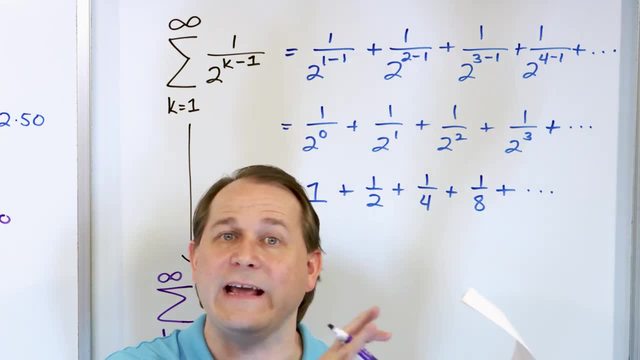 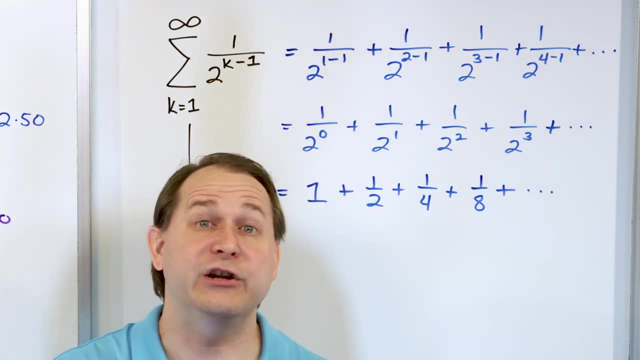 So if I mess around with the sumand, with the calculation there, and change the exponent or change something related to the index, the variable, then if I change anything regarding that, I also need to go adjust my limits of summation to make sure I get the same term. 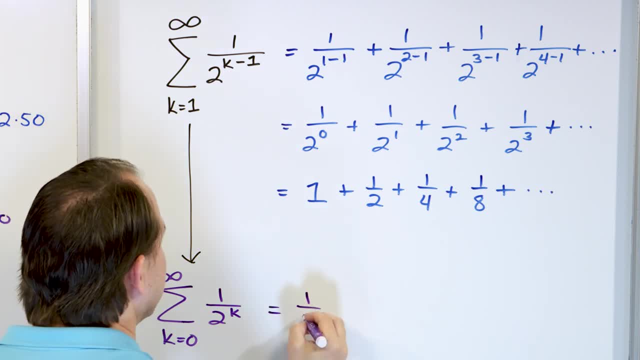 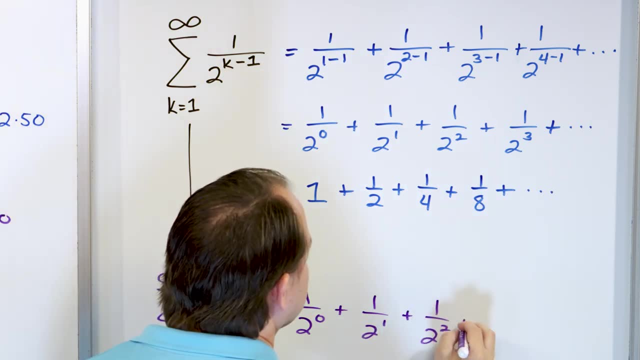 So if we go through this calculation, we can see that this will be one over two to the power of zero, one over two to the power of one when k becomes one. one over two, squared one over two, third plus dot, dot, dot. 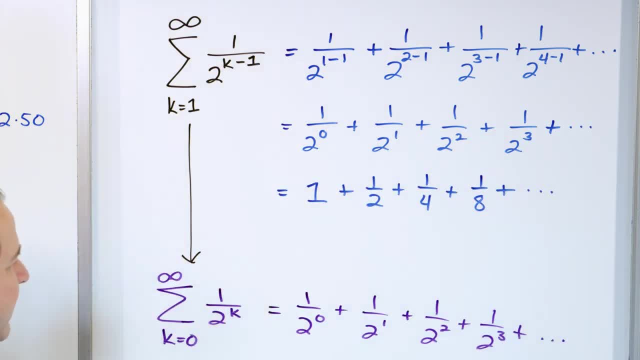 And you can see, these terms are the same terms as these, which are the same terms as these, So this series can be represented by this, Or this series could also be represented by this, And I could, if I wanted to change this even further. 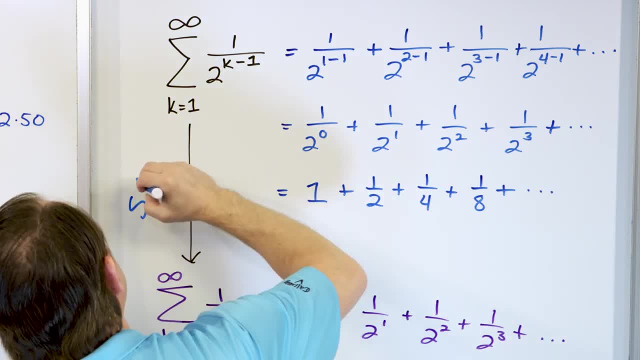 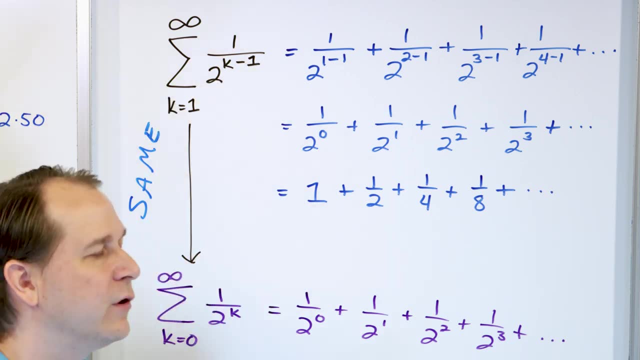 and then change the limits even more drastically, But these are the same. In other words, it's not really more correct to say this one is the right answer or this one's the right answer, As long as those two sums the summations. 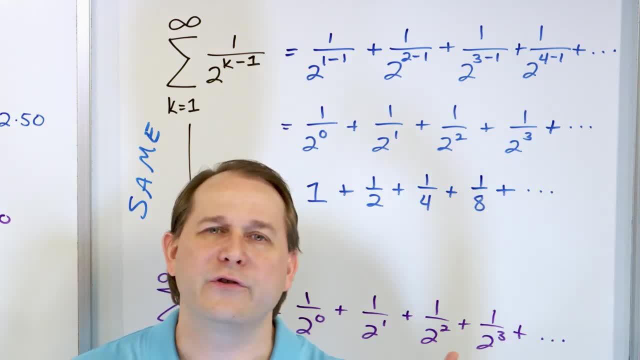 the summation convention. as long as it's giving you the same terms, then they're both equally correct. They represent the same things, But still, sometimes when we do problems, one of them looks a little simpler than others. You know, like five tenths and one half. 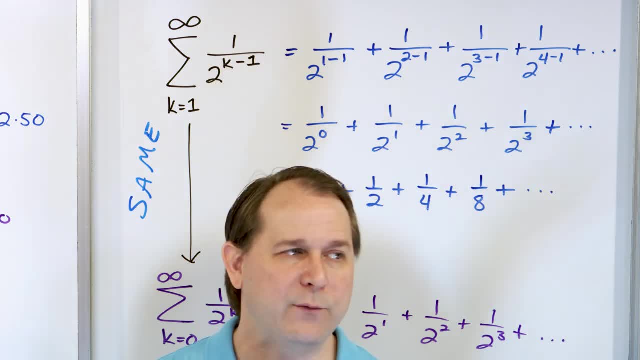 they both represent half the pizza, right Five tenths and one half. they represent the same thing, But we usually say one half is simpler, So that's what we usually like. This one here it looks simpler, So usually we'll probably write something like this down: 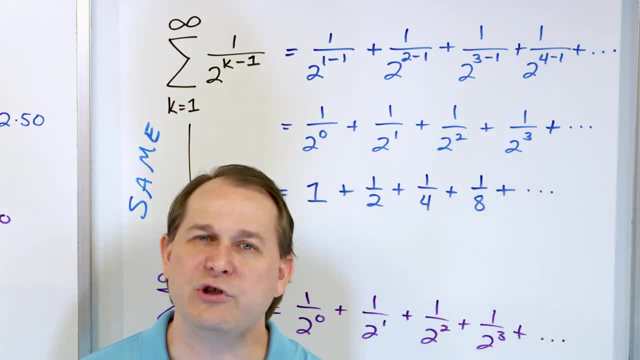 although this gives exactly the same terms. So just keep that in mind When you get your answers to these problems and you look at my answers or you look at answers in your textbook or whatever, as long as it could be a little different. 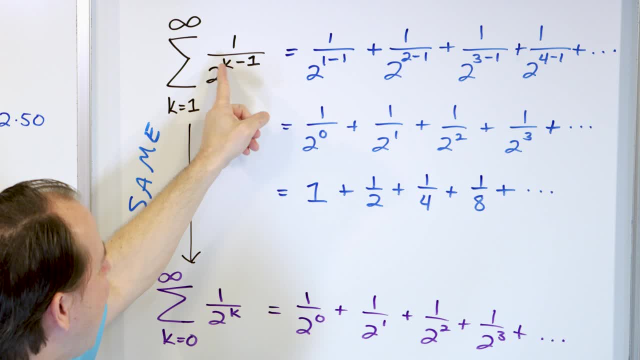 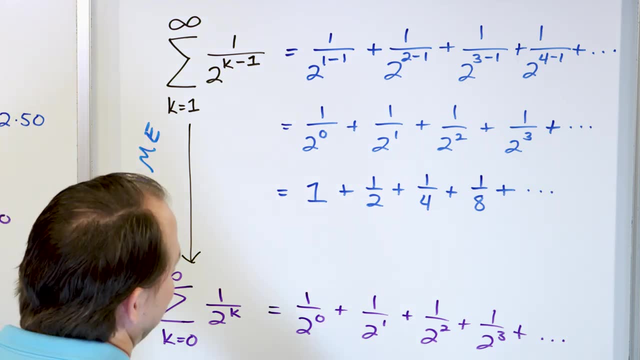 If you adjust the exponent here, if you adjust anything related to k- adding or subtracting- and you compensate by messing around with the limits of summation, then it can still be correct. is all I'm trying to tell you. All right, so finally, 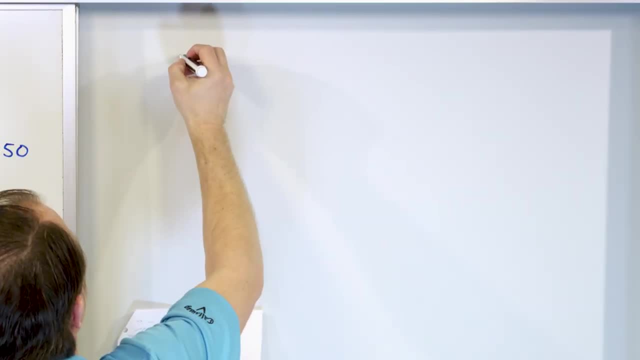 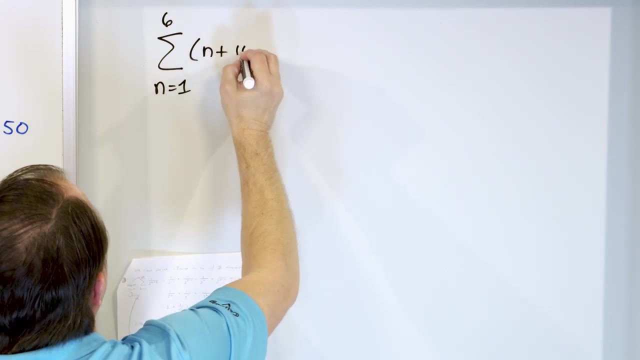 let's do a couple of quick problems. None of these are hard, but let's get some examples. What if I do? the limits from n is equal to one, up to six of n plus 10?. What I want you to do is I want you to write it in expanded form. 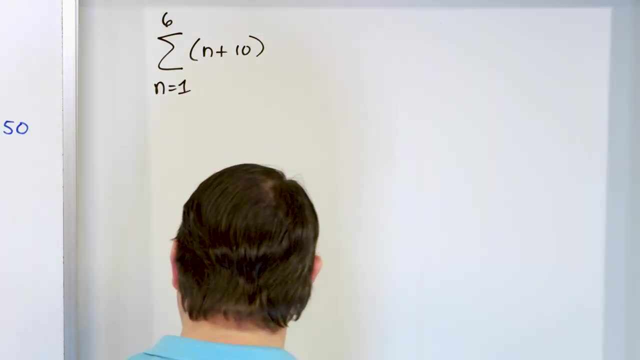 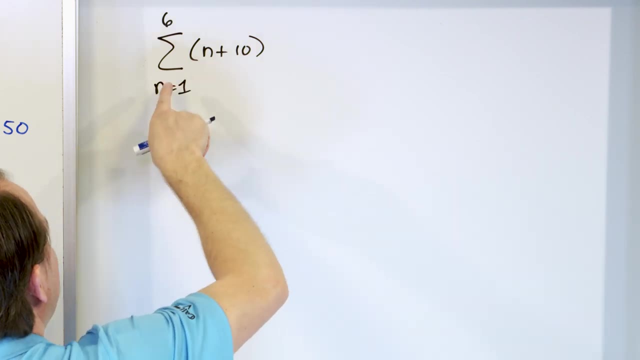 I want you to take the sum, the summation notation, and I want to expand this into the full-blown sum. What do we do? We just go through as a loop, like a little computer program. When n is one, n goes into one here. 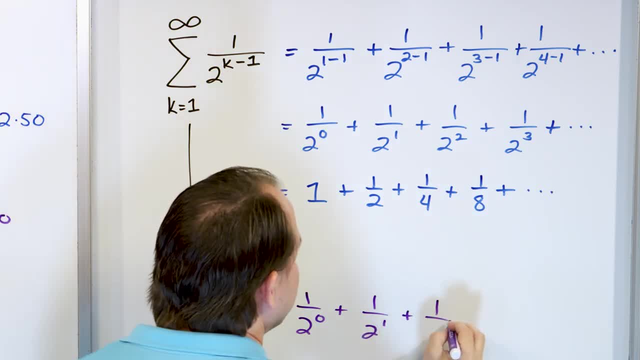 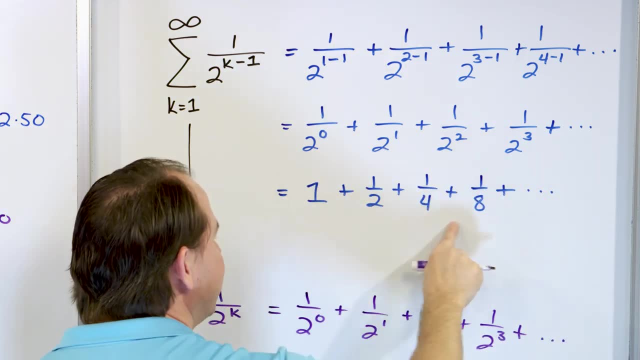 one over two to the power of one. when k becomes one, one over two, squared one over two, third plus dot dot dot. You can see these terms are the same terms as these, which are the same terms as these. This series can be written in this way: If I change anything regarding that, I also need 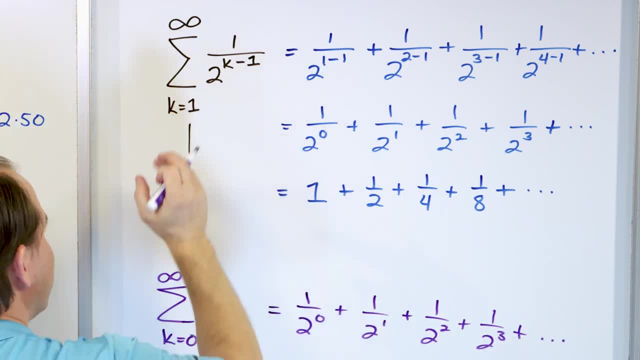 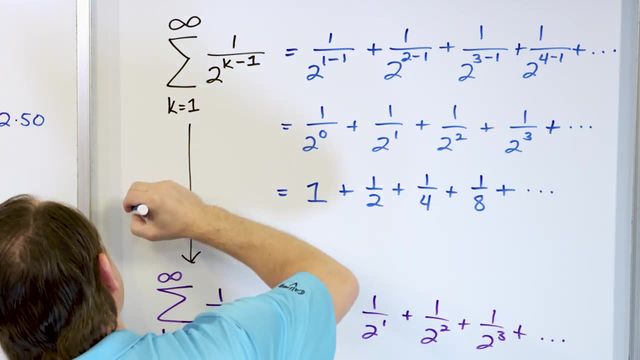 to be represented by this, or this series could also be represented by this, And I could, if I wanted to, change this even further and then change the limits even more drastically, but these are the same. In other words, it's not really more correct to say this one is the right answer, or? 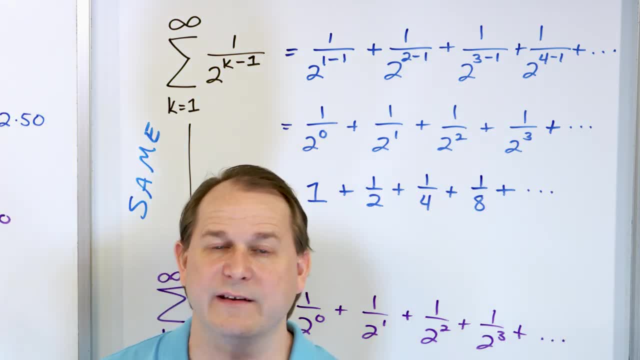 this one's the right answer. As long as those two sums, the summations, the summation convention, as long as it's giving you the same terms, then they're both equally correct. They represent the same things, But still, sometimes when we do problems, one of them looks a little simpler. 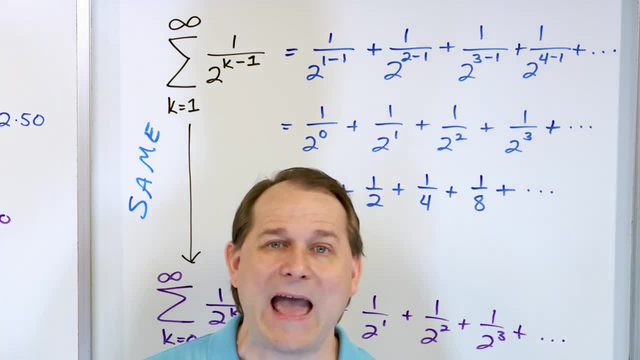 you know, like five tenths and one half. They both represent half the pizza, right? Five tenths and one half. They represent the same thing, but we usually say one half is simpler. So that's what we usually like. This one here is, it looks simpler. So usually we'll probably write something. 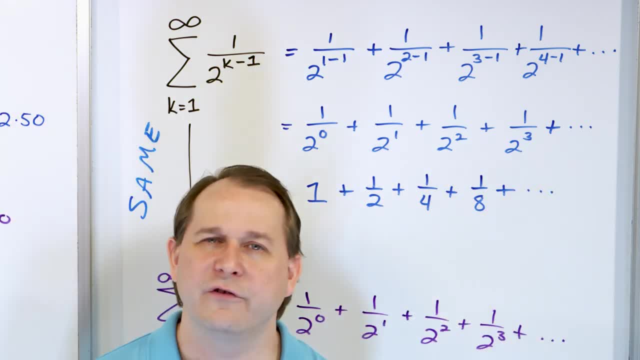 like this down, although this gives exactly the same terms. So just keep that in mind when you get your answers to these problems and you look at my answers or you look at answers in your textbook or whatever, as long as it could be a little different If you adjust the exponent here. 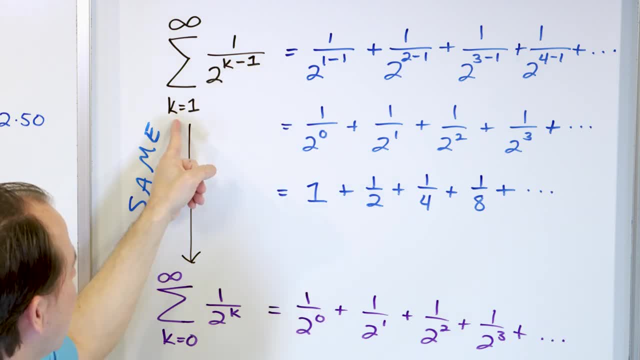 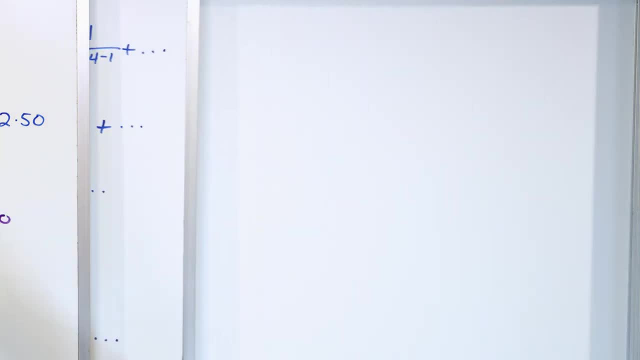 if you adjust anything related to k- adding or subtracting- and you compensate by messing around with the limits of summation, then it can still be correct. is all I'm trying to tell you. All right, so finally, let's do a couple of quick problems. None of these are hard, but let's get some. 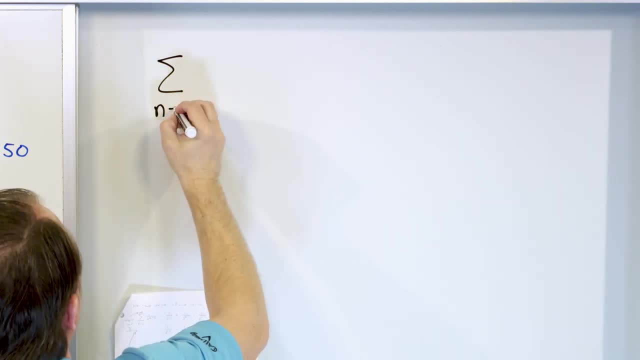 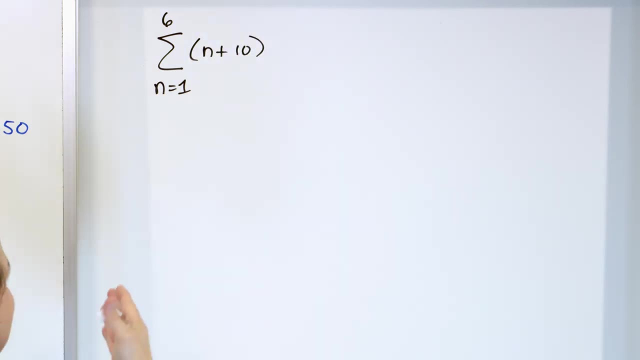 examples. What if I do? the limits from n is equal to 1 up to 6 of n plus 10?. What I want you to do is I want you to write it in expanded form. I want you to take the sum, the summation notation. 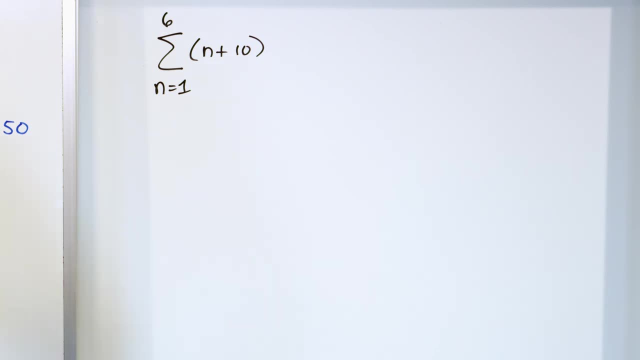 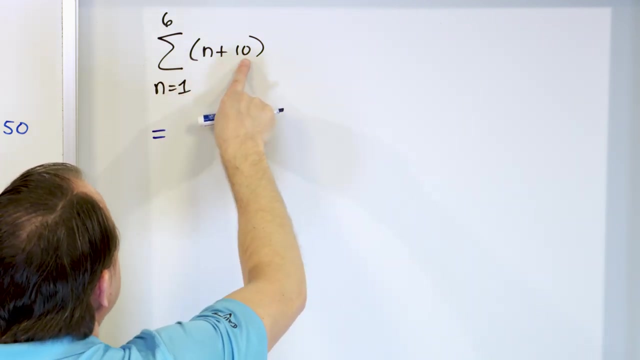 and I want to expand this into the full-blown sum. What do we do? We just go through as a loop, like a little computer program. When n is 1, n goes into 1 here, 1 plus 10. Now don't do too. 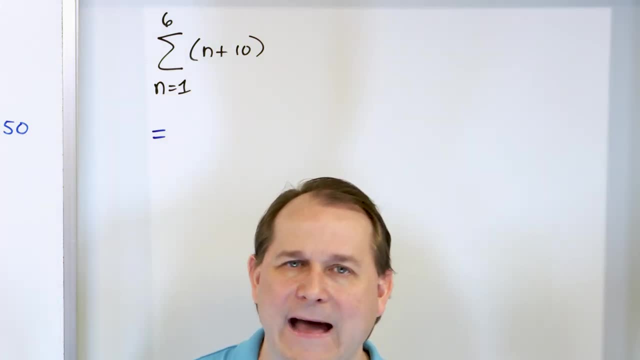 many things at once. Don't try to add 1 plus 10 in this step. I don't want that. I want you to just put the number in there, because if you do too many things at once, you will make a mistake when the 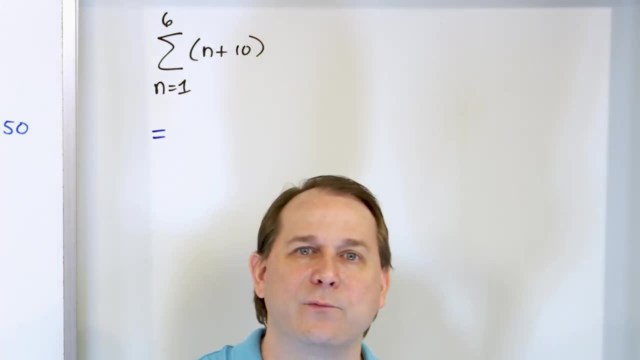 one plus 10.. Now, don't do too many things at once. Don't try to add one plus 10 in this step. I don't want that. I want you to just put the number in there, because if you do too many things at once, 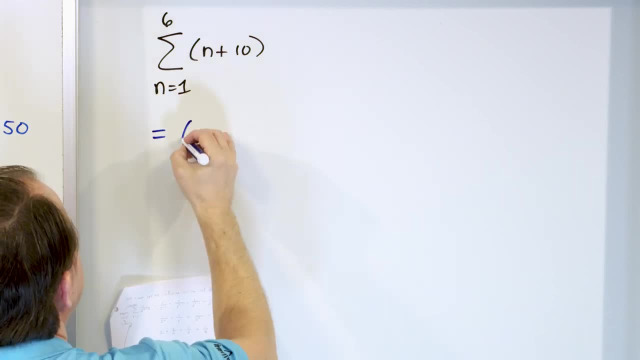 you will make a mistake when the problems get harder. What I want you to write down for the first term is n being one, one plus 10.. This is the first term when I put it in here. I'm gonna add to that, because it's a summation- n being two. 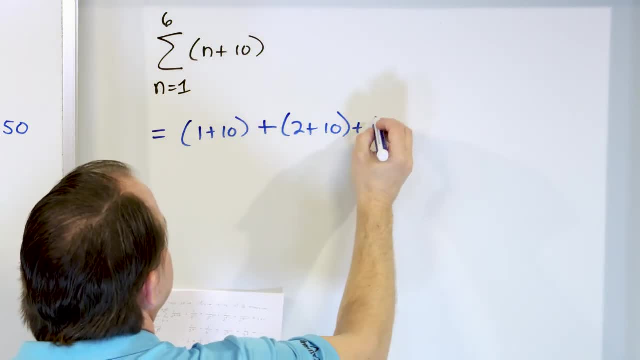 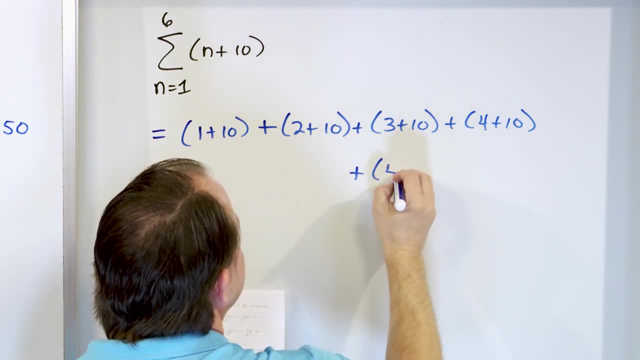 Then it'll be two plus 10, right, Then it'll be three plus 10.. Then it'll be four plus 10.. I'll go down here. then it'll be five plus 10.. Then it'll be six plus 10,. 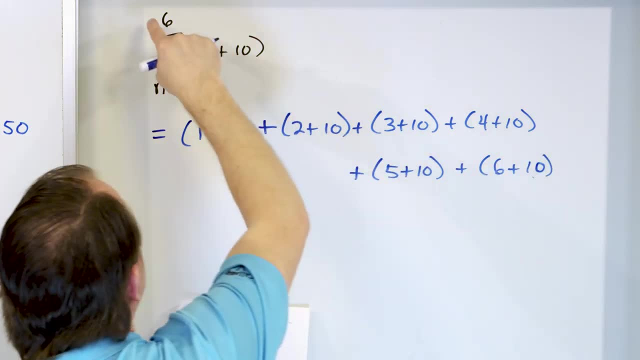 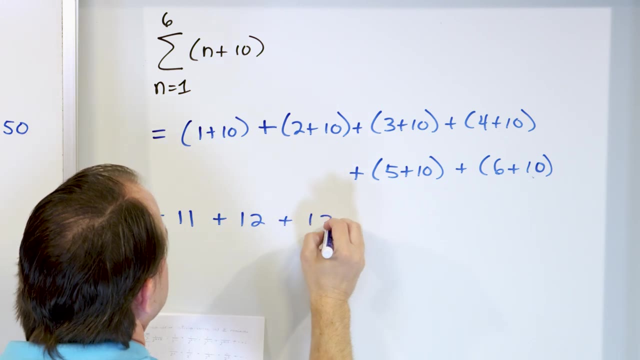 because then, finally, n has gotten to its maximum value of six. Now, in the next step, then you go and add. You say: this is 11,, this is 12,, 13,, 14,, 15,, 16.. Now I know that you can all grab a calculator. 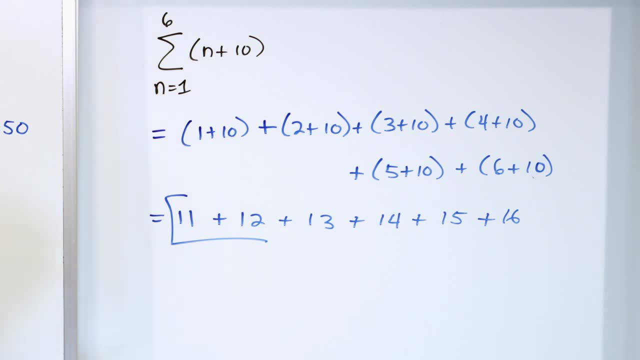 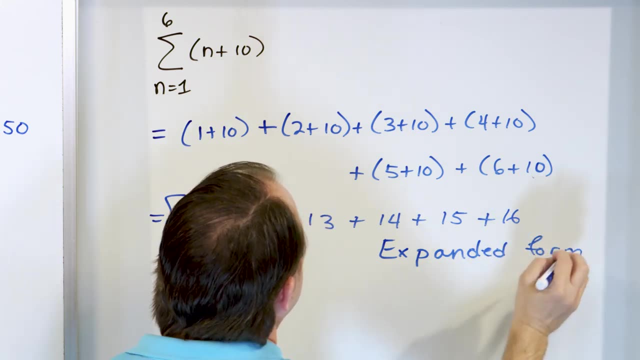 and add these up. I don't want you to do that. What I want you to do is circle this, because this is what we call expanded form. All I care about is that you can translate what the summation is telling you, the sigma: 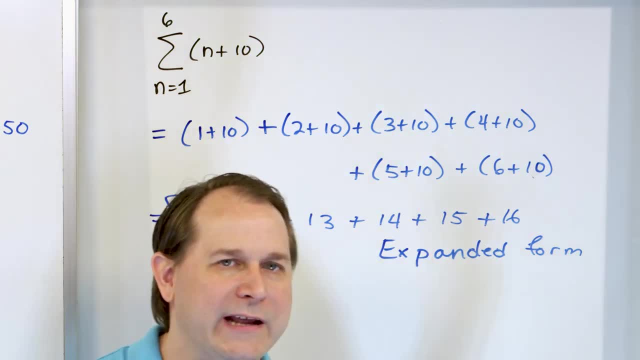 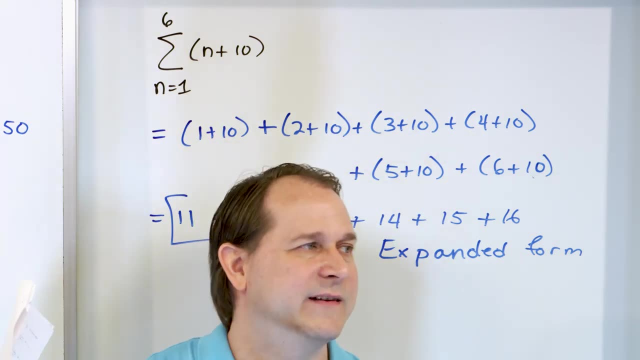 and write down the sum. That's all I care about. I know that you can all grab the calculator and add those together. That isn't helpful to me. What I want to know is if you can take the sum, the summation, the sigma and blow out the terms. 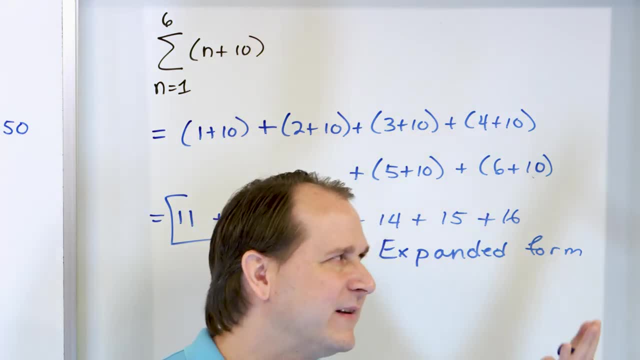 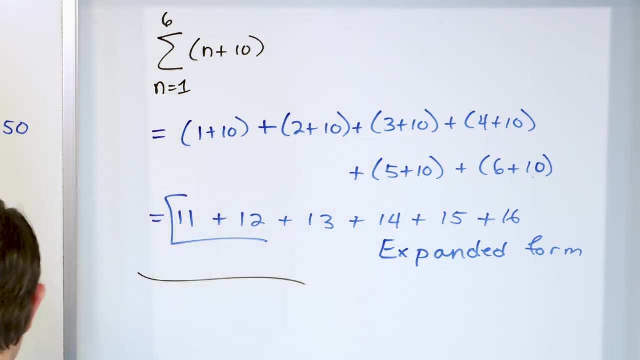 Later on in a few lessons, we'll talk about how to add these things together. I mean, obviously you can add these, but what happens if there's 1,000 terms? How do I add them up without spending my whole life doing it? 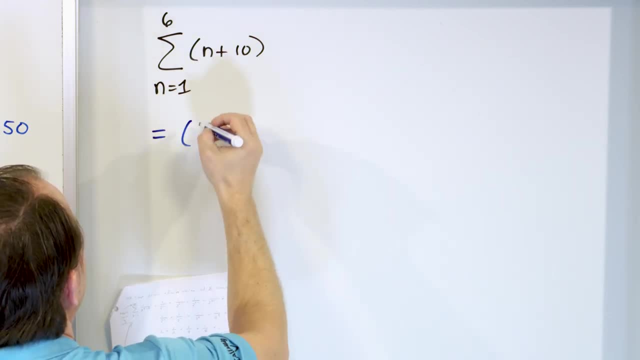 problems get harder. What I want you to write down for the first term is n being 1,, 1 plus 10.. This is the first term when I put it in here. I want you to do that because it's a summation, n being 2.. Then it'll be 2 plus 10.. Then it'll 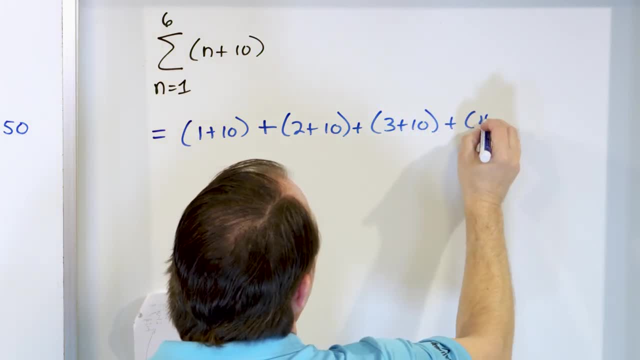 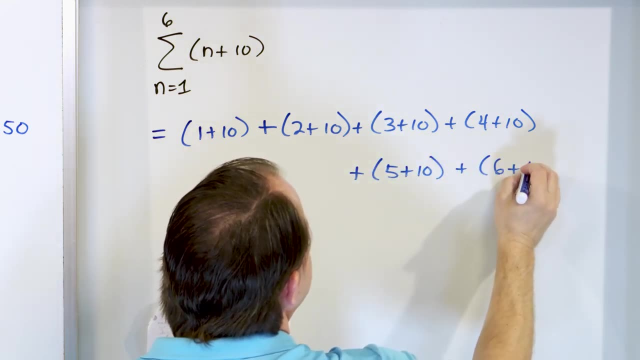 be 3 plus 10.. Then it'll be 4 plus 10.. I'll go down here. Then it'll be 5 plus 10.. Then it'll be 6 plus 10, because then, finally, n has gotten to its maximum value of 6.. 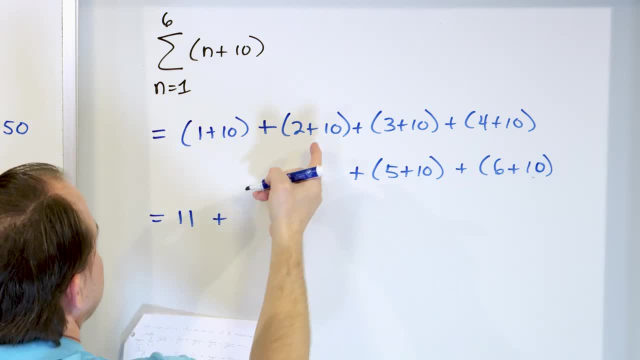 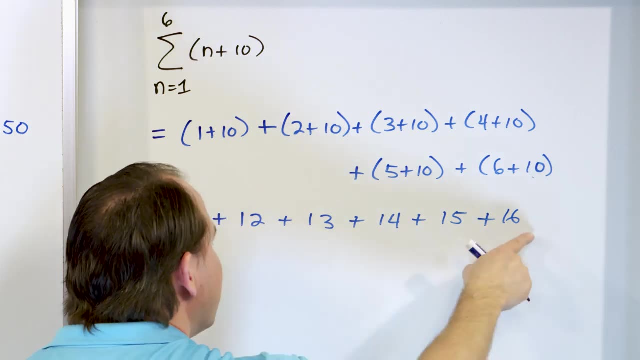 Now in the next step. then you go and add. You say this is 11,, this is 12,, 13,, 14,, 15,, 16.. Now I know that you can all grab a calculator and add these up. I don't want you to do that. 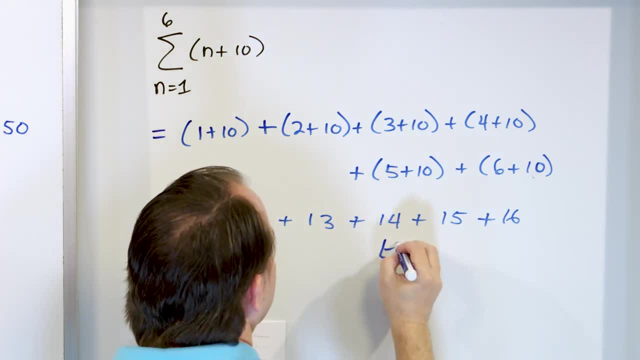 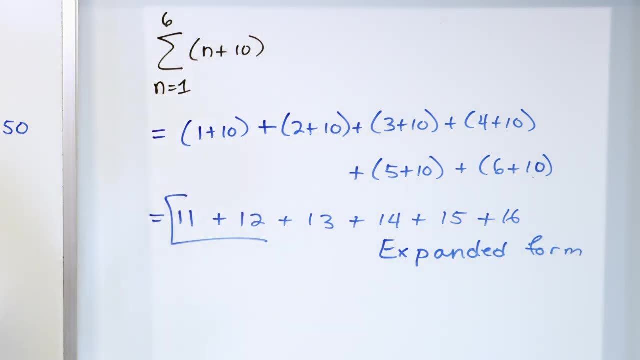 What I want you to do is circle this, because this is what we call expanded form. All I care about is that you can translate what the summation is telling you, the sigma, and write down the sum. That's all I care about. I know that you can all grab the calculator and add those together. 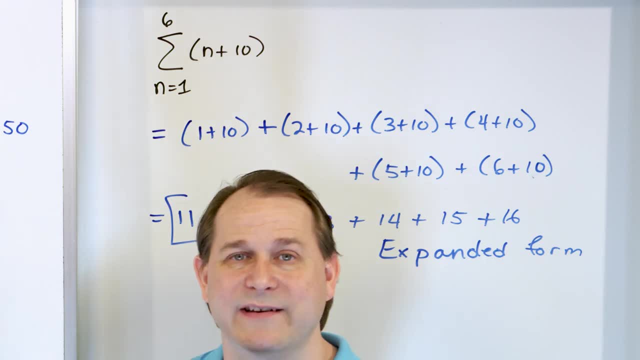 That isn't helpful to me. What I want to know is if you can take the sum, the summation, the sigma and blow out the terms. Later on in a few lessons, we'll talk about how to add these things together. I mean, obviously you can add these, but what happens if there's a thousand? 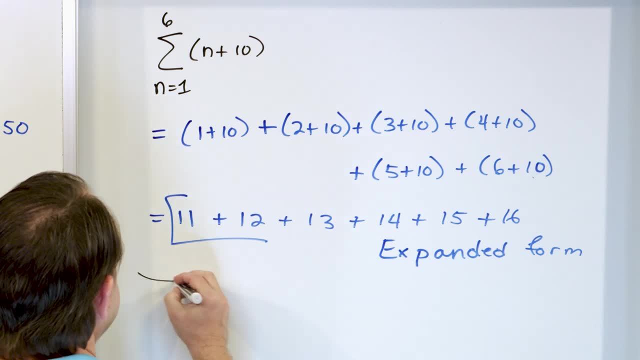 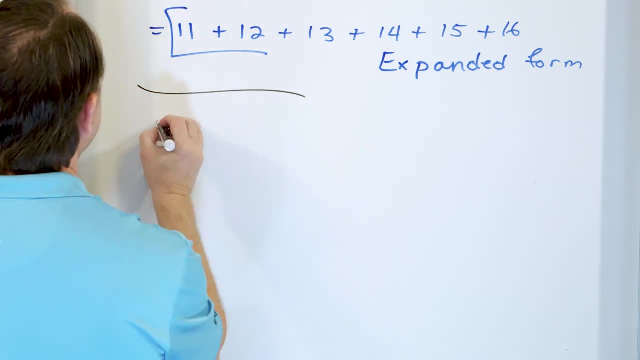 terms. How do I add them up without spending my whole life doing it? All right, So that's writing in expanded form. We're going to do one more like that and we'll call it a day and wrap up this lesson. What if I have the summation? n is 1 up to 6 and 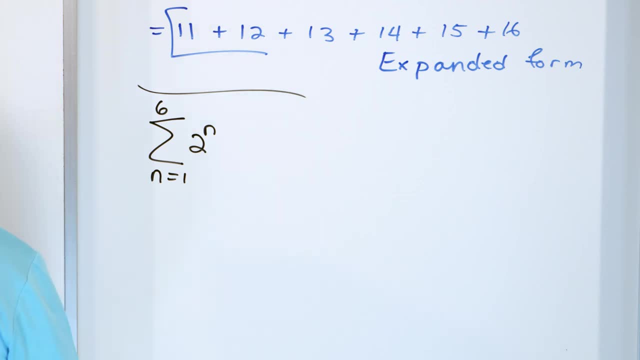 the sum and is 2 to the power of n. Okay, So what you do here is you say n is 1 plus 1.. So 2 to the power of 1., Then n goes to 2.. 2 to the power of 2.. Then n goes to 3.. 2 to the power. 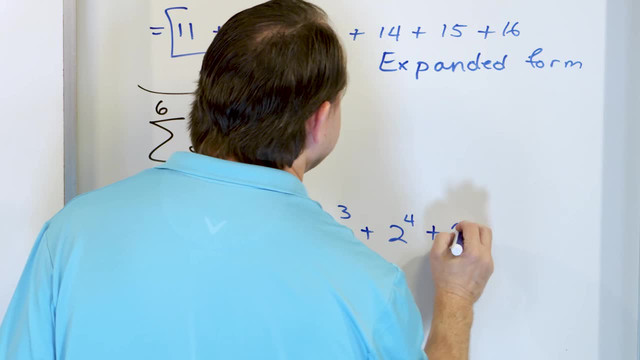 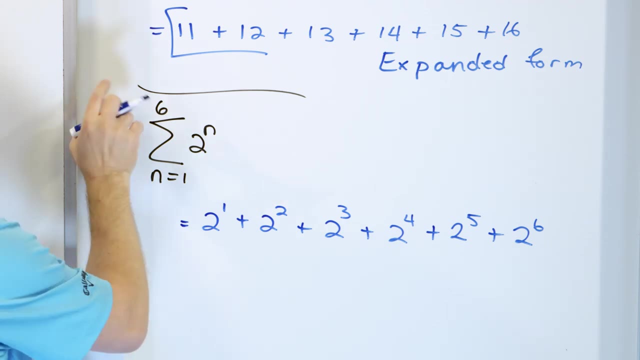 of 3.. And you see the pattern here: 2 to the power of 4.. 2 to the power of 5., 2 to the power of 6.. I stop at 6 because n has finally reached its maximum number, which is 6.. And I stop If there. 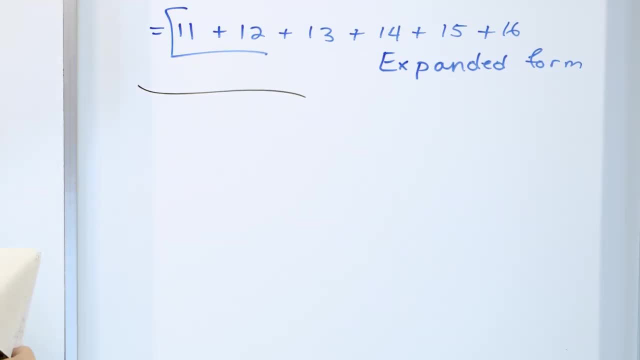 So that's writing in expanded form. We're going to do one more like that and we'll call it a day and wrap up this lesson. What if I have the summation, n is 1 up to 6, and the sum and is 2 to the power of n. 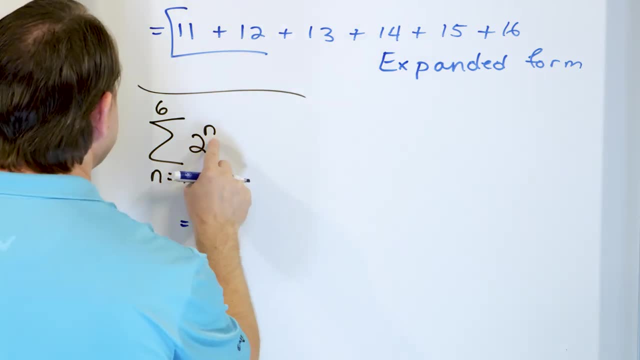 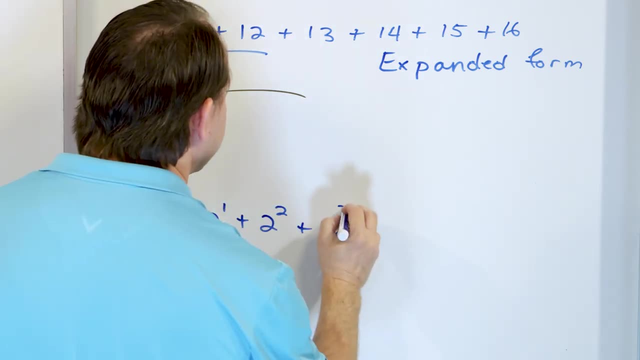 So what you do here is you say n is 1,, so 2 to the power of 1.. Then n goes to 2,, 2 to the power of 2.. Then n goes to 3,, 2 to the power of 3.. 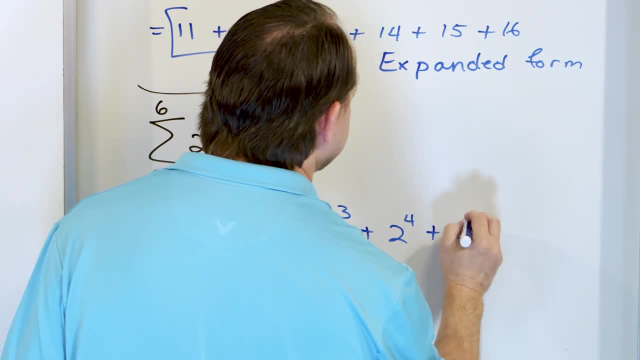 And you see the pattern here: 2 to the power of 4.. 2 to the power of 5,, 2 to the power of 6.. I stop at 6 because n has finally reached its maximum number, which is 6.. 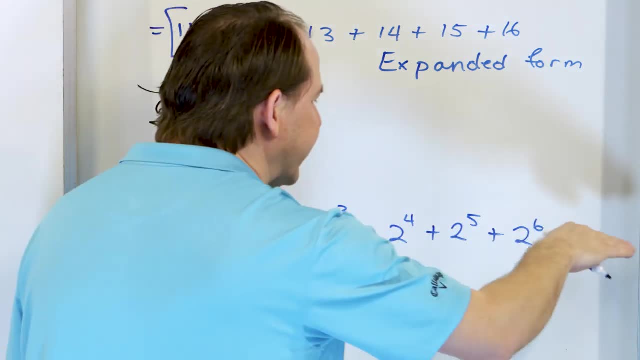 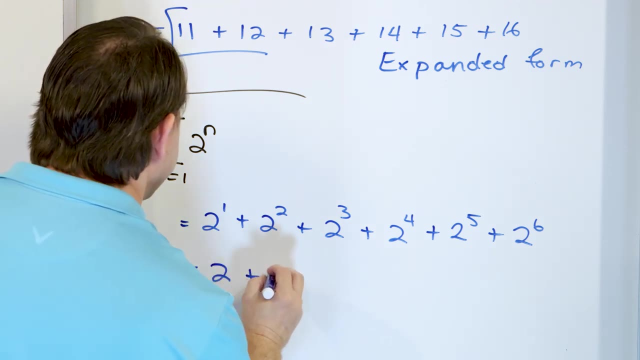 And I stop. If there was an infinity here then I would just put dot, dot, dot and I would keep the terms, would go forever. but this is a finite series, And so then you all know that this is 2,, this is 4,. 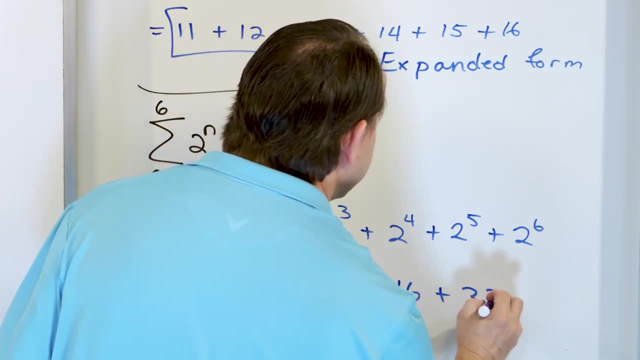 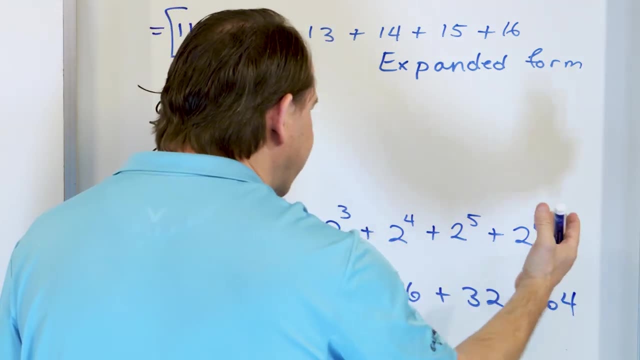 this is 8,, this is 16,, this is 32, and this is 64.. Might need a calculator to figure these last terms out, but you can see. what's happening is it's doubling, Doubling and then doubling again. 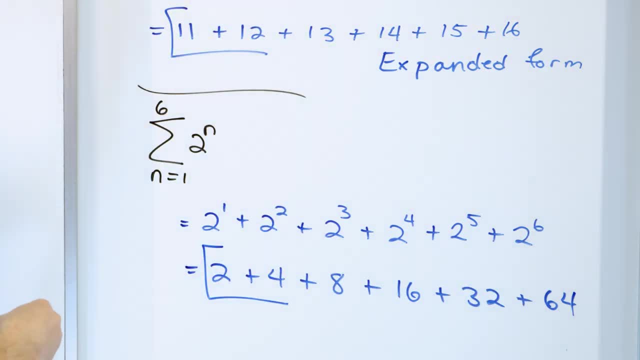 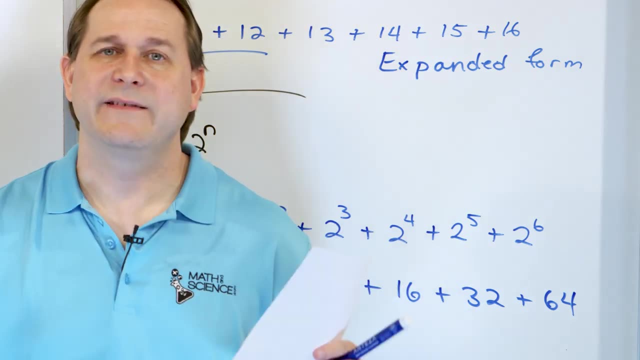 This is what we call expanded form. That's what I want you to write down. So in this lesson we have learned a tremendous amount of material. It's probably one of the more important lessons in recent times because it has such far-reaching implications. 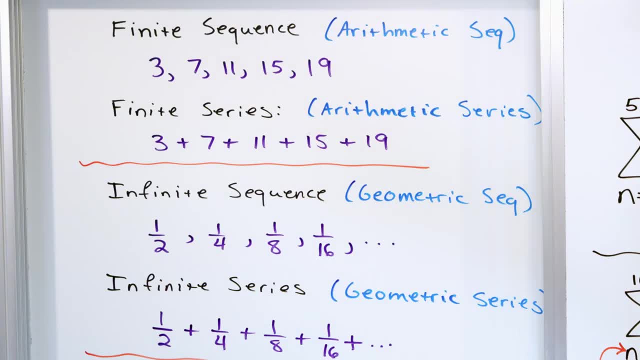 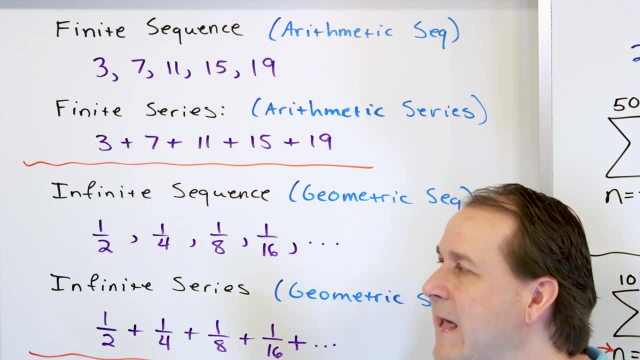 to calculus and other advanced math beyond that. We started out by saying that we have the concept of a sequence. It's just a listing of numbers. When you add up the terms of the sequence, we call it a series. It's a finite series when it has a limited finite number. 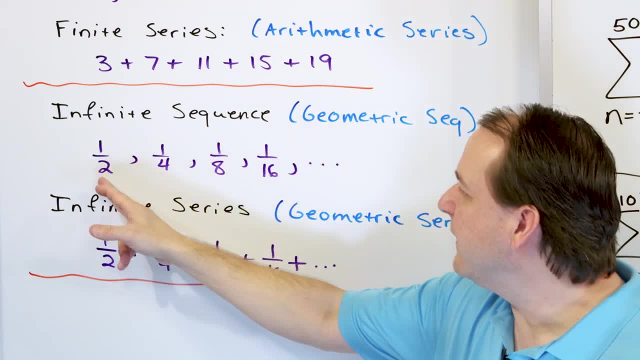 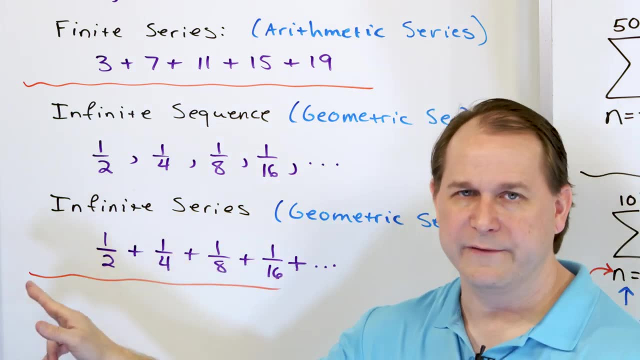 of terms. And then we said we can have an infinite sequence where the terms of the sequence just keep going and going and following the same pattern, forever separated by commas. If we add up those terms of the infinite sequence, we arrive at what we call an infinite series. 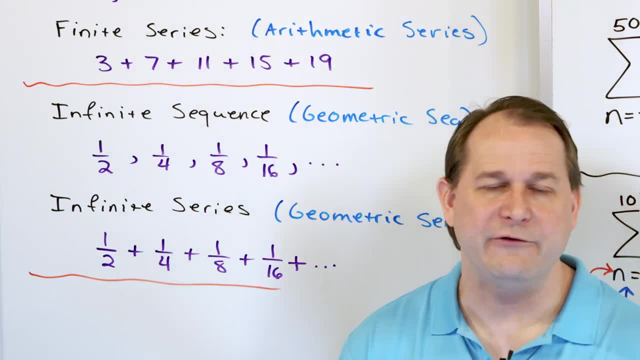 Now, because the terms of the sequence can be arithmetic or geometric, then we also have, instead of just arithmetic sequence and geometric sequence, we also now have arithmetic series and geometric series. There are other kinds of series in math that you'll learn in more advanced classes. 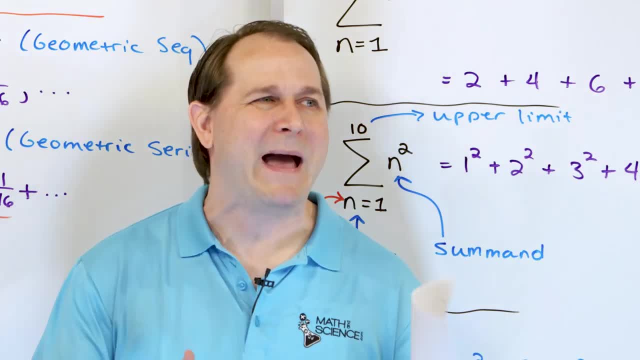 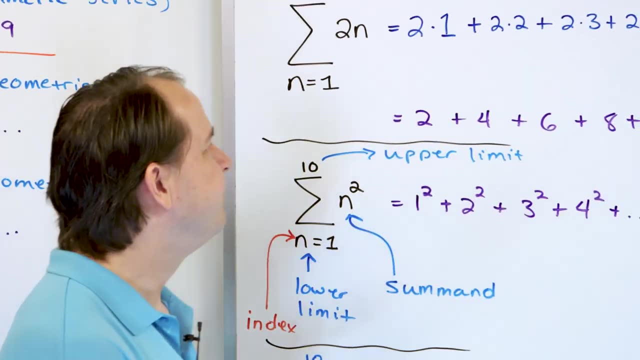 It's not limited to just these. There's tons of other kinds of series. There's power series, There's all kinds of things. I don't want to get into them, But there are other series that have other names that we'll learn down the road. 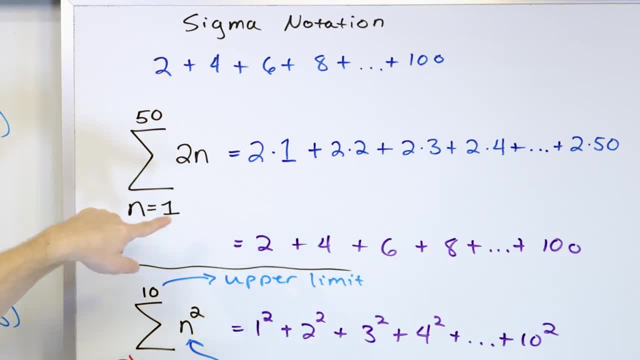 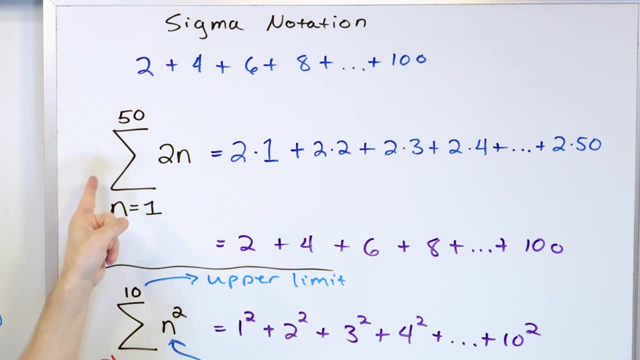 Then we talked about the summation notation. It's basically a loop that you just crank through, calculating the answers through the sum and, And you just follow the limits of summation here And basically that's it. You just crank through it. 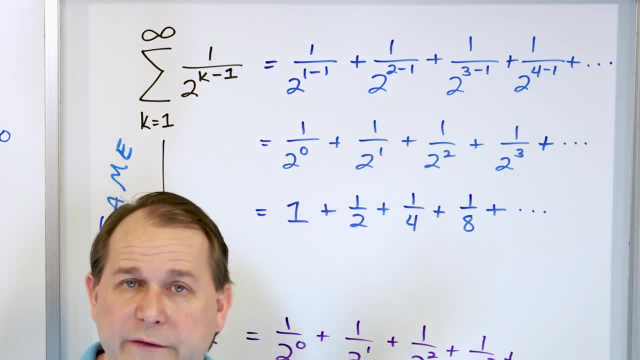 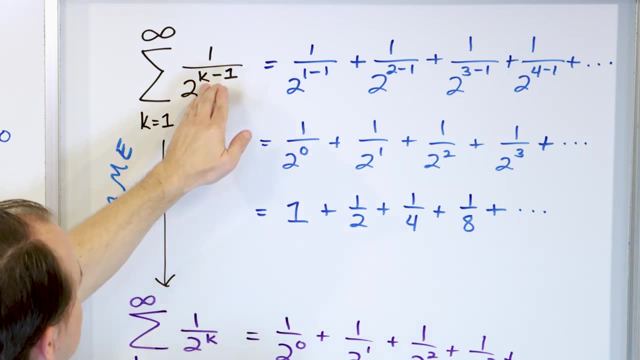 And then we have the idea that you can represent an infinite series, also with the summation notation, where infinity becomes the infinite series. That's the upper limit. Importantly, we also said that if you change, add or subtract numbers to the index in here you 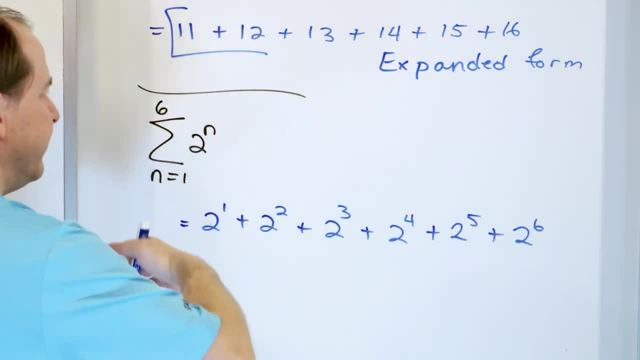 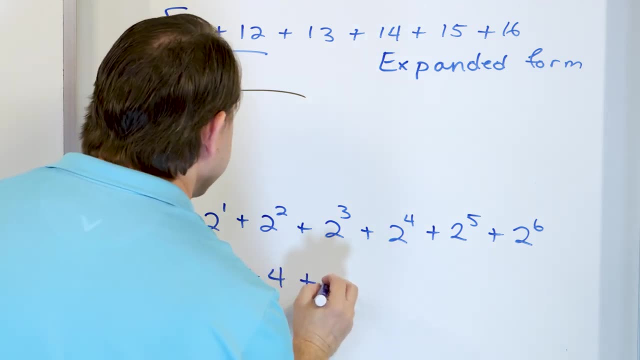 was an infinity here, then I would just put dot, dot, dot and I would keep the terms, would go forever. But this is a finite series, All right. And so then you all know that this is 2.. This is 4.. This is 5.. This is 6.. This is 7.. This is 8.. This is 9.. This is 10.. This is 11.. This is 12.. This is. 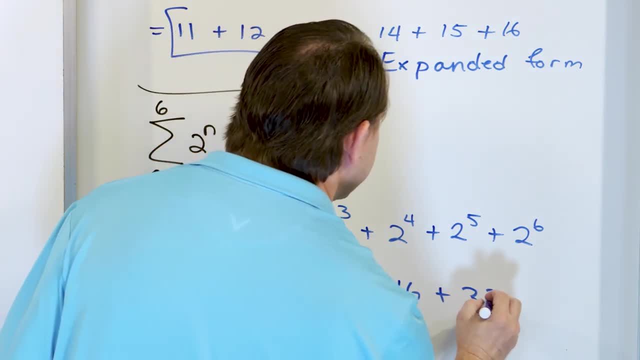 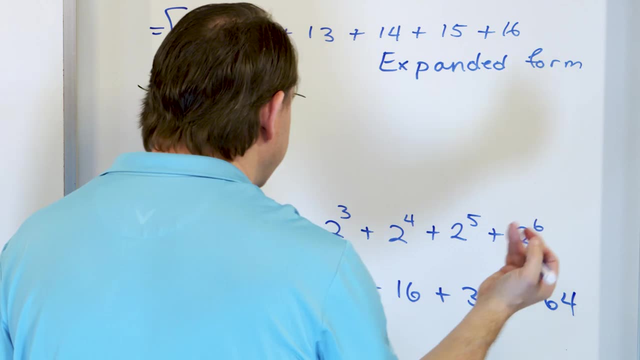 8. This is 16.. This is 32.. And this is 64. Now you need a calculator to figure these last terms out, But you can see what's happening is it's doubling, doubling and then doubling again. 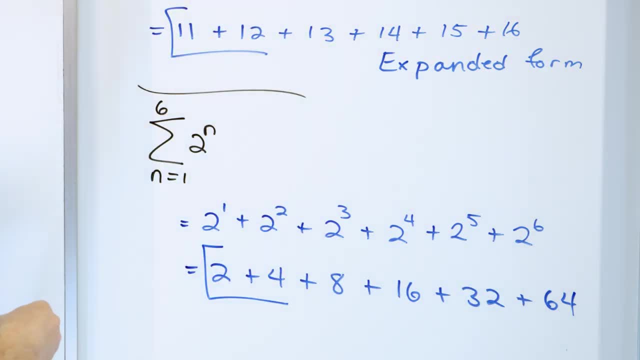 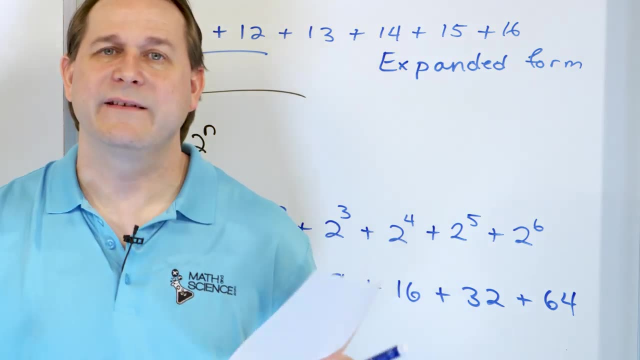 This is what we call expanded form. That's what I want you to write down, All right? So in this lesson we have learned a tremendous amount of material. It's probably one of the more important lessons in recent times because it has such far-reaching implications to calculus. 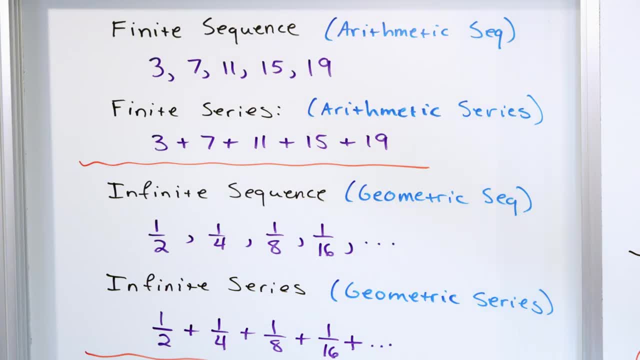 and other advanced math beyond that. We started out by saying that we have the concept of a series, We have the concept of a series, We have the concept of a series, We have the concept of a sequence. It's just a listing of numbers When you add up the terms of the sequence. 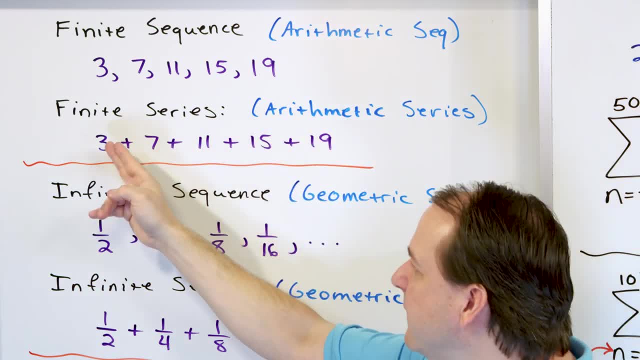 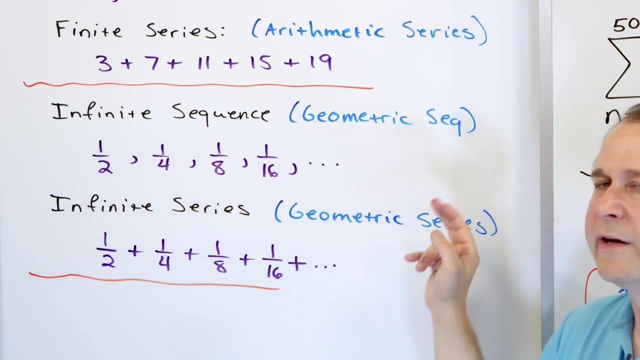 we call it a series. It's a finite series when it has a limited, finite number of terms. Right, And then we said we can have an infinite sequence where the terms of the sequence just keep going and going and following the same pattern, forever separated by commas, If we add up those terms. 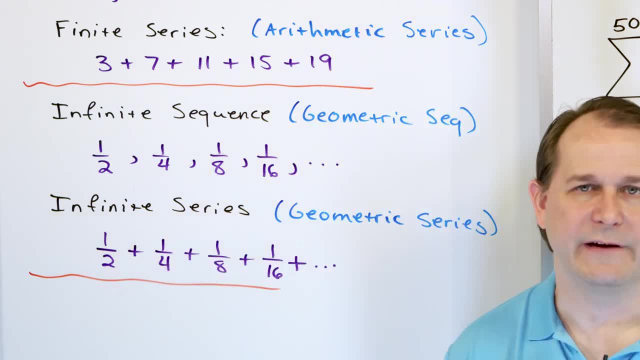 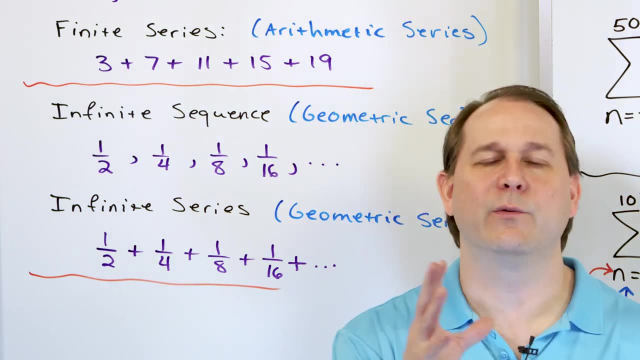 of the infinite sequence, we arrive at what we call an infinite series. Now, because the terms of the sequence can be arithmetic or geometric. then we also have, instead of just arithmetic, sequence and geometric: we have an infinite sequence And we have an infinite sequence. 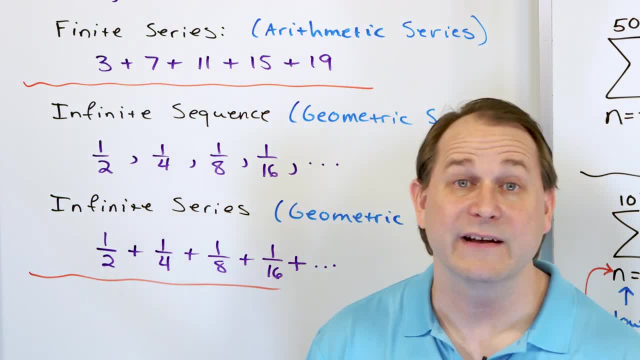 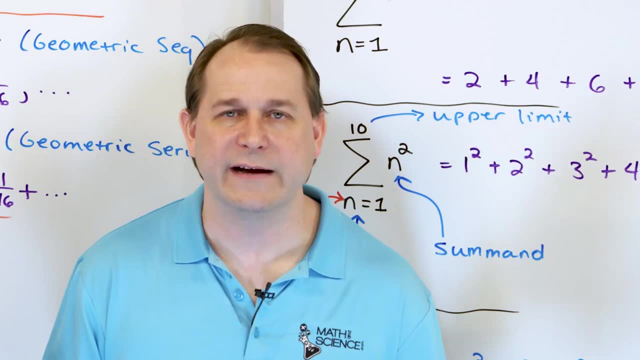 and geometric sequence. we also now have arithmetic series and geometric series. There are other kinds of series in math that you'll learn in more advanced classes. It's not limited to just these. There's tons of other kinds of series. There's power series, There's all kinds. 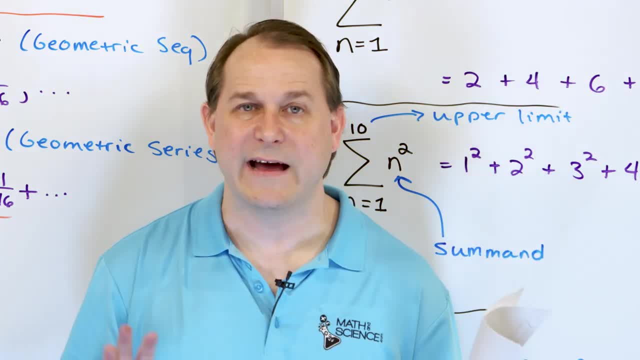 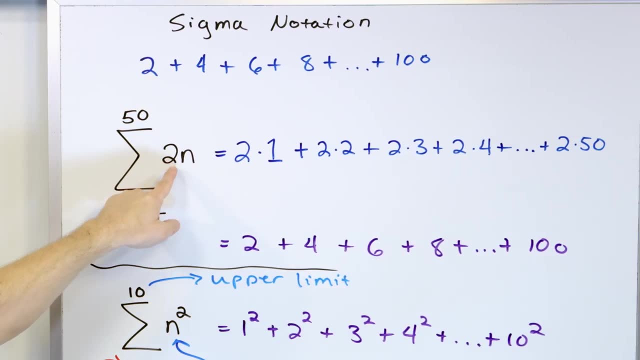 of things. I don't want to get into them, But there are other series that have other names that we'll learn down the road. Then we talked about the summation notation. It's basically a loop that you just crank through, calculating the answers through the sum, and, and you just 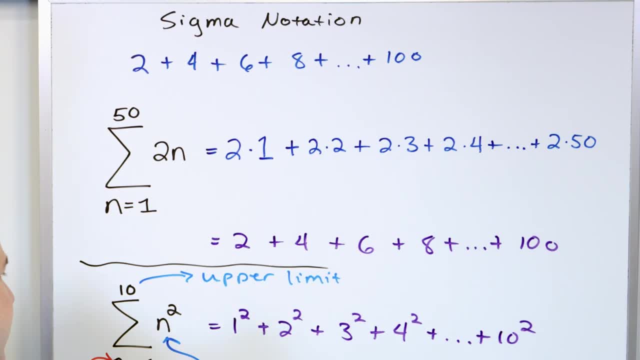 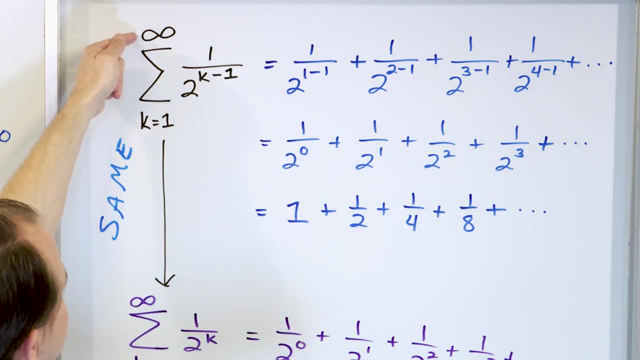 follow the limits of summation here And yeah, basically that's it. You just crank through it And then we have the idea that you can represent an infinite series, also with the summation notation, where infinity becomes the upper limit. Importantly, we also said that if you change, add or subtract numbers,